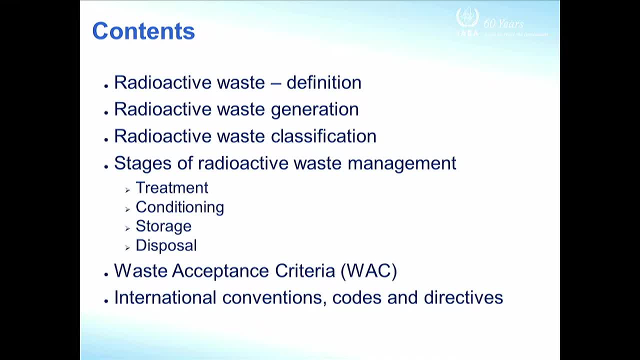 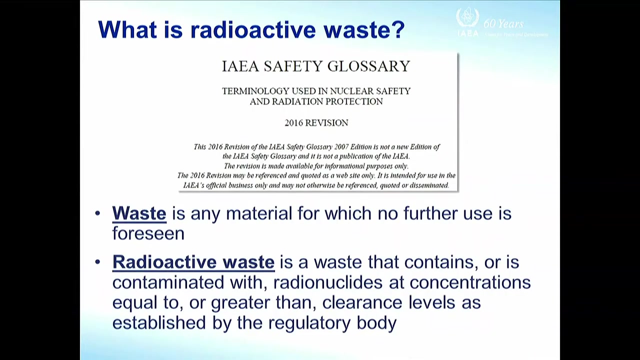 of the radioactive waste, the classification of the waste and the different stages during the process of managing the radioactive waste, The waste acceptance criteria, and I will mention some of the international conventions in place so far. So we have a glossary of safety terms. 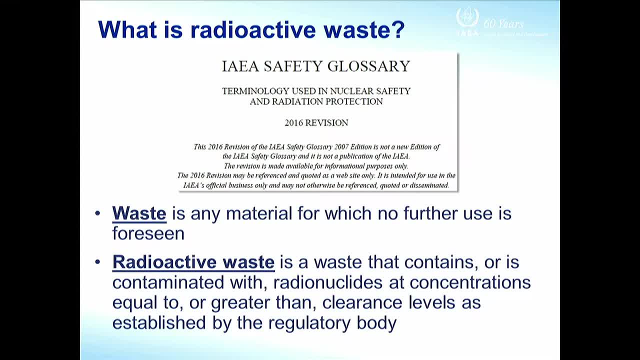 and terminology and in this glossary. you can find it in internet if you Google IAEA safety glossary and it was. oh, thank you. I think it's too late And it was issued in 2016,. it was the last revision. 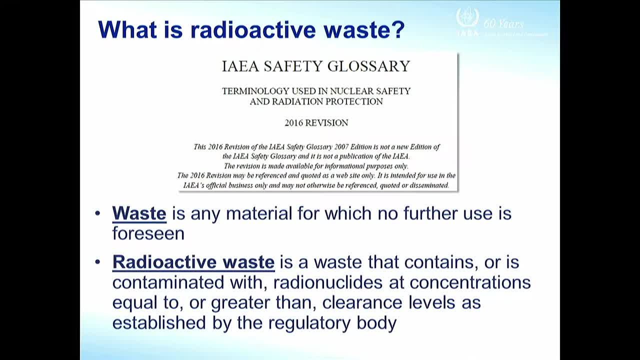 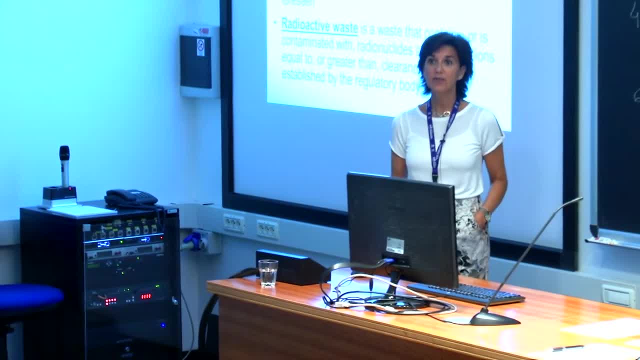 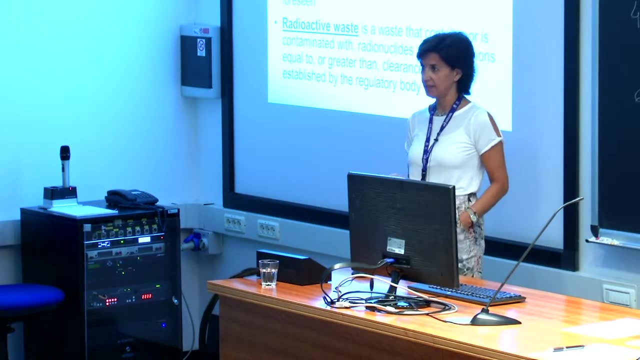 So there is mention that the waste is any material for which no further use is foreseen. So in the case of radioactive waste, it is a waste that contains or is contaminated because it's different. When it contains, it's because it's activated. 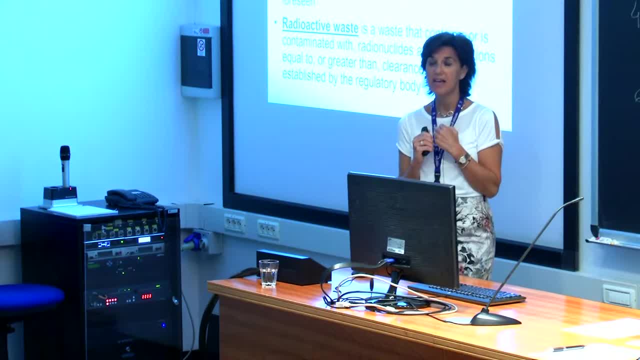 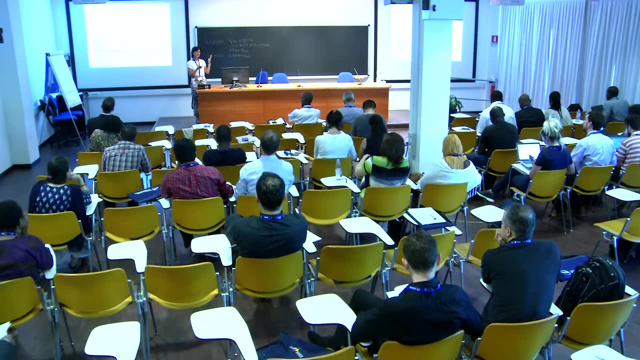 and the radioactivity is part of the material itself and when it's contaminated- sometimes the contamination can be avoided- We can clean the material. sometimes it's not that easy, but if it's contaminated we can decontaminate it. 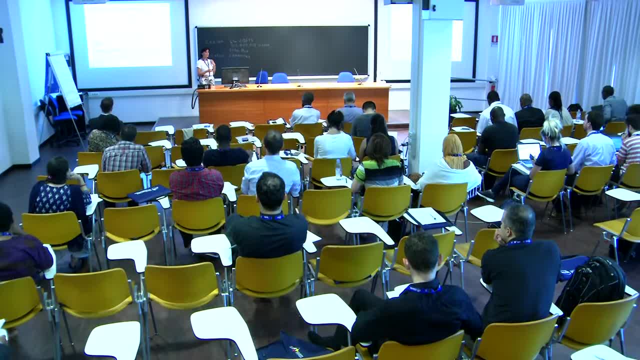 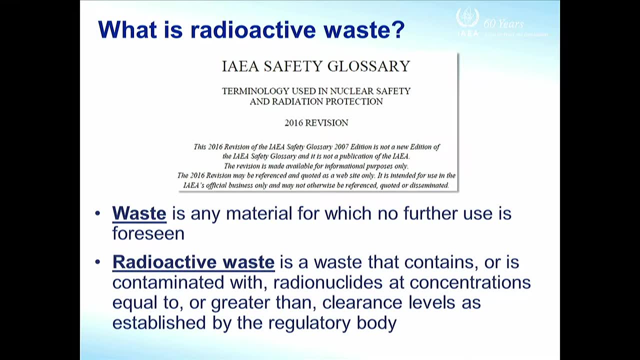 but if the radioactivity is part of the material, we cannot decontaminate it. So the radioactive waste is any material that contains or is contaminated with radionuclides at a certain level of concentration that is below the limit set by the regulatory body. 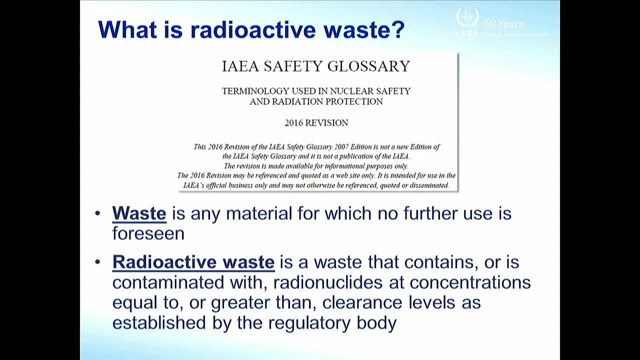 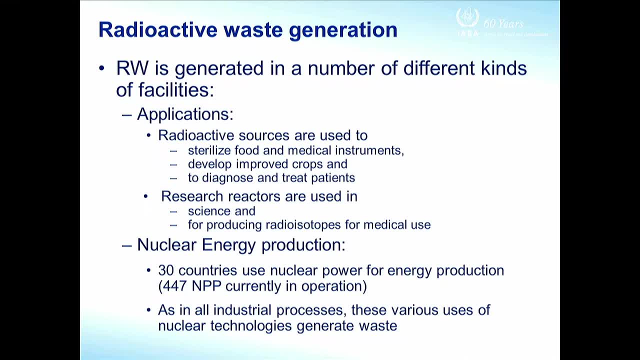 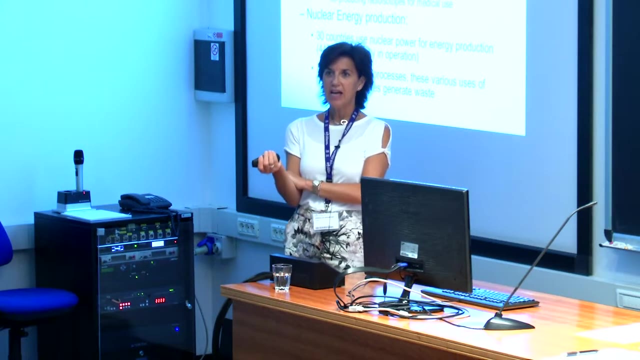 for which no other uses are foreseen. So there are many different type of facilities generating radioactive waste, and the waste are completely different, So it ranges from the radioisotopes used in medical treatments that are very short-lived and the concentrations are very small, only for treatments. 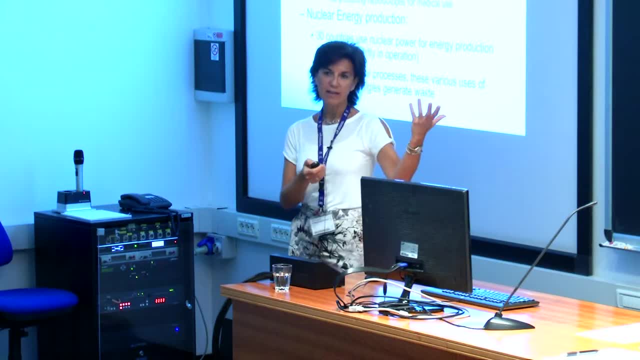 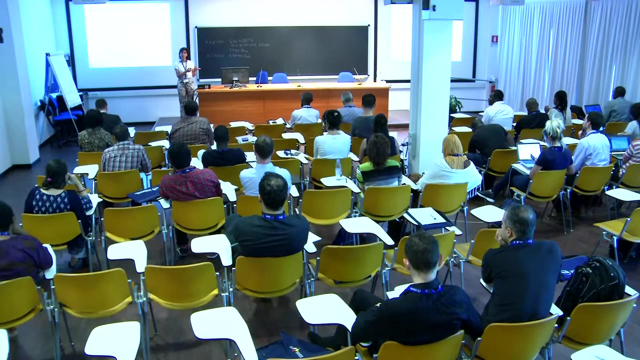 and it ranges from then to natural occurrence material, to the spent fuel. So the varieties and the forms are huge, And also the facilities. can be a small laboratory dedicated to research, produce or generate waste, and the main generator is the operation of the nuclear power plant. 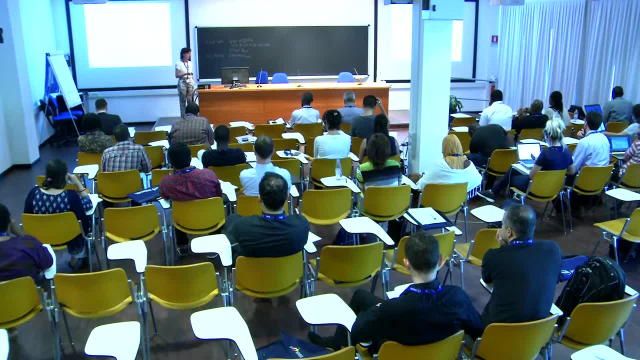 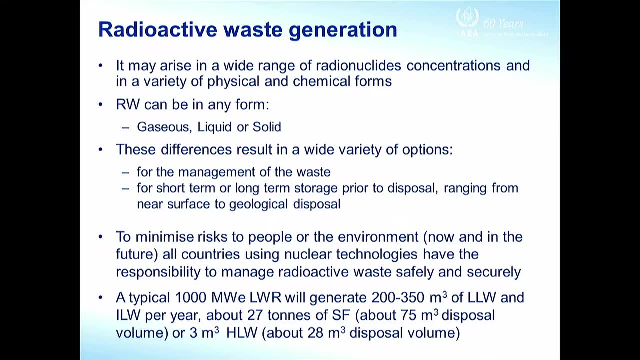 So the range of facilities producing waste is enormous. So for that the nature of the weights are very different and we can find radioactive waste with radionuclides in different concentrations and in physical and chemical forms. The radioactive waste can be gaseous, liquid and solids, and these differences result in 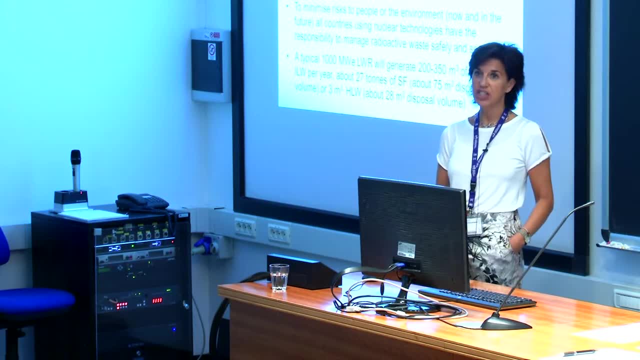 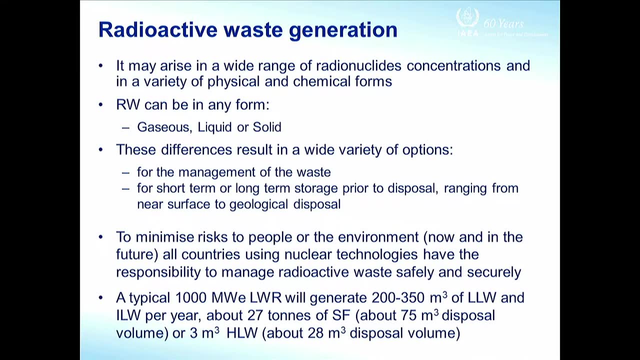 a wide variety of options for managing the radioactive waste. So the main, the overall objective in safety is the relative ways should be managed in the form that the risks to people and the environment are minimized, and it should be done in all countries using new methods. 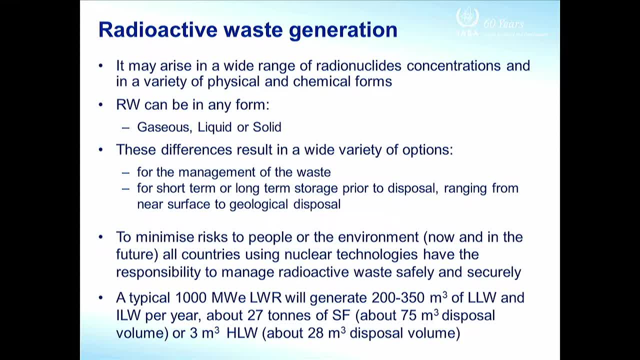 So, for example, to give you an idea of the quantity of radioactive waste produced by a nuclear power plant, around 1000 megaWatts generate around 200-350 cubic meters of low level waste and intermediate level waste in the operation of the nuclear power plant. 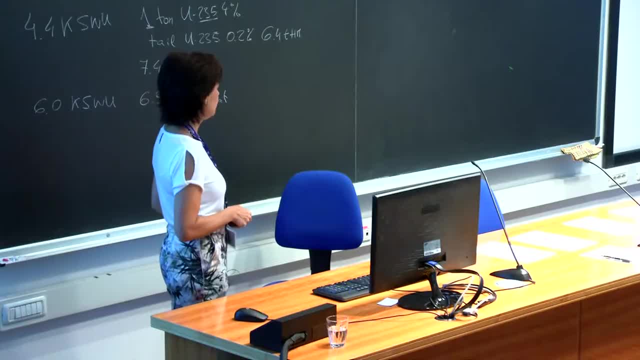 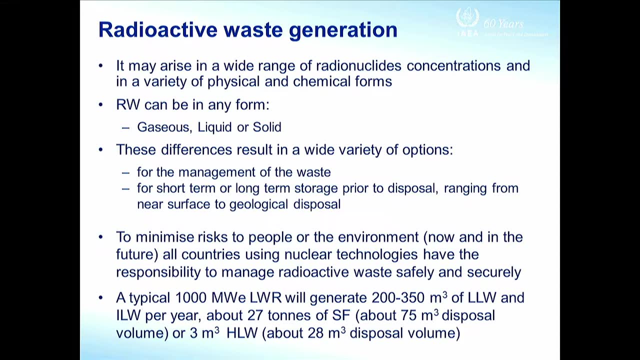 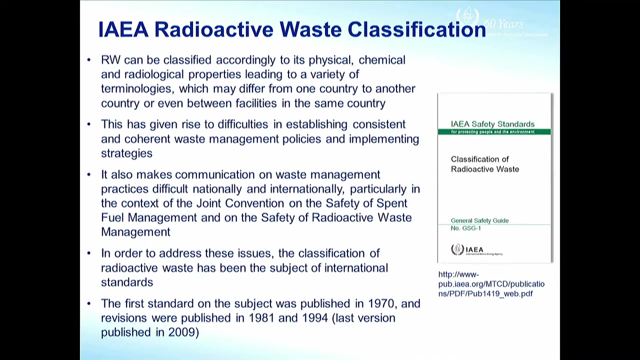 of the nuclear power plant and also generate about 27 tons of spent fuel. and if this spent fuel undergoes to reprocessing, it's generated around three cubic meters of high level waste per year. So, as we see, the radioactive waste are from different. 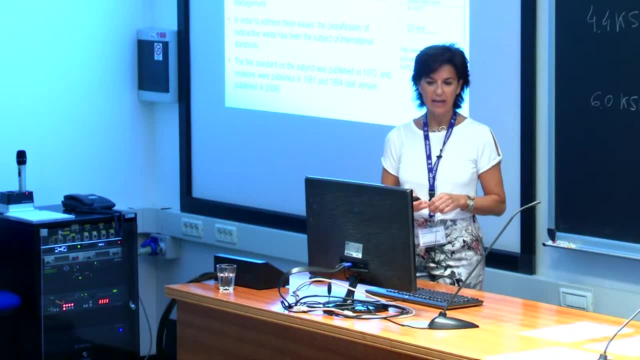 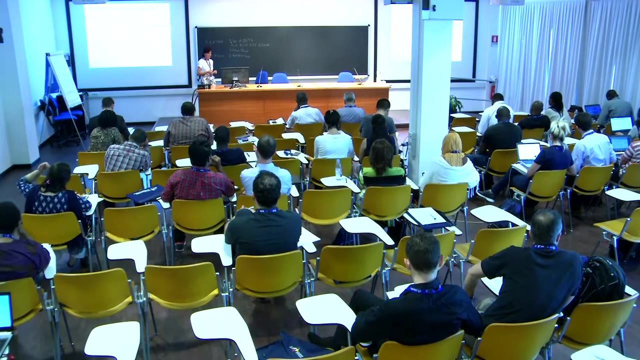 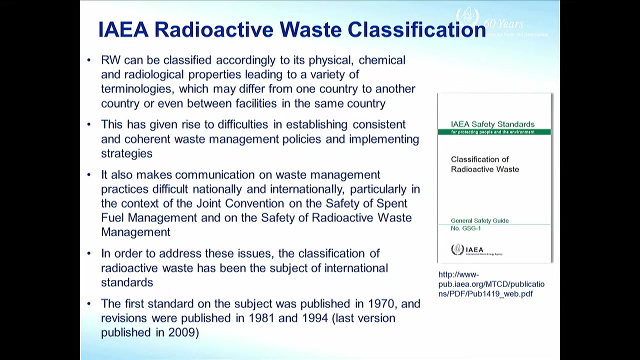 the different nature and from different generation. So it should be classified in order to harmonize, to compare from one facility to another facility in the same country and also between countries. So the radioactive waste can be classified according with their physical, chemical and radiological properties. 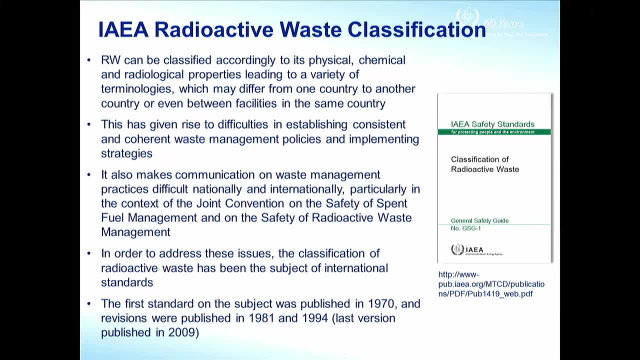 And due to the difficulties in comparison between facilities and between countries, it was decided to make guidelines for international classification. So this is the current classification in place so far, And the first one was issued in 1970 and it was revised in 1981 and 94.. 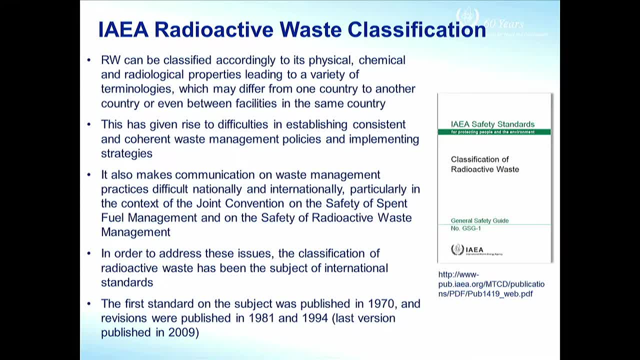 And the last one was published in 2009.. So the INC recommends countries to use this classification in order to harmonize and to be able to compare the radioactive waste produced in one country to another country, And it's very important that we will see. 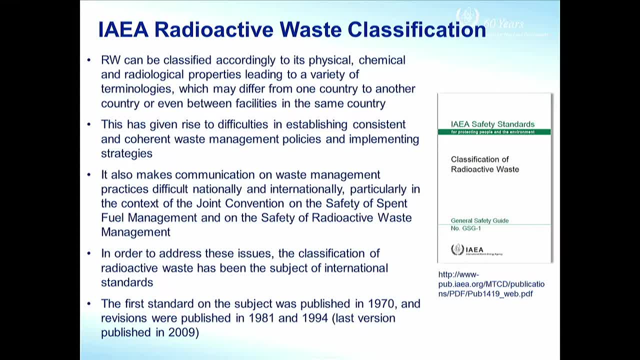 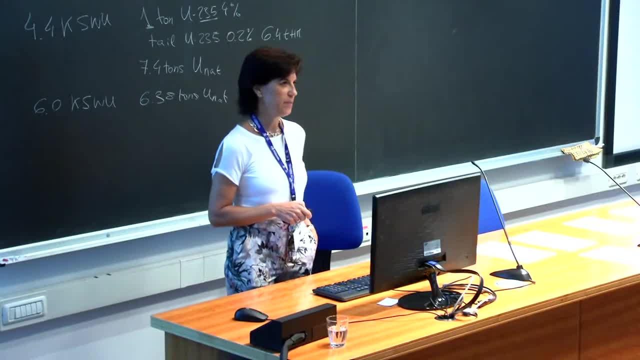 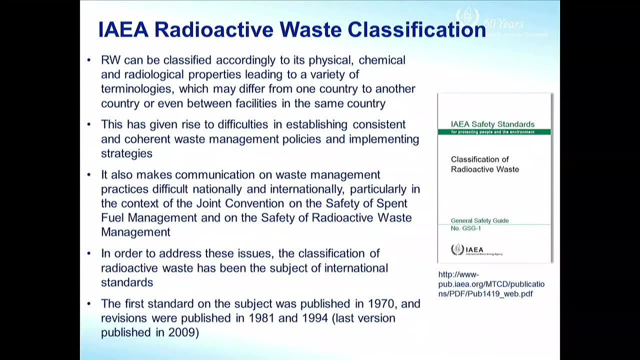 at the end of the presentation in terms of the joint convention on the safety of spent fuel and radioactive waste management. So the convention is a legal bonding convention and it's based on the peer review between among countries on what they are managing. 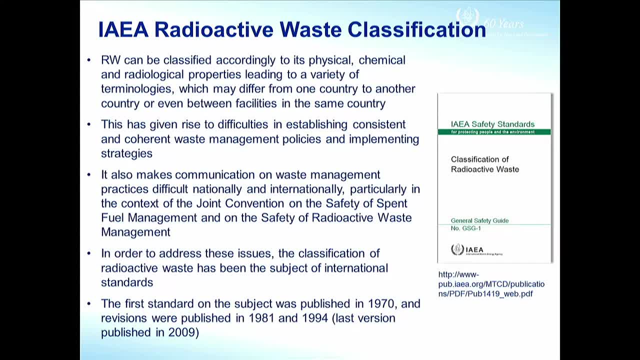 So the classification should be comparable, Otherwise we don't know if we are. when we are talking about intermediate level waste, what does it mean? Or low level waste, what does it mean in one country to another country? Should mean the same in all countries. 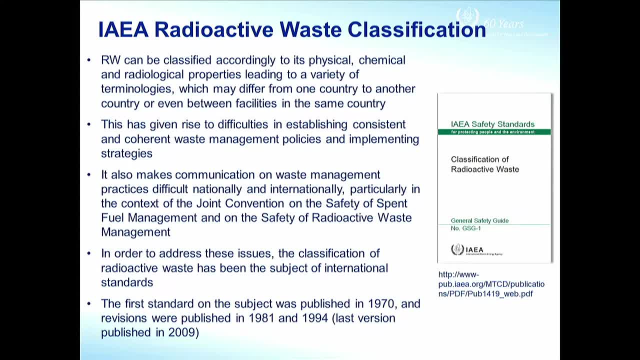 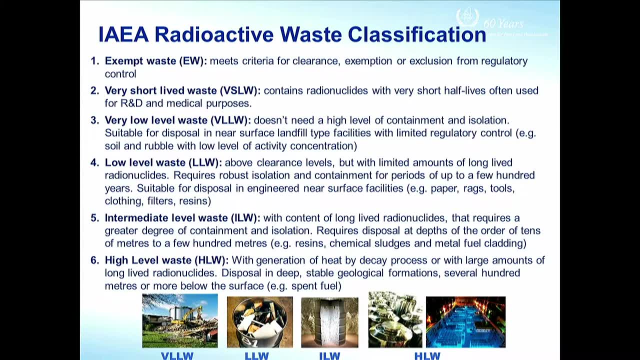 in order to compare and to be able to talk about it. So this is the current classification proposed by the agency and included in the document I mentioned before. So first of all, we have the exempt waste. What does it mean? Is the waste that the content? 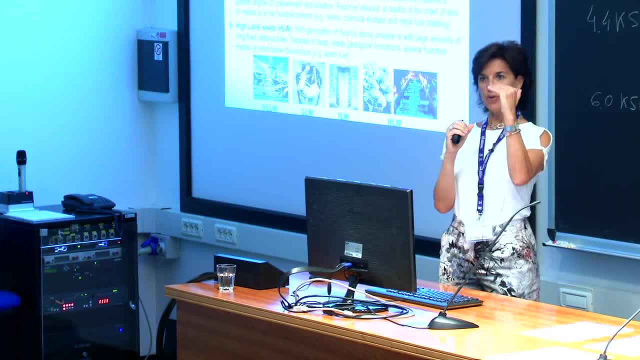 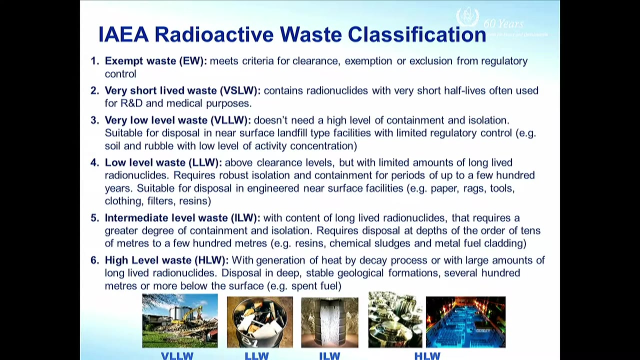 the radionuclide or the radioactivity content doesn't reach the level set by the regulatory body, So can be cleared or exempt to go under under regulation. The second category is the very, and this is very important in decommissioning, for example. 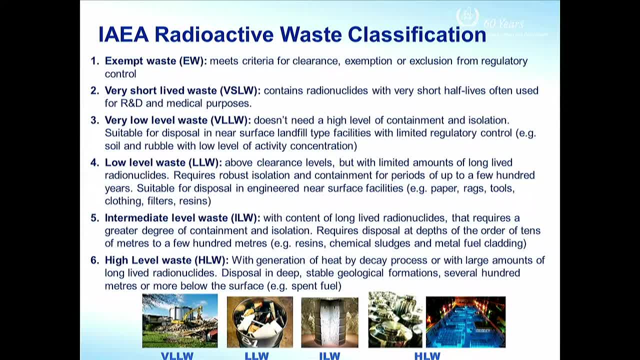 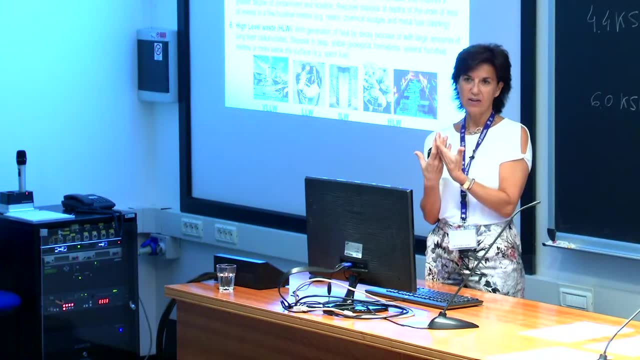 Because in the nuclear power plant, if we consider everything, because the nuclear power plant is a nuclear facility itself- if we consider everything under regulatory constraint, or there's a huge amount of waste and there are a lot of buildings that are not contaminated and never were exposed to. 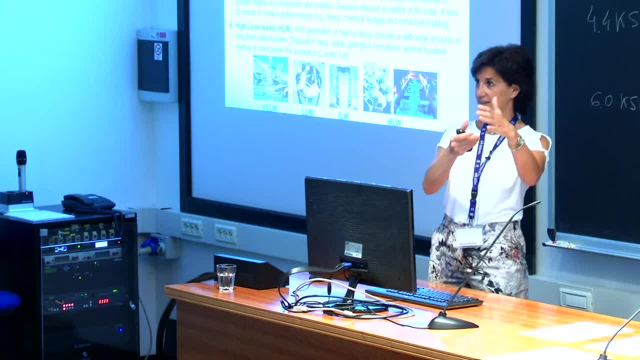 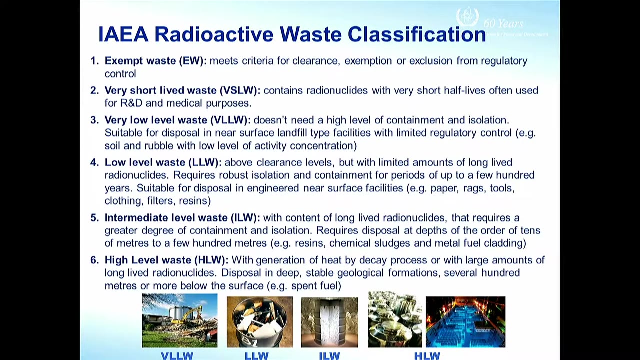 to contamination. so they can be cleared and they can be apart from the regulation. So they are measured and they are exempt waste. They are considered not contaminated and they are not undergoes to the managing of the radioactive waste material. So we have another. 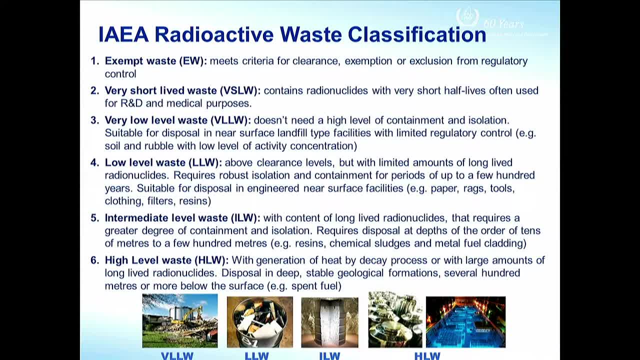 the second category is the very short lived waste, And it is mainly those material used for medical purposes, because the half life of the radioactive waste used are very, very short hours or days, but not longer than that. So these activity 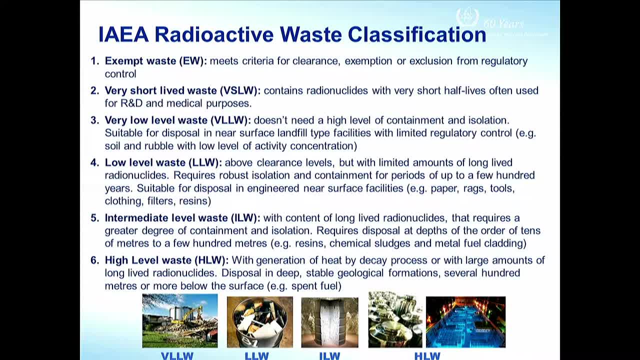 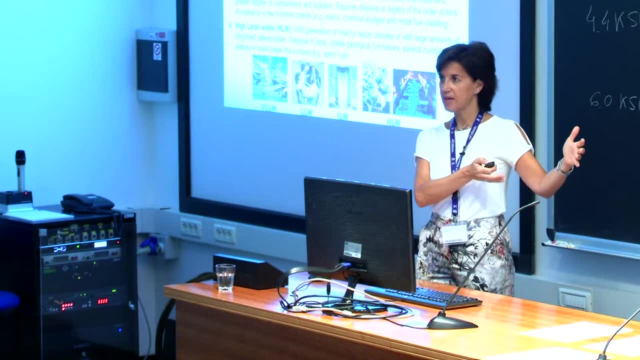 we can. these waste can be managed. only keep it in some store facilities, in the same, in the same, in the same facility of the producer and leave it them until decay. And when it decay they can be managed as conventional waste. And, for example, some medical waste produced by radiopharmac. radiopharmacs are more dangerous by the biological risks. For example, the needles are more risk by the biological risk than the radiological. So radiological if we can, if they leave the waste for months or years. 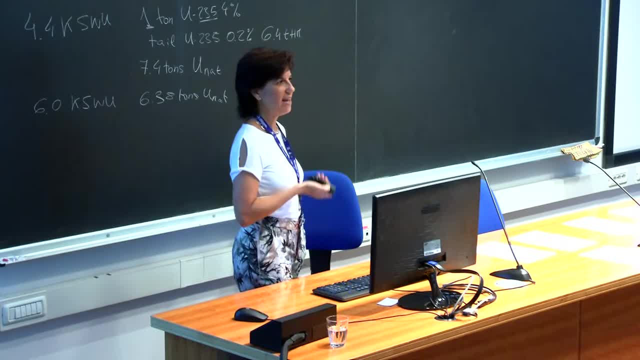 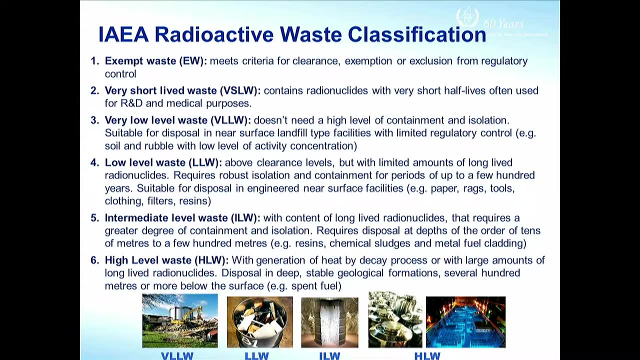 they are sure that the radioactivity has decayed under the limit and it's not longer at risk, And they are then treated as biological waste. So the third category is the very low level waste, And they don't need a high level of containment. 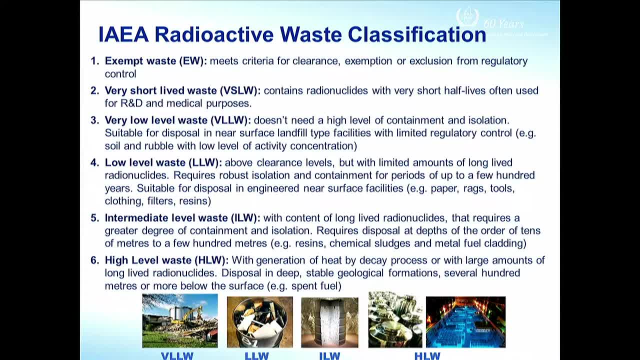 or isolation, and they can be. they can be disposed in the surface, in the repository surface, And we will see the different options. Then the fourth category is the low level waste, So they have levels above the clearance and they have limited amounts of longleaf radionuclides. 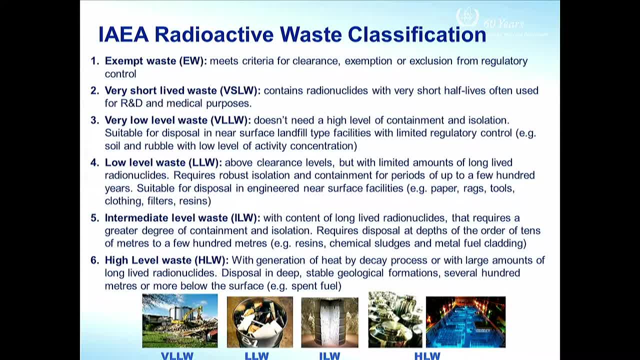 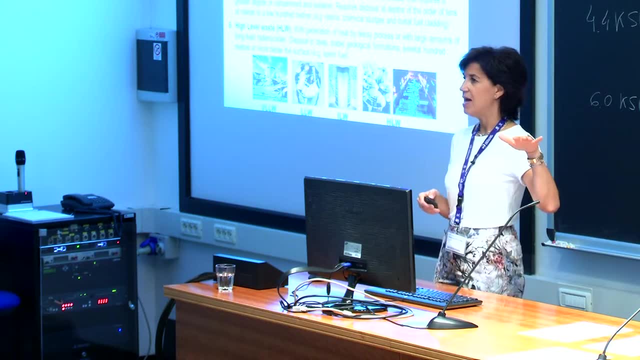 that usually are alpha emitters. So, for example, in the case of Spain, is the case of El Cabril- I don't know if you've heard about it, stuck about it- So if our repository in the south west of the country and is dedicated to low level and intermediate level waste, 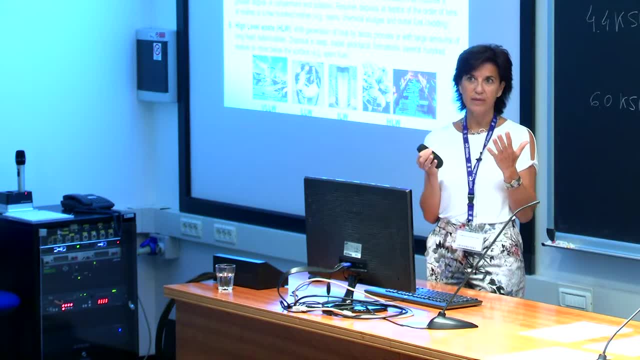 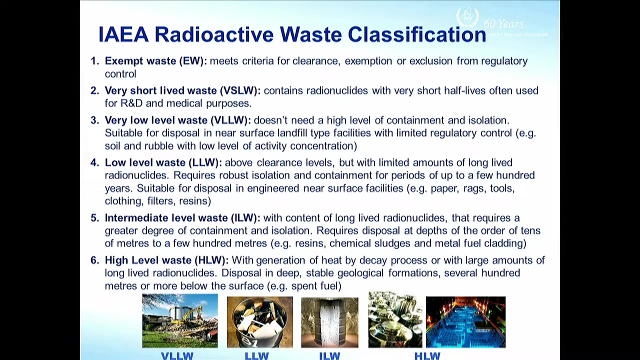 but they have a very strict. they are very stricted in the alpha emitters that can be disposed of there. So this is the limitation, because they consider them low level waste. And we have another category. The fifth category is the intermediate level waste. 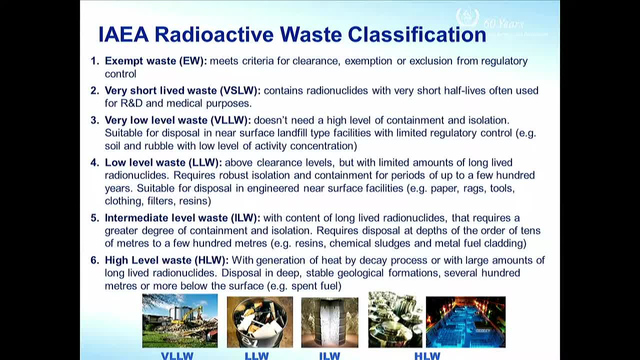 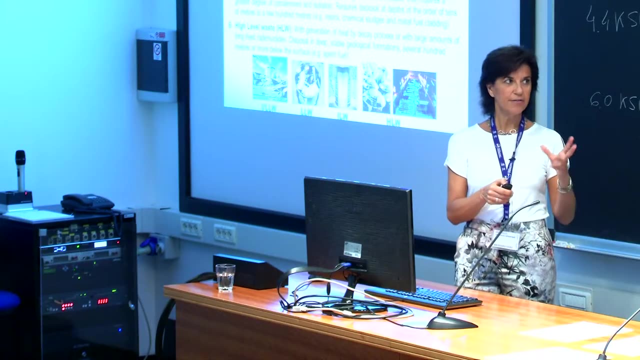 And so they have. they contain certain amount of longleaf radionuclides that can be beta gamma emitters and alpha emitters. They require greater degree of containment and isolation and they are disposed underground, a few meters underground. And the sixth category: 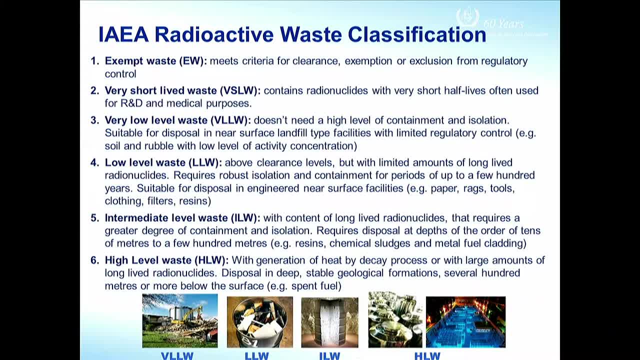 is the high level waste that consists in the spent fuel itself when it's considered as a waste in the open cycle option, or the high level waste produced after reprocessing of the spent field after the PUREX process, And it's mainly formed by fission products. 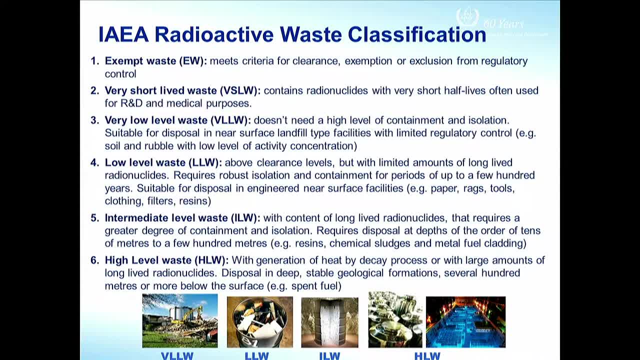 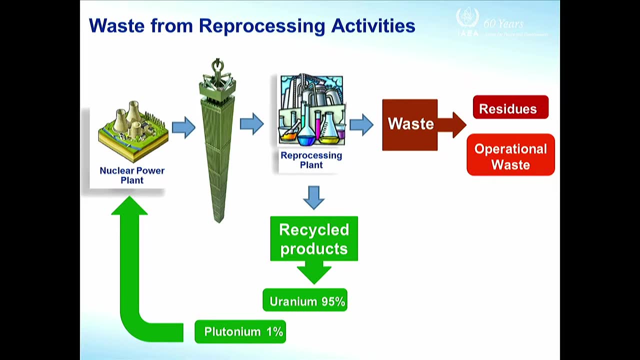 and myelactinides And they are vitified in glasses matrix condition in glasses matrix And disposed in deep geological repository as a spent fuel. So, for example, to give an example of an activity that generate low level, intermediate level and high level waste. 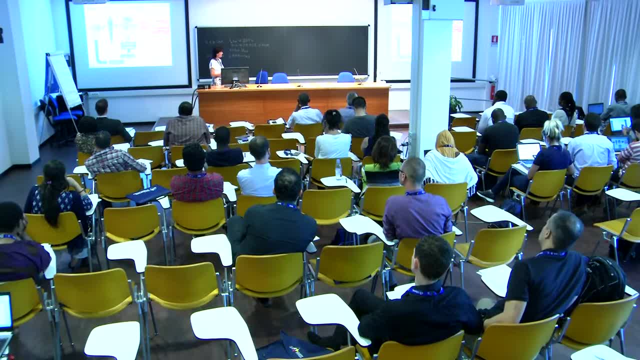 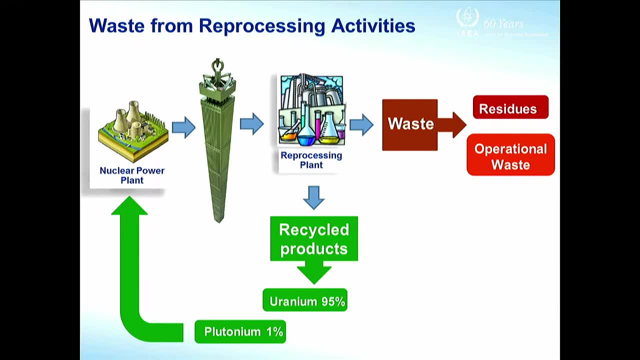 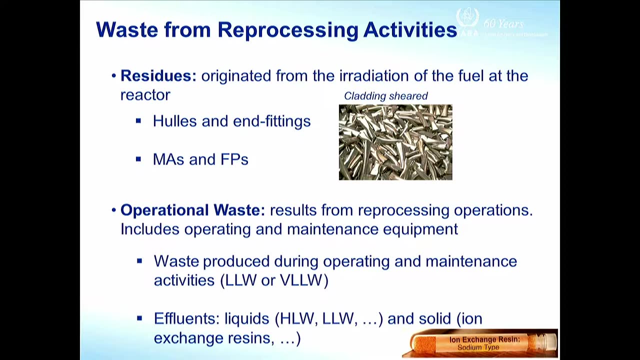 is the reprocessing activities. So once uranium and plutonium is reprocessed and recycled products, they generate a waste and the waste are the residues. So the residues are originated from the irradiation of the fuel at the reactor And they are the hues and the end fittings. 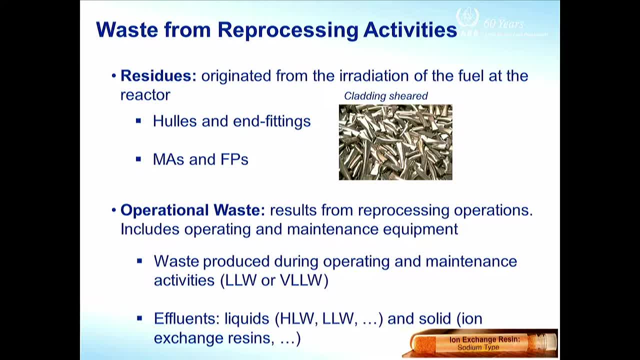 of the tubes, of the rods containing the fuel And also residues, are the minor actinides and the fissure products that form the high level waste stream that has to be vitified. So the hues and the end fittings are considered intermediate level waste and they are super compacted. 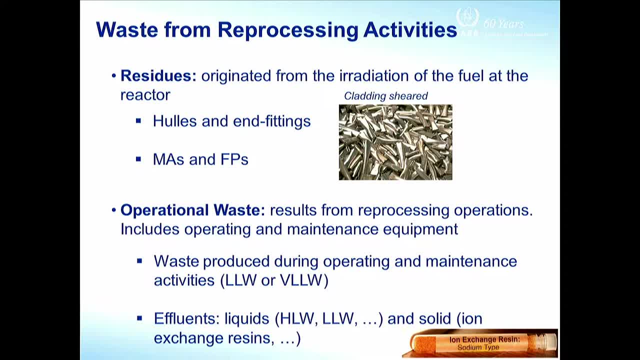 And we will see later. And the minor actinides and fissure products are liquid, high level liquid waste that has to be solidified, including in a condition in a matrix glass, And there are the so-called operational waste that are generated in the operation of the facility. 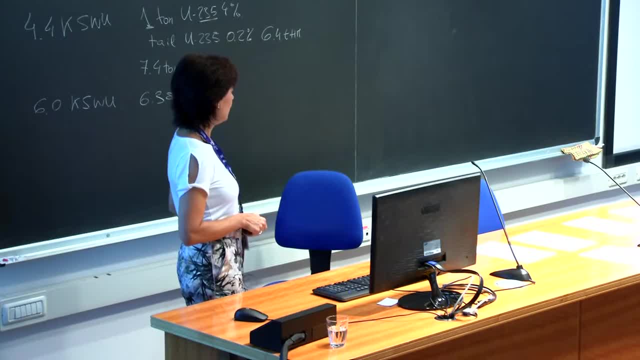 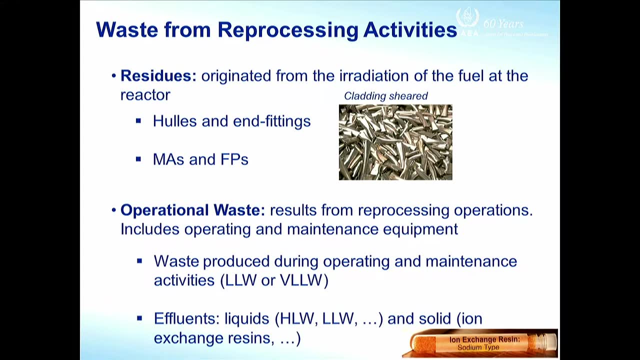 so they are low-level and very low-level waste, And also they are intermediate waste. High level is the minor actinides and fissure products, But there are, for example, some resins originated in the purification processes that have to be managed as radioactive waste. 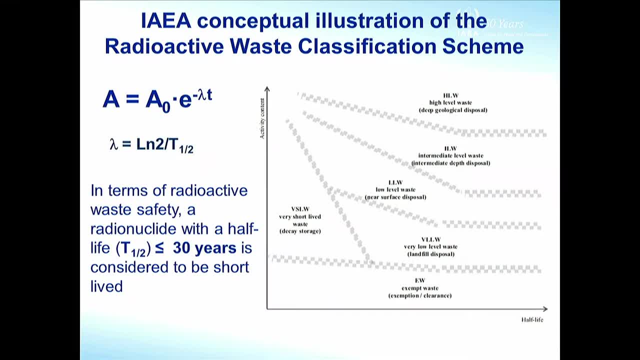 Okay, And I don't know if you can see properly. I think yeah. So this is the conceptual classification that you can find in the safety guide I mentioned, And so it gives an idea. This is the level of activity and this is the timeframe. 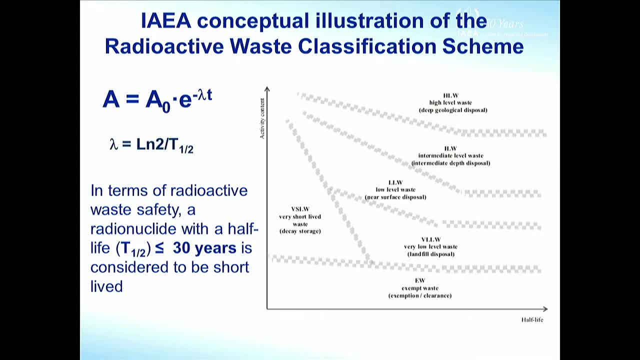 So you see, the six category are drawn in these drafts. So this is the exemption waste, This is the short-lived that decay very, very fast. This is the low-level waste, the intermediate waste and the high-level waste that needs a lot of time. 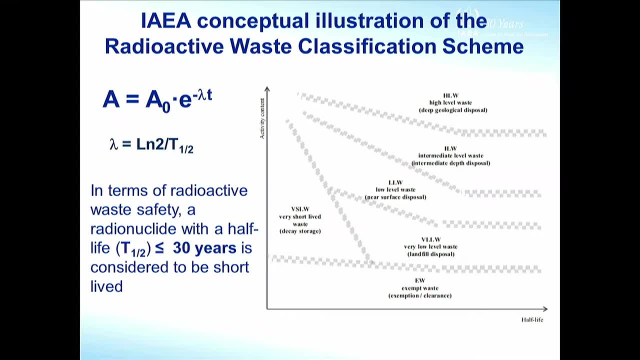 to reach the low level or the exemption level. And in terms of safety, aridonuclide with a high level half-life lower than 30 years is considered short-lived, So all radionuclides with half-life higher than 30 years. 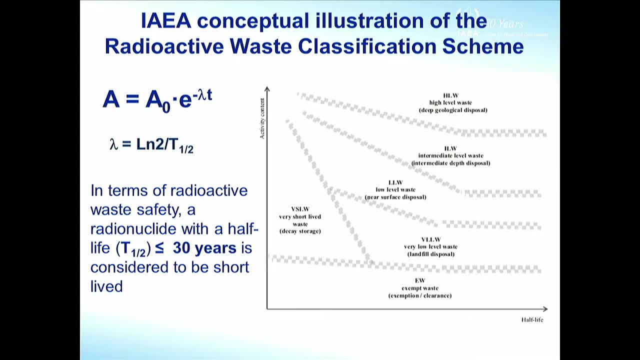 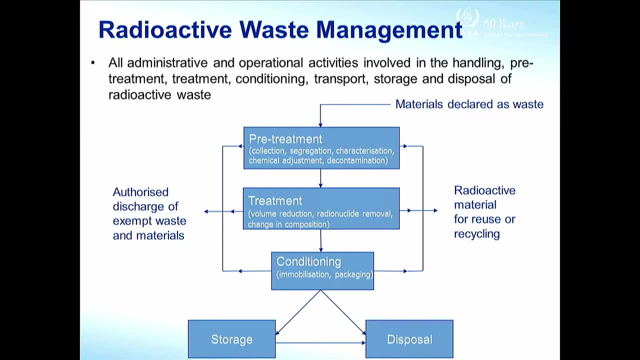 are considered long-lived radionuclides. So the different stages include in the management of the radioactive waste: are the basic steps are drawn in the picture and it consider in the pre-treatment treatment And then it's when the waste are segregated in those who can be considered not radioactive waste anymore. 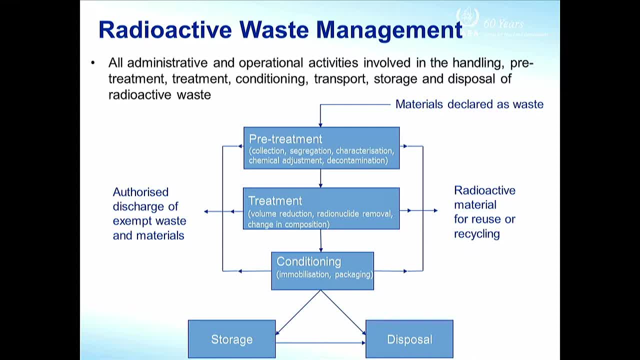 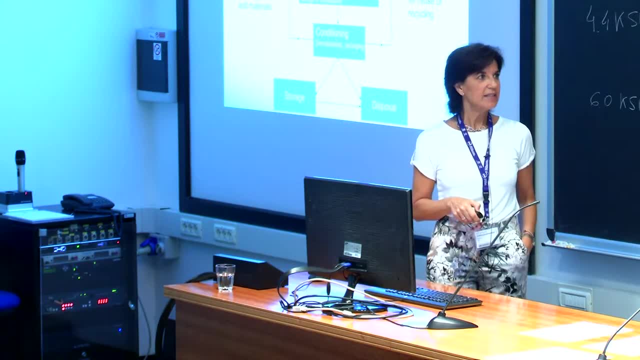 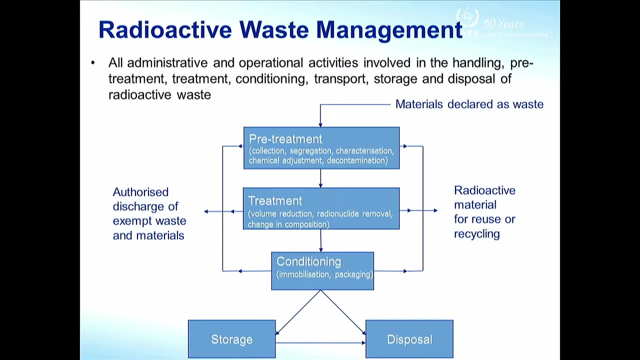 and conventional waste and those and the materials that can be recycling inside the nuclear cycle, And then, once the waste are treated, are conditioned to make them solid and difficult, the radioactivity to be leased and released, and then, after a period of a storage, they should be disposed of or directly. 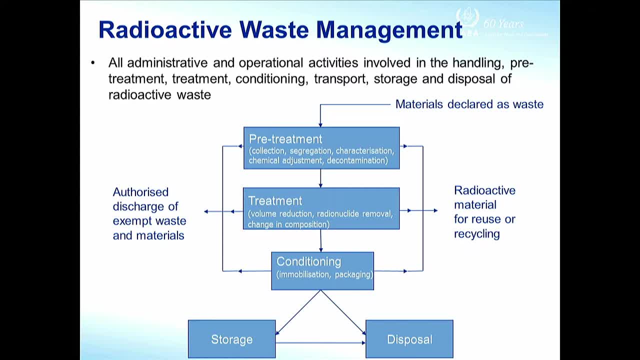 from conditioning. they can be disposed of. they don't need. sometimes they don't need to pass through the storage. this is a very generic draw. so this is in the case of high level ways of a spent fuel. but some of the low level ways or intermediate ways can be conditioned and then they early dispose of. 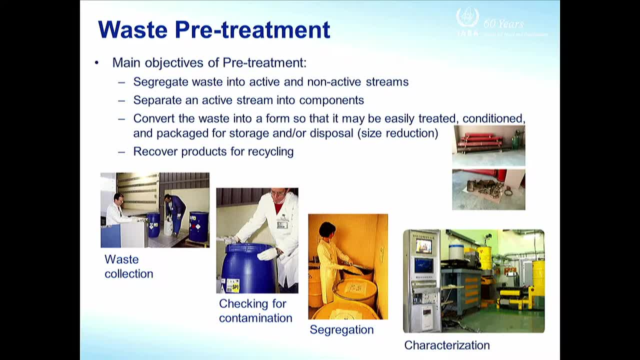 in the suitable facility. so let's talk about waste treatment. so the main objectives of these states in the management of the radioactive waste is to segregate the material into active and non active, so we can exempt some of the materials, and also to separate them in different stream components, and this 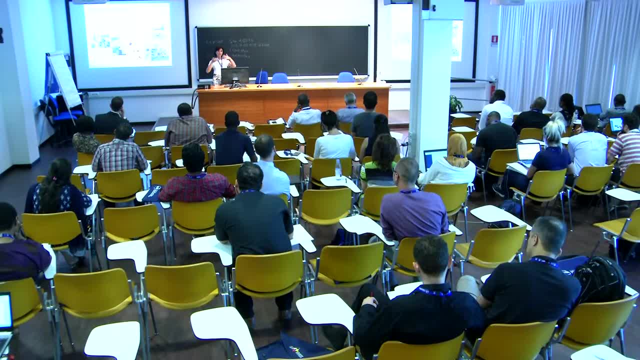 is very important because when the facility received the waste- or potentially for the next phase of the program, the waste is turned into a produce, the waste. they are of different level of contamination or different level of activity content, So sometimes we can produce cross-contamination. 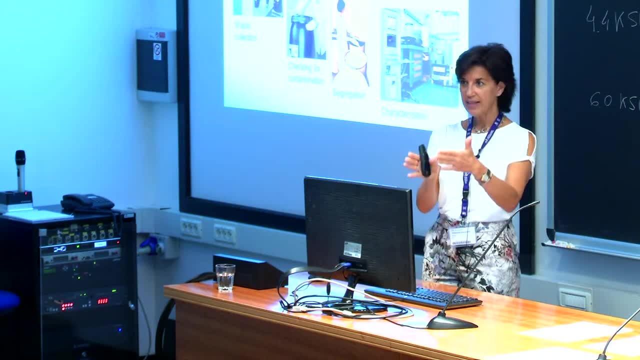 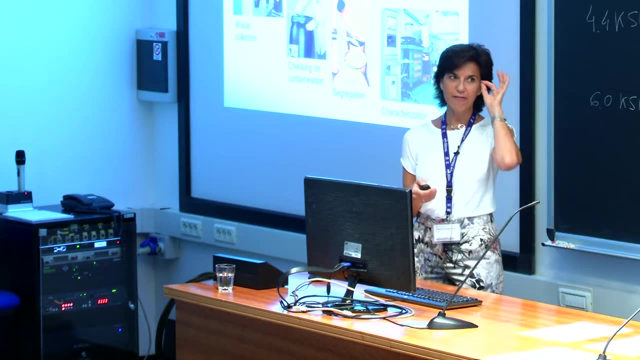 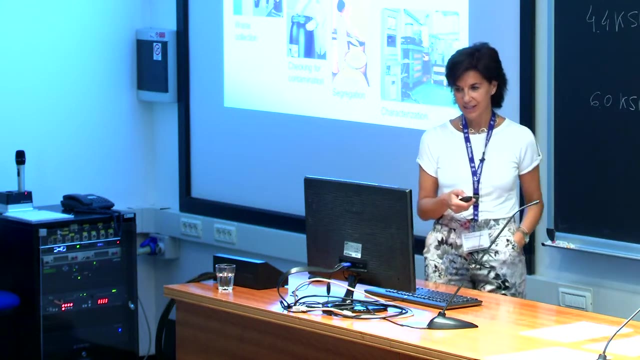 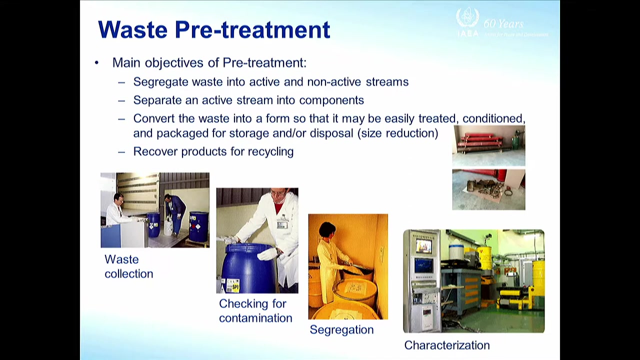 So it's very interesting to keep all the streams separately to avoid cross-cutting contamination and to produce huge amount of waste. So the first principle is to produce as low volume as possible of radioactive waste. So another objective is to convert the waste into a form that it's easily to be treated. 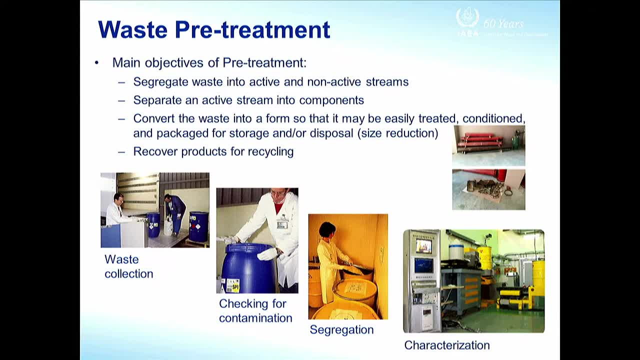 and conditioned and to recover products for recycling. So if we segregate from the beginning, it's easier to recycle some of the materials that if we put everything together and then we segregate. sometimes they are contaminated and they are not easy to recycle after. 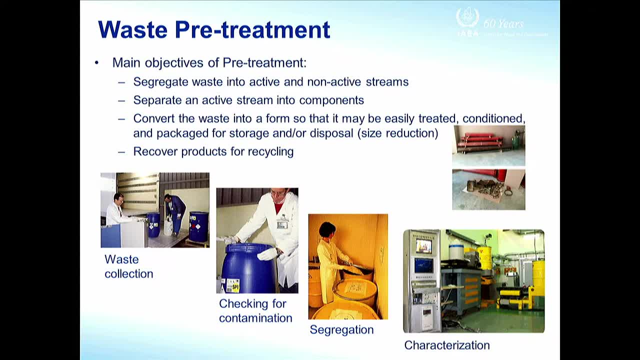 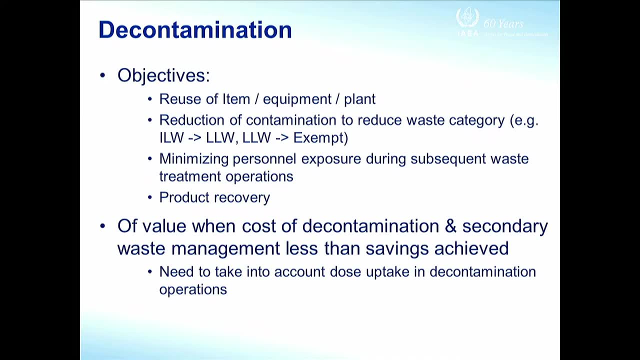 So the most important part, Part of this pretreatment, is the decontamination activities, that the main objective is to reuse the materials, to able to reuse the material and to reduce the contamination and sometimes, if the contamination can be avoided, the classification of the waste can be lowered from intermediate. 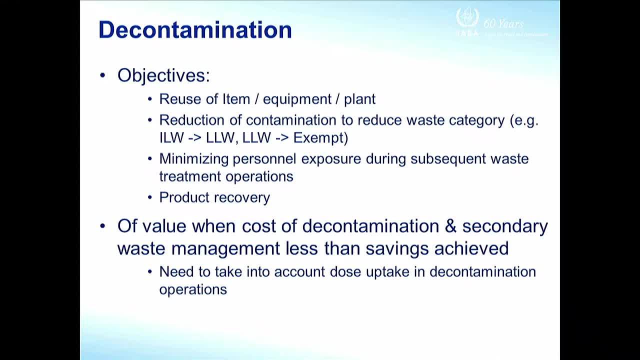 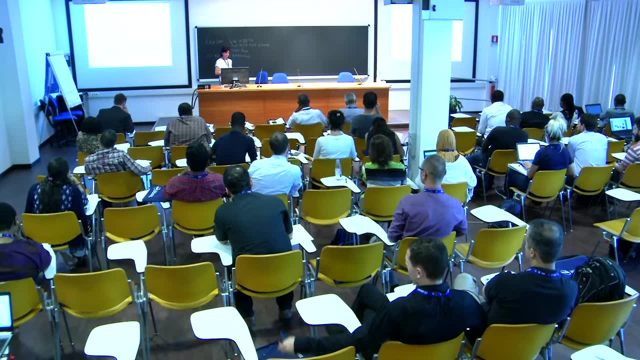 to low level That make it easier to recycle. Thank you, Thank you. So that's the first thing. The second thing now is to manage the, the waste, Also minimize the personnel and the workers' exposure and allow it's the product recovery. 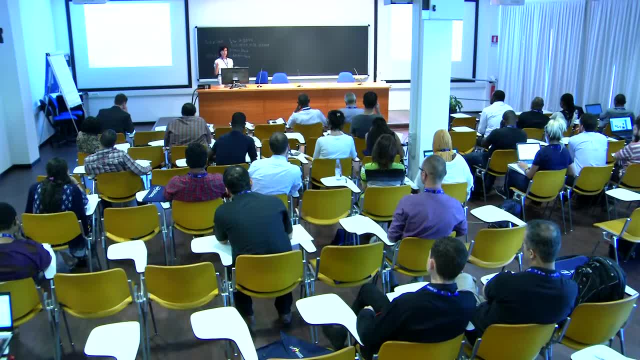 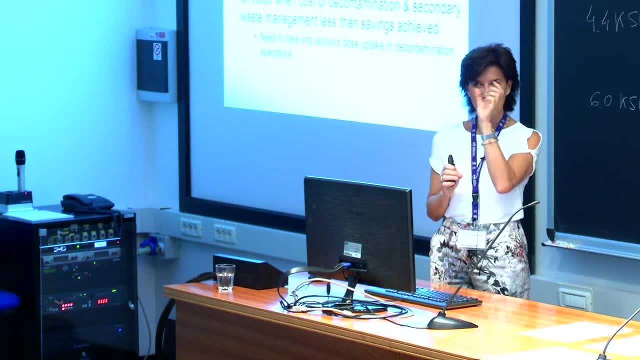 And always we have to keep in mind the benefits and the drawbacks of the contamination, because sometimes we have something contaminated in one cm- cubic cm- and it's very easily to manage because the volume is very low, and then if we try to decontaminate it, we create litres. 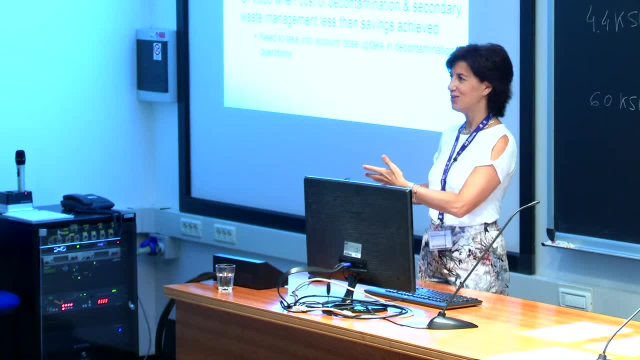 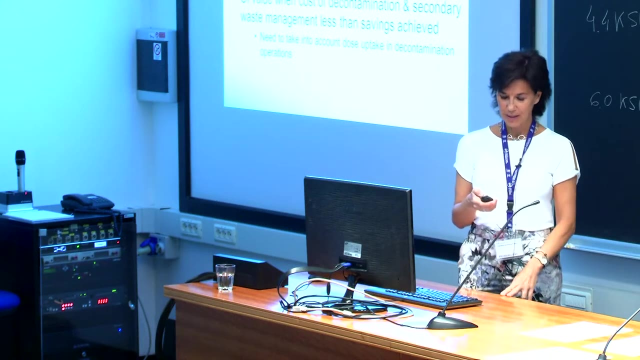 and litres of waste And- that's the most important thing- liters of contaminated water or contaminated organic solvent. sometimes it's much difficult to manage. so the balance between the benefits- economic and also from technical point of view- should be always keep in mind- and the characterization. so the characterization of 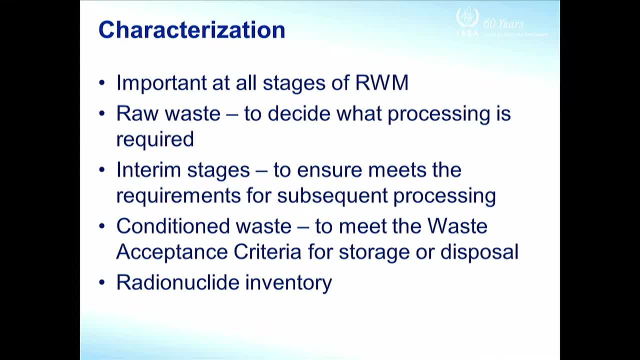 the radioactive waste is very important in all stages of the management of the radioactive waste because first of all, we have to know what is included, which type of contamination or which type of radionuclides are contained in the waste. also, it's important to have the inventory of the 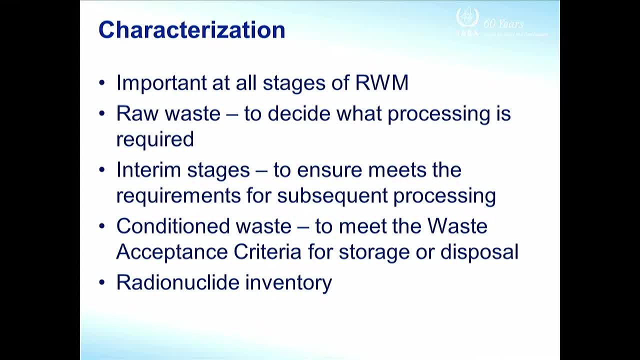 random clients stored or disposed in the facility. so, for example, in the case of a facility dedicated to low level, very limited to long live radio nuclides, it's necessary to know the inventory because the reward is not that much body never allows or the facility is not licensed for long live and applies the 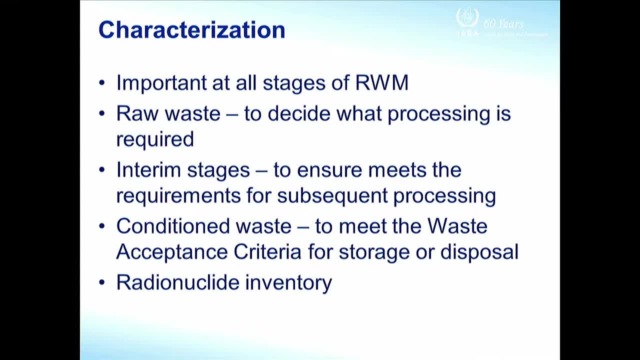 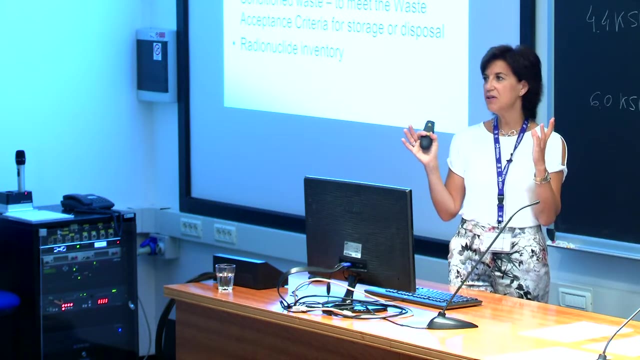 the level of alpha meters should be keep under a certain level. so the characterization is very important and it's not easy to characterize- to characterize radioactive waste, because the gamma meters can be characterized with non-destructive methods, because the gamma rates are difficult to stop. so with a detector, germanium detector, we can easily detect. 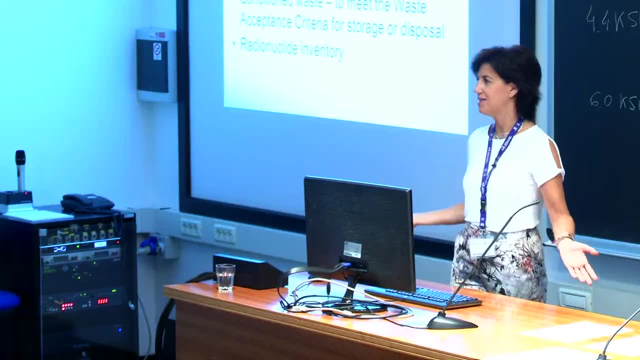 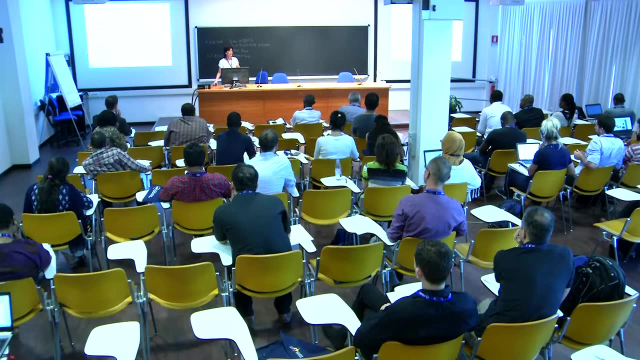 but what happened with the content of alpha meters, beta gamma meters, of the pure beta meters as strontium-19 or uranium plutonium that, not that emit gamma rays or very soft gamma rays? so they are very difficult to to characterize and it's necessary to develop. 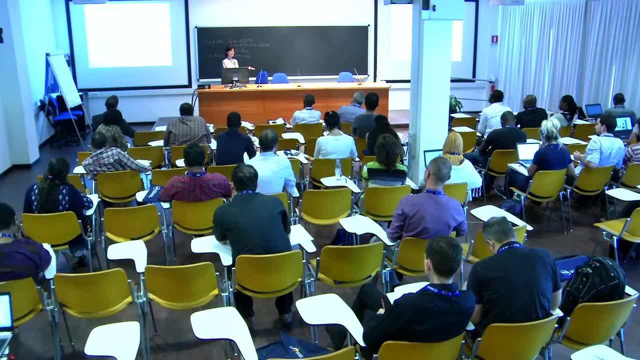 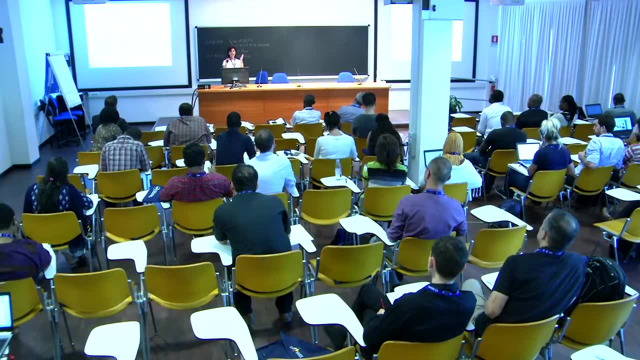 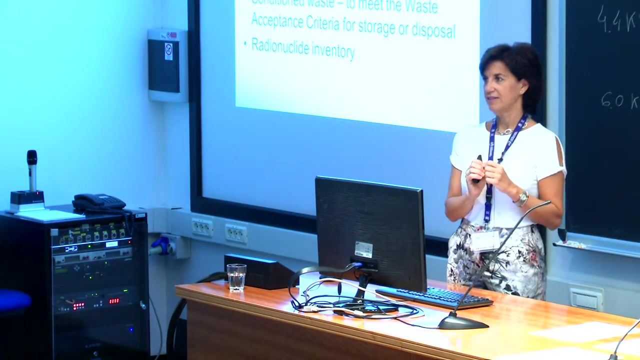 methodologies that, using destructive methods, can allow the facilities to get the inventory and then to apply the so-called correlation factors. so, measuring the gamma meters, we can calculate, knowing from where the stream games, the alpha and beta content. so it's not an easy task, the characterization, and it's very important. 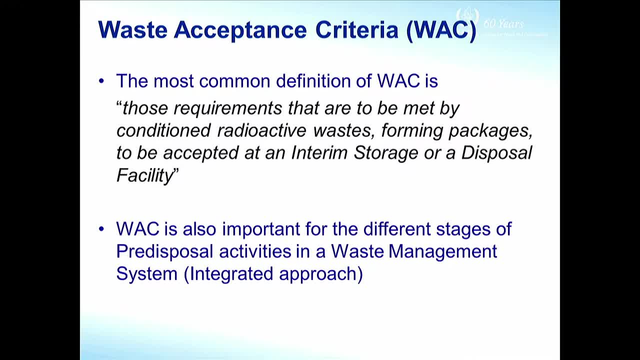 and it's also necessary to meet and to be sure that the waste meet the acceptance criteria. so the most common definition of the waste, acceptance criteria- and it could be applied also to a spent fuel, sorry- are those requirements that are to be met by conditioned radioactive waste forming. 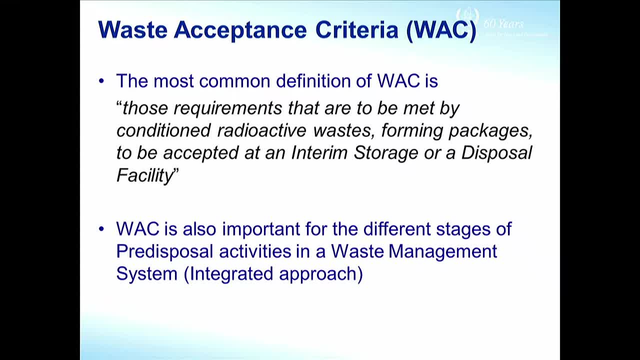 packages to be accepted at an interim storage or a disposal facility. but it's not only important at the final, for the interim storage or disposal facility is also the waste acceptance criteria are also very important in all different stages of the management because, for example, if we produce a 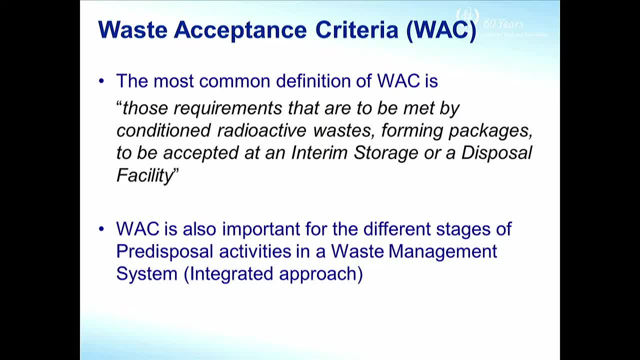 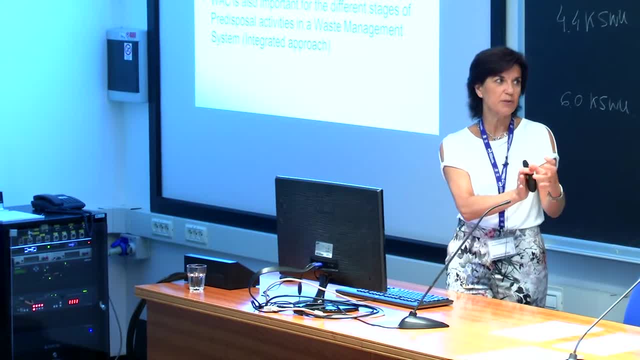 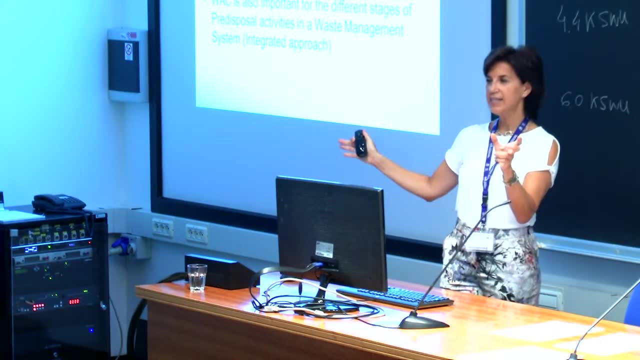 material. in the case of a spent fuel, if we storage the fuel in or we manage the fuel in in a certain circumstances, we have to be and to help. we have to keep in mind why, what, what is the next step, because sometimes decision-taking in one stages have a lot of impact in. 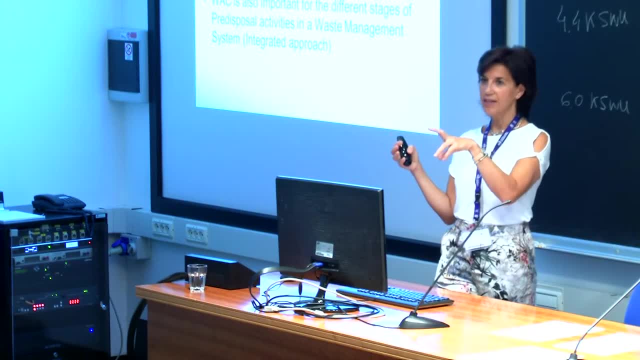 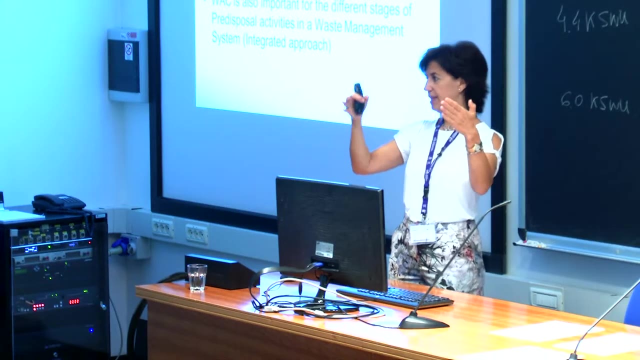 the second stage. so now the approach for radically ways and also for spent fuel management, is to have an integrated approach to the whole management, and then we are sure that the decision-taking in one stage doesn't have a lot of impact in the next stages of the process. 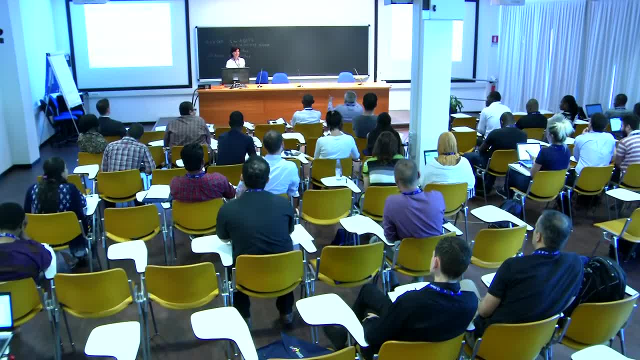 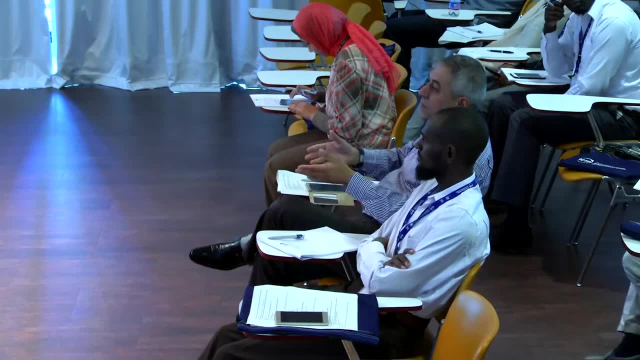 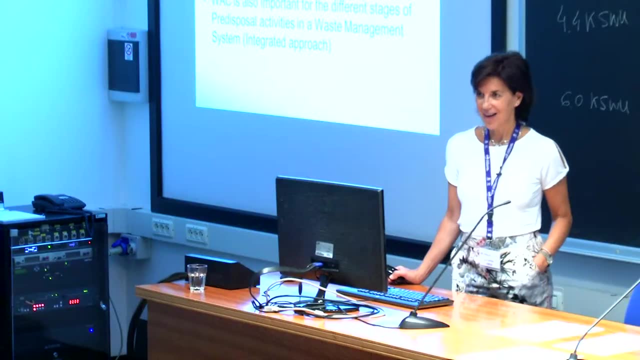 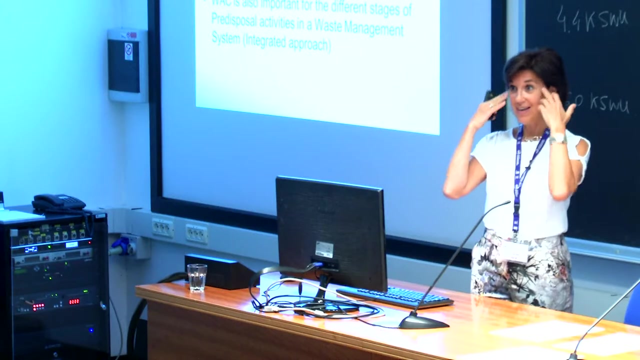 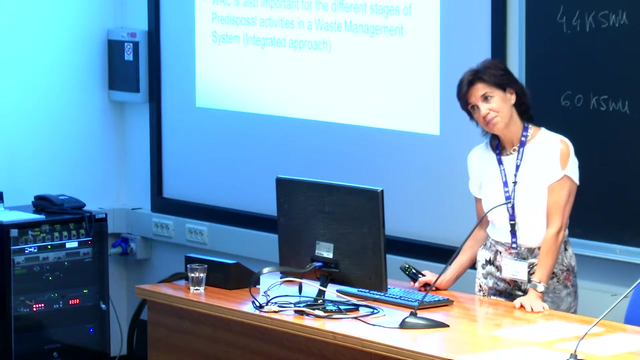 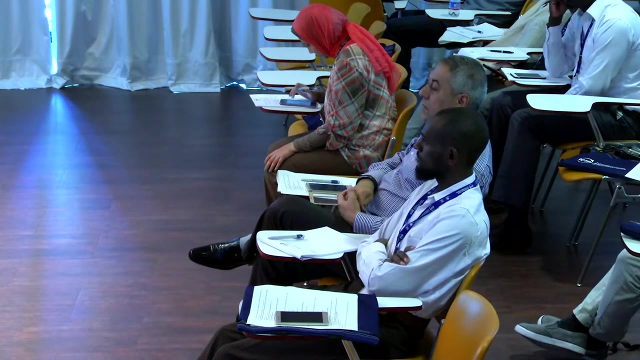 This is the issue. Yeah, that's why we are working now into an integrated approach of the different stages. It's very difficult to have in mind now what will happen in 60 years. Oh yeah, because, for example, in the case of radioactive waste, 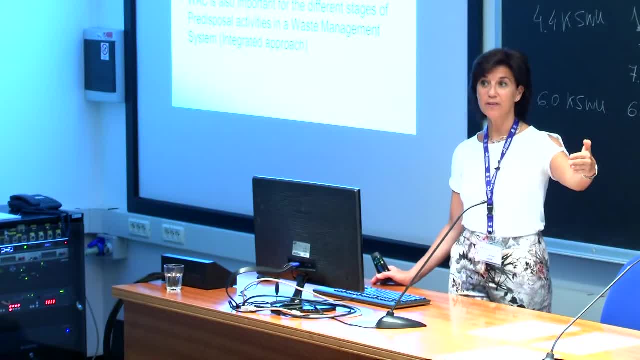 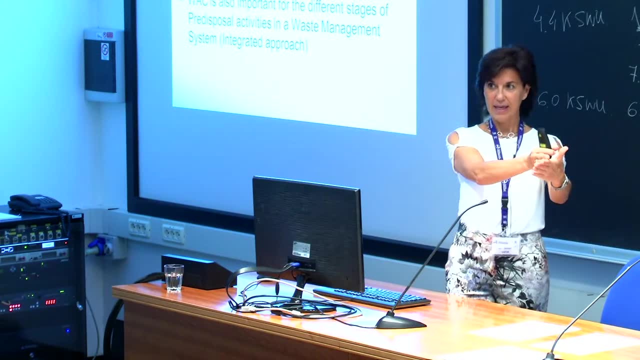 you know what the disposal facility, the requirements for the disposal facility are. You know, So you have to have in mind in all the process the acceptance criteria at the end. And for the radioactive waste intermediate low level, it's not that difficult. 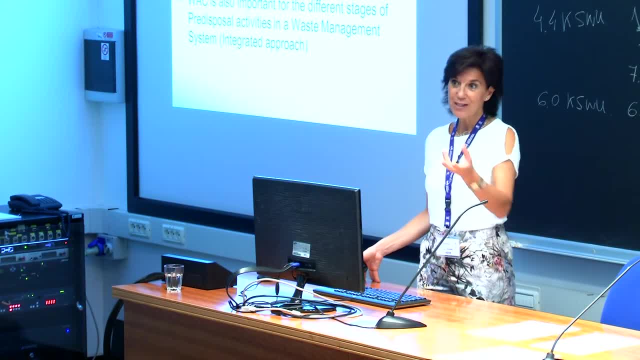 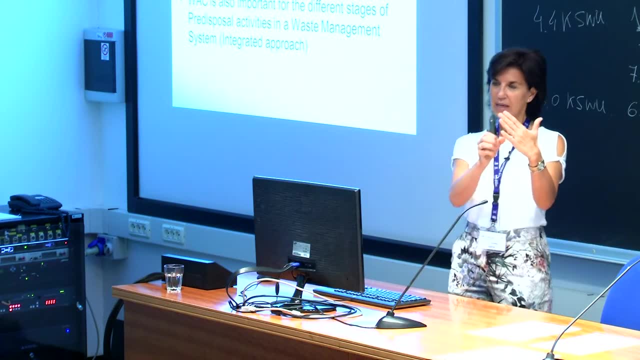 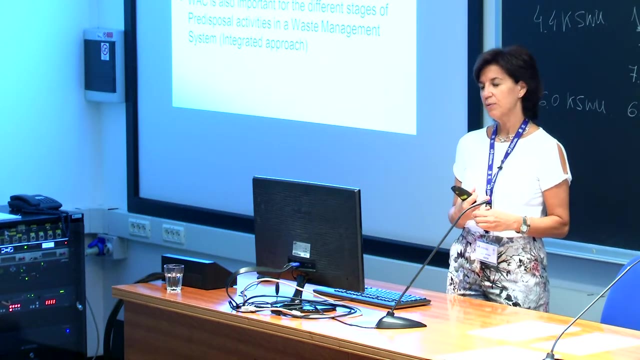 because the facilities are now in place, But for a spent fuel storage, for a spent fuel disposal, for example, it's very difficult to have in mind. So now we have a meeting, a big meeting. It was a conference in 2015.. 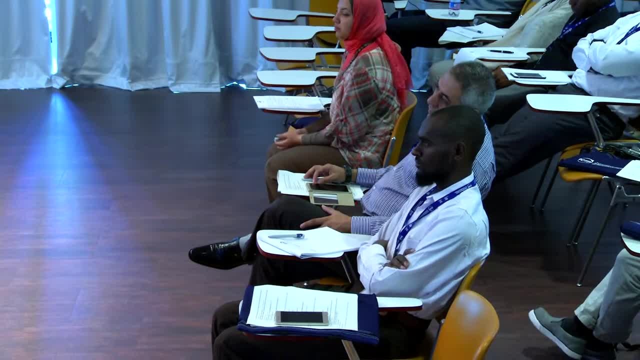 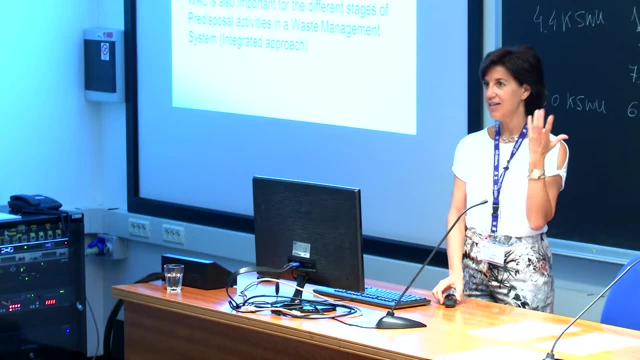 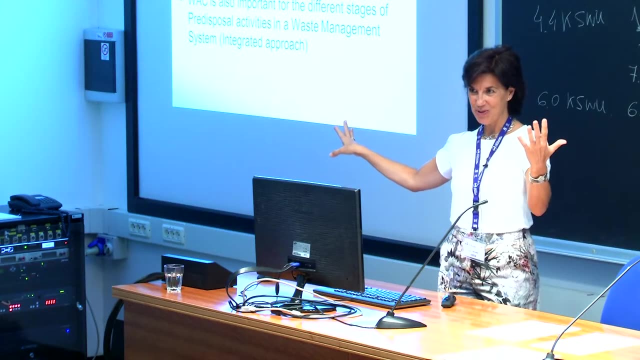 And the main message of the conference on spent fuel management was we should approach the management of spent fuel in an integrated way And the communities have to talk to each other, because the community dedicated to storage doesn't have in mind disposal issues, Even in the agency, for example. 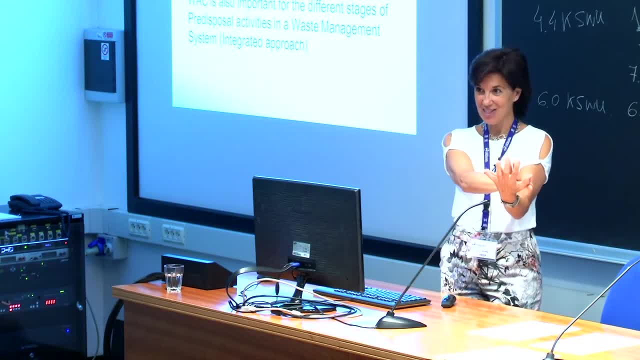 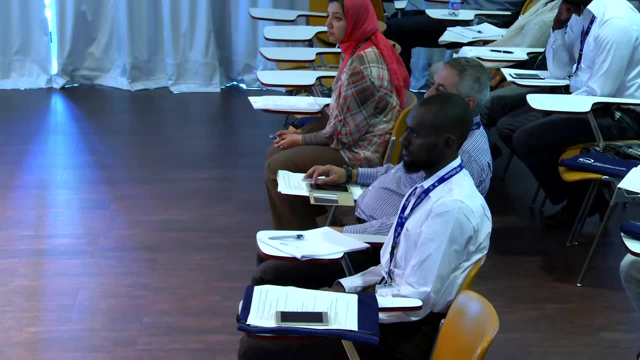 we are separated in different sections. So we are working in the storage in one section and they are working in disposal in another section And we have to talk to each other And we have to be aware what the needs in disposal have to have in mind. 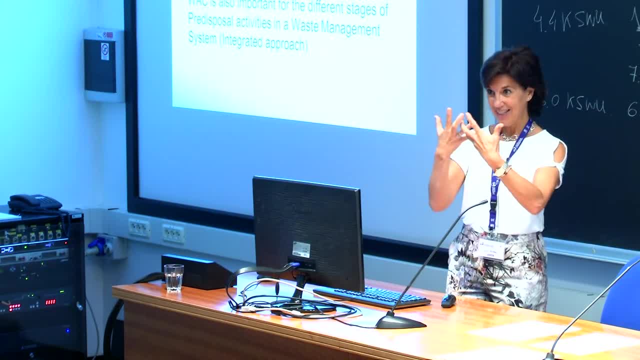 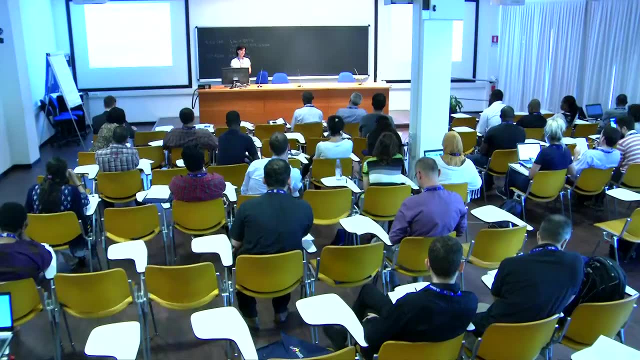 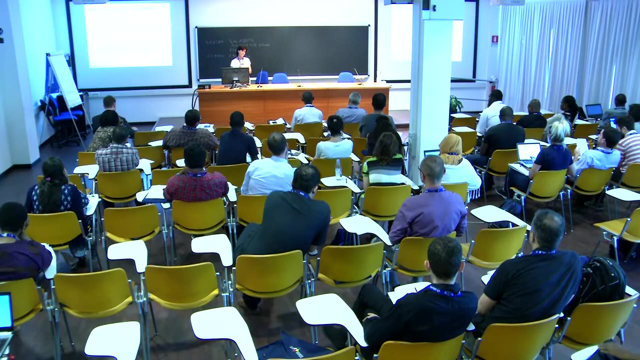 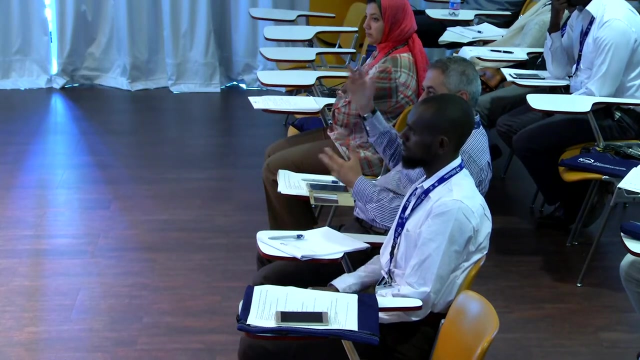 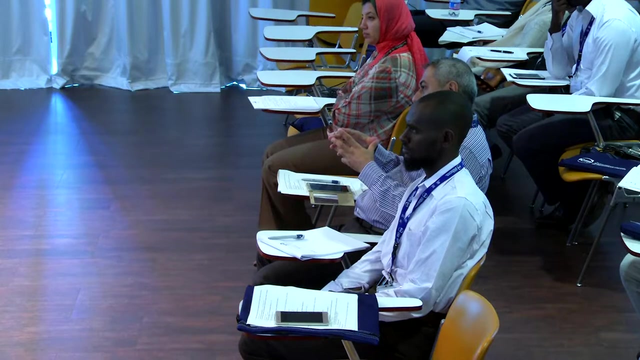 what is happening in the storage so far to be able to smooth the interfaces. So there's a lot of effort that applies to that because it's very difficult. So maybe take So in the ideal world we should have some acceptance criteria. 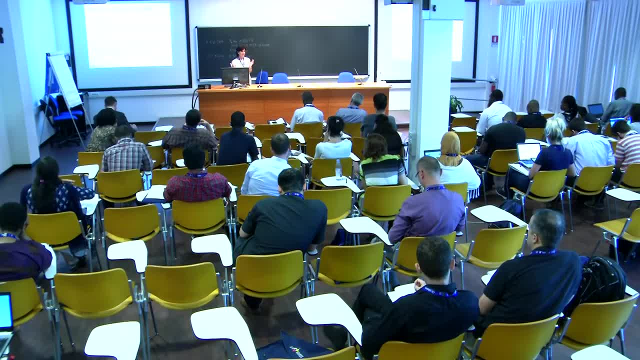 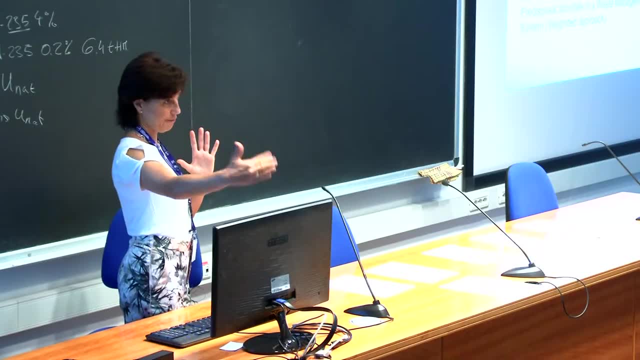 that of course the technology changes And maybe solutions in 60 years are completely different than we know now. But at least we should have something in mind for disposal and it should be known by the people working now in the storage to keep in mind that in the future. 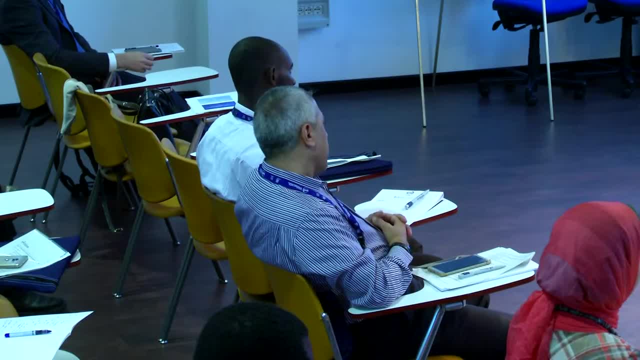 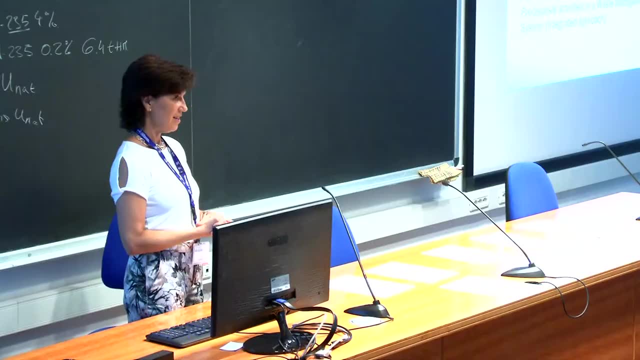 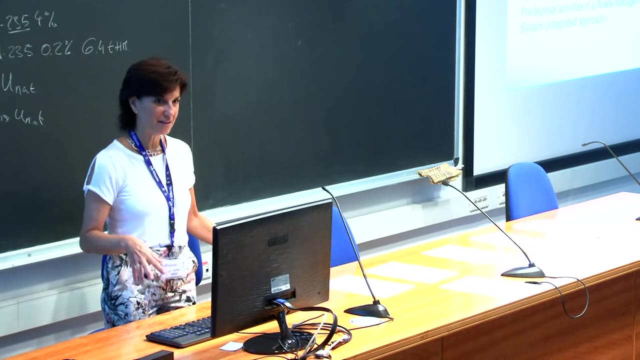 the constraints or the needs will be this and that and that, And it's not that easy, Even, for example, for the safeguards. if I explain like this, it sounds very funny and it's not funny. So we have a meeting in April. 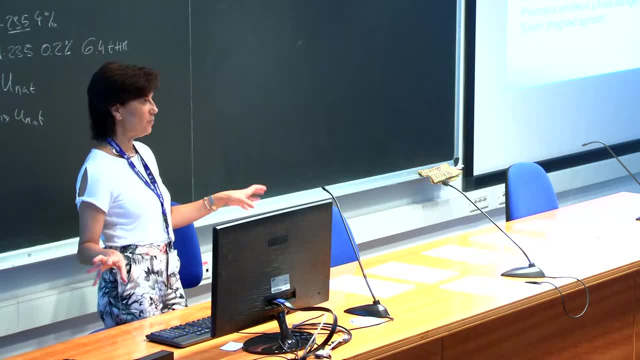 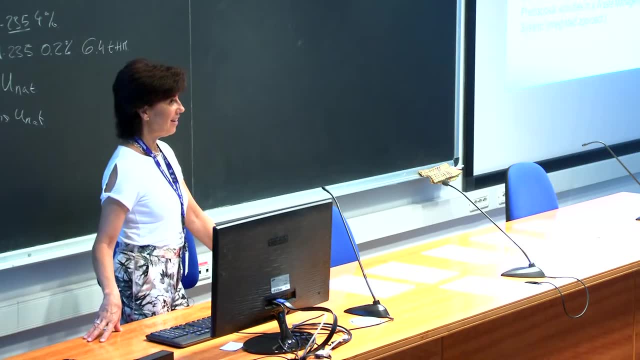 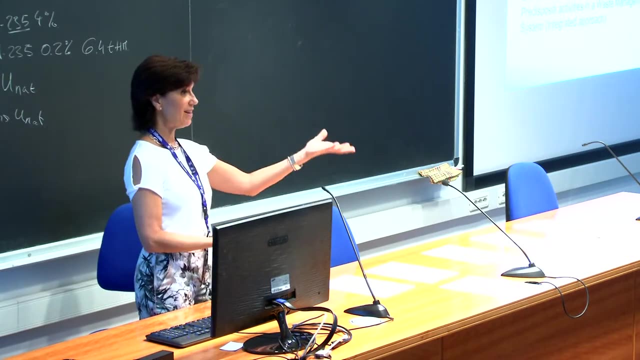 in the agency with the main actors in the world on disposal and storage, And then we invite a person from safeguards And the person from safeguards said: now we are working very hard with countries, for example, from Sweden, And the representative 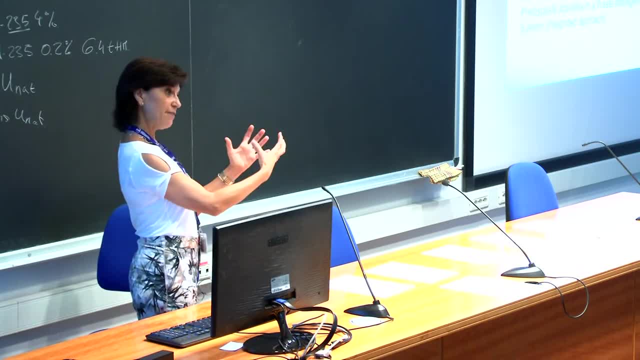 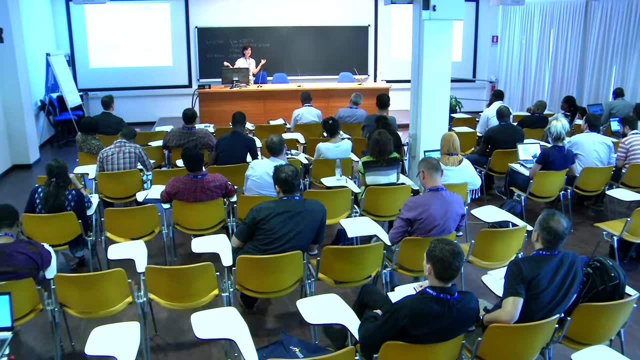 from Sweden said: ah, thank you, because they designed the facility for disposal without taking into account the safeguards requirements. And then the lady from safeguards said: and we need inspection here, inspection there, inspection there, And then, once the walls are built, 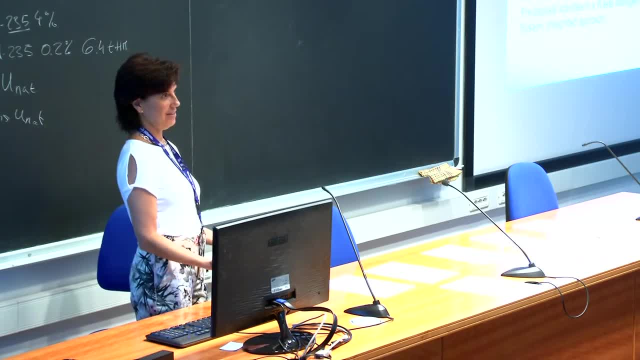 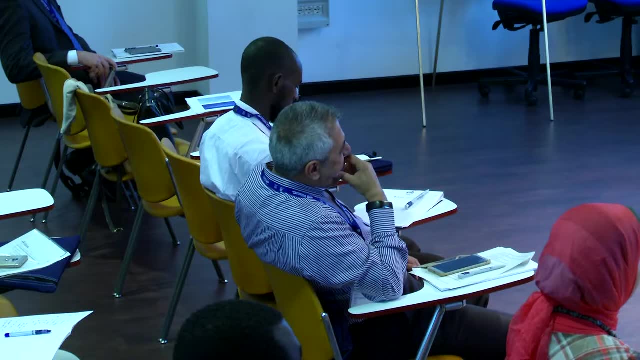 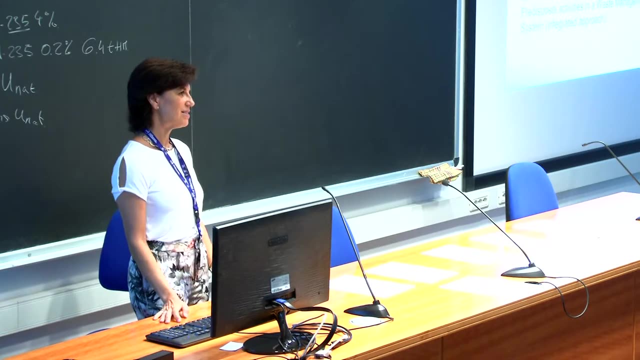 then we have to drill, Oh no, So it sounds common sense, but the communities are very isolated And a lot of effort now is applying to have in mind all the requirements in the disposal or in the storage, but mainly in the disposal. 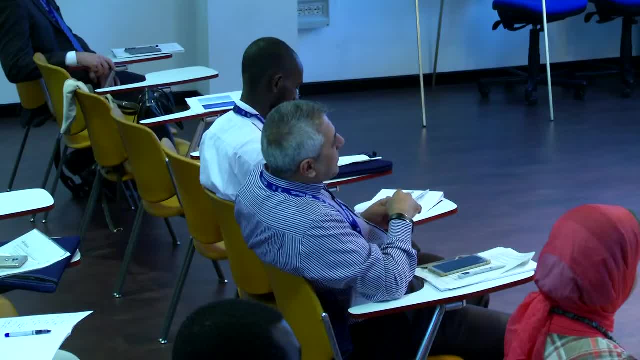 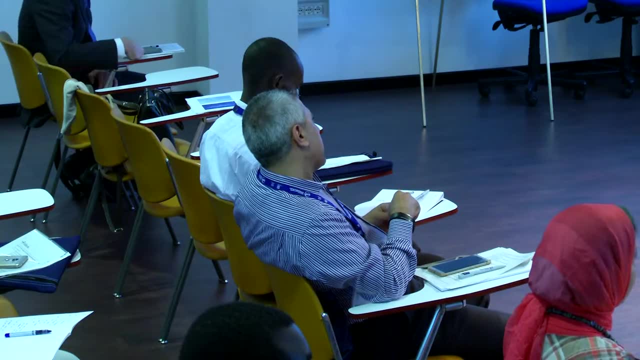 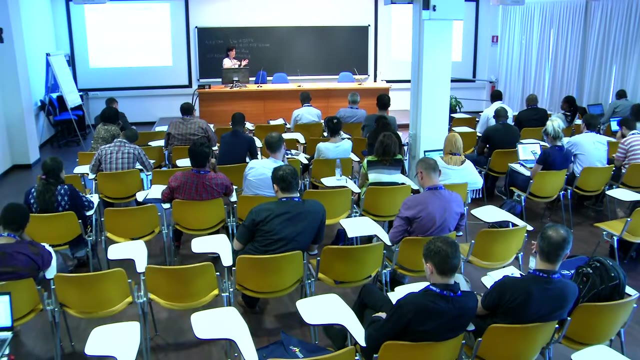 because it will last a lot of time. So it's not that it's very difficult And of course this is the general definition And as the waste are more difficult to manage, the acceptance criteria are more difficult to meet at the end. 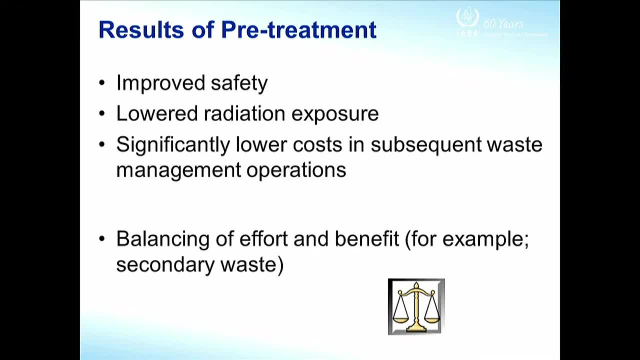 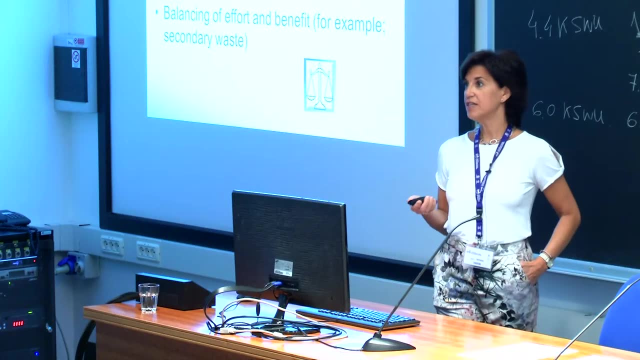 So what are the results of the pretreatment? So we will try to improve the safety, to lower the radiation exposure, And so we have to balance the effort and benefit not to avoiding generating a lot of secondary waste that sometimes are more difficult. 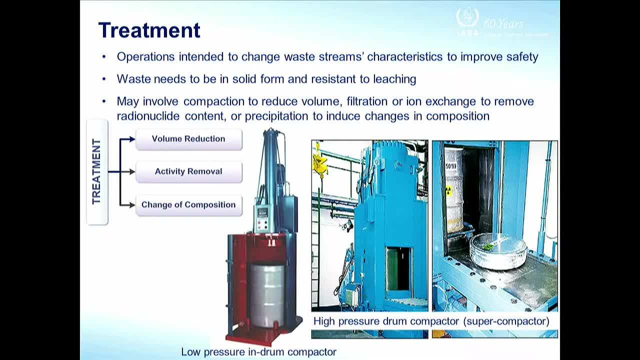 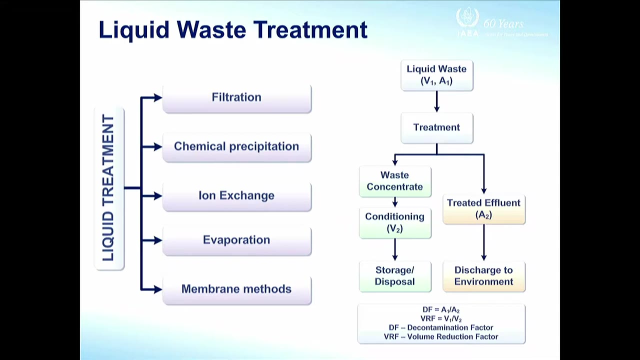 to manage than the primary waste Treatment. So there are different operations in treatment that, in principle, are dedicated to reduce the volume, to remove, when it's possible, the activity of the waste, to lower, classificate them, And we have some examples of liquid waste treatment. 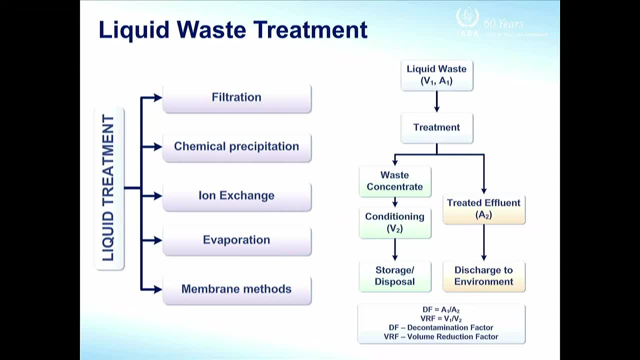 And, as you can see, they are dedicated to reduce the volume. So, after filtering or evaporation, distillation or ion-contained resin purification, we can have reduced volume of waste and we can, in order to condition, lower volume, But sometimes it's more difficult. 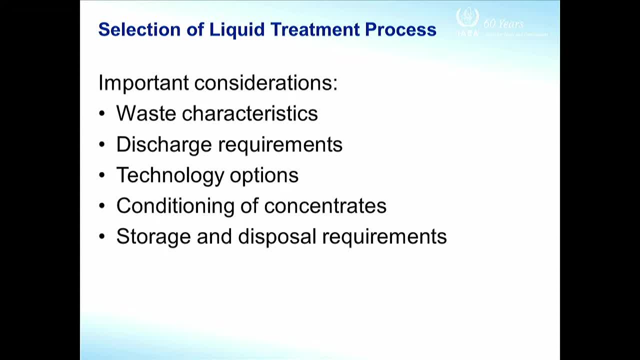 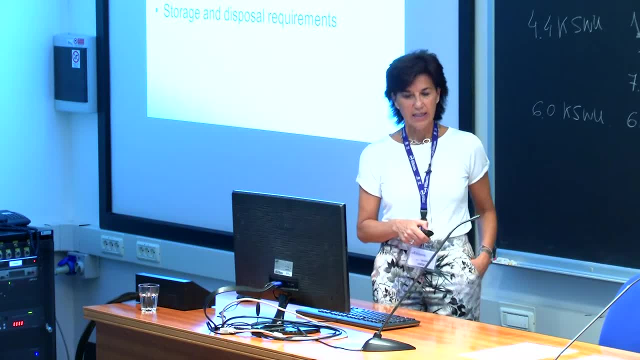 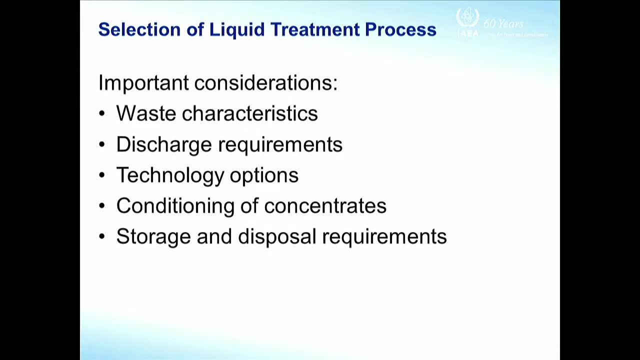 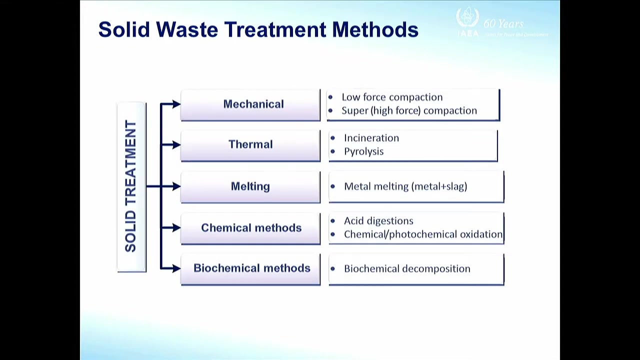 so we have to keep in mind that sometimes the conditioning of the concentrators are more difficult than the conditioning of the waste itself. An important consideration to choose the treatment is the characteristics of the waste. Sometimes, for example, if we separate the liquid, 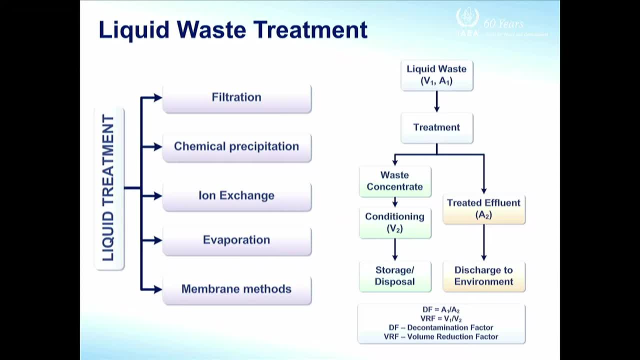 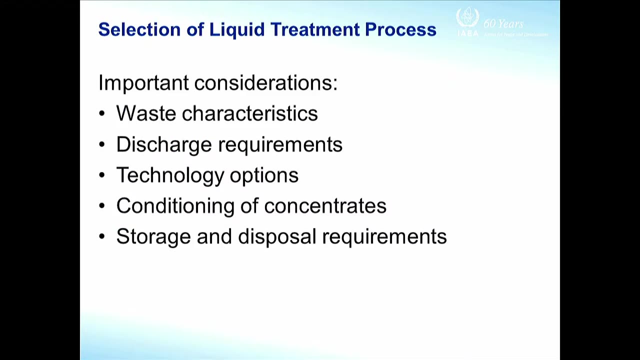 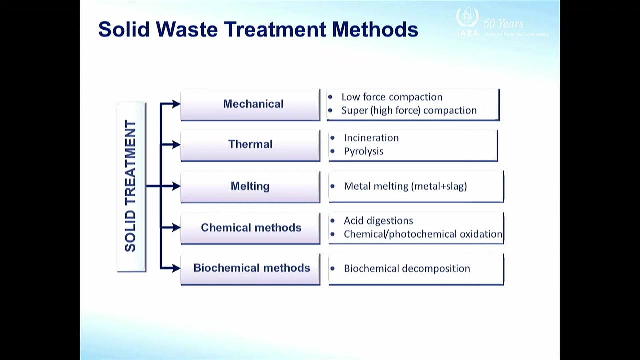 sorry- the liquid stream. by distillation we can have water and the concentrate and the water we can discharge, because by distillation we cannot have contamination. and in the case of solid waste there are different methods based on compactation and also melting or incineration. 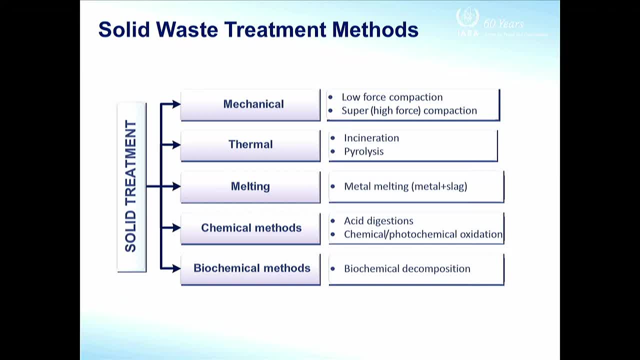 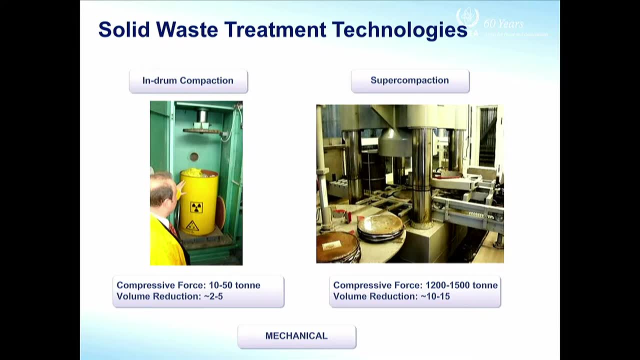 and chemical and biochemical treatments. So, for example, in the case of compaction, sometimes we can compact inside the drum. This is the normal harmonized 220 liters drum and a lot of volume of waste are produced in the operations of the gloves. 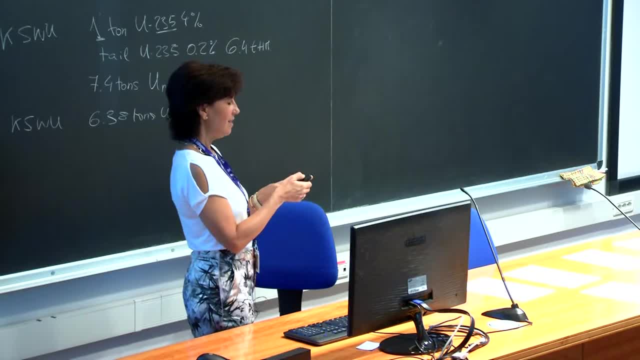 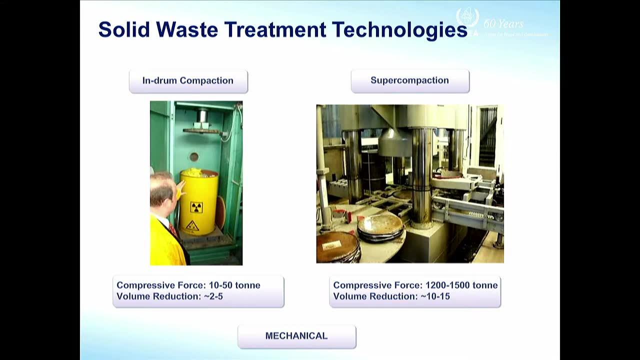 the cover, shoes, the clothes, the masks and this waste can be compacted to increase the volume that can be placed in one drum, or sometimes with the metal parts, as we saw during the reprocessing with the heels, for example, of the rods. 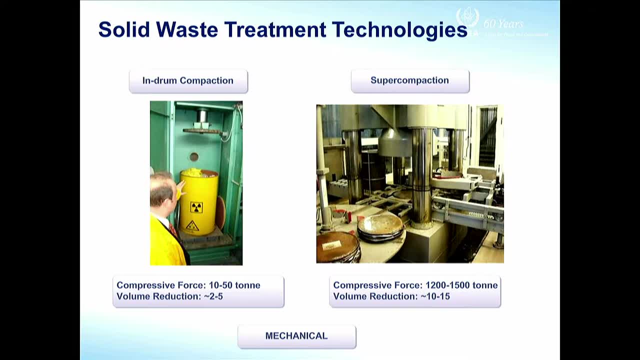 to reduce a lot the volume. So you can see here in the slide the volume reduction when we compact in the drum is 2-5 times and super compaction the reduction is 10-15 times and then we improve the volume in the repository. 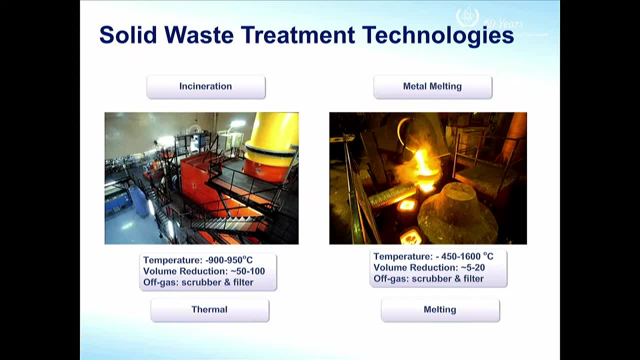 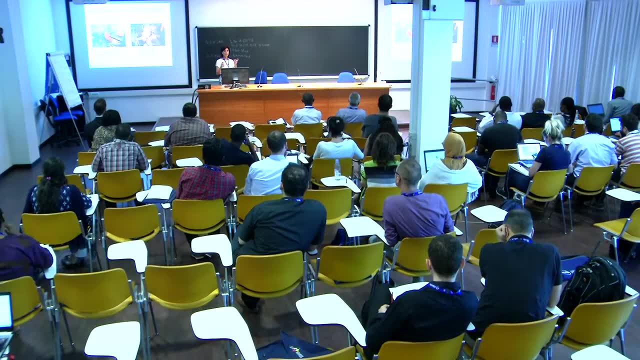 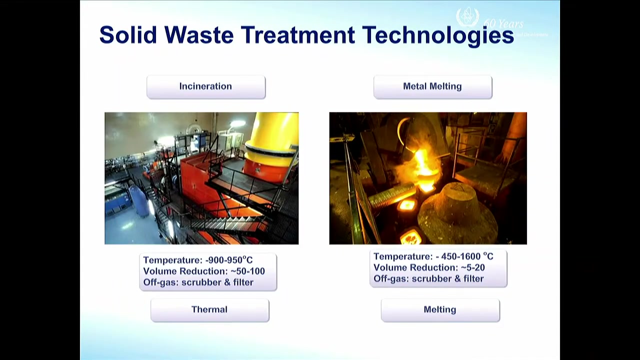 Other option is the incineration, and it's normal. the organic part is transforming CO2, water and we get secondary waste. the ashes and the volume is reduced dramatically. So we have volume reduction 50-100 times and melting is used during decommissioning. 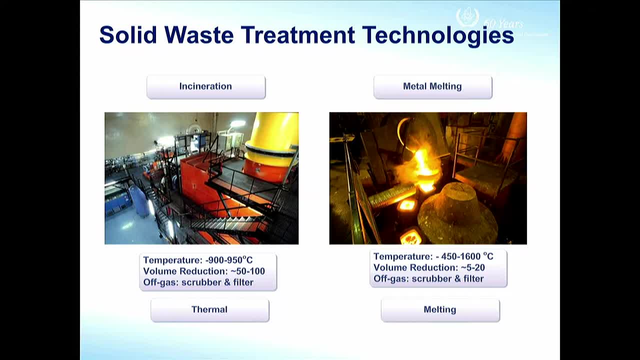 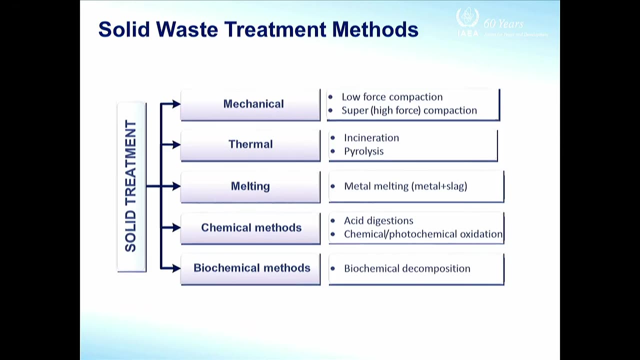 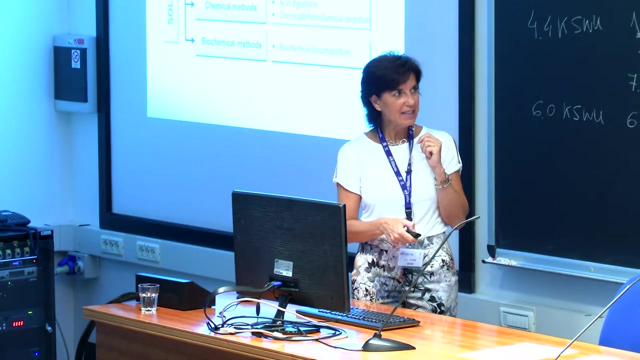 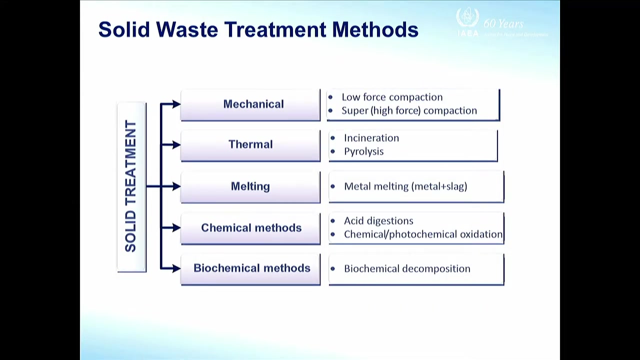 for example, some research reactors have shown that the aluminum part of the core can be melted and the products are separated in the result- metal- and also what it means in English, I don't remember the name- slag- has been proved that the main radioactive content inside the nuclear 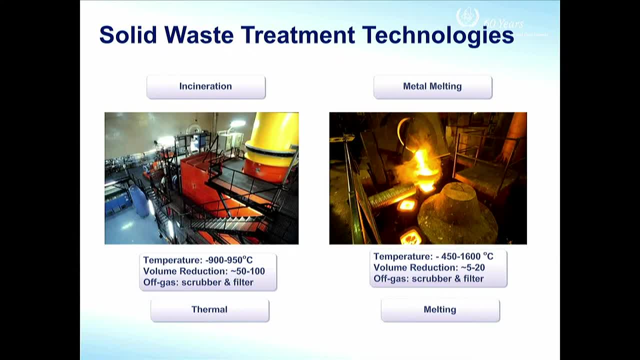 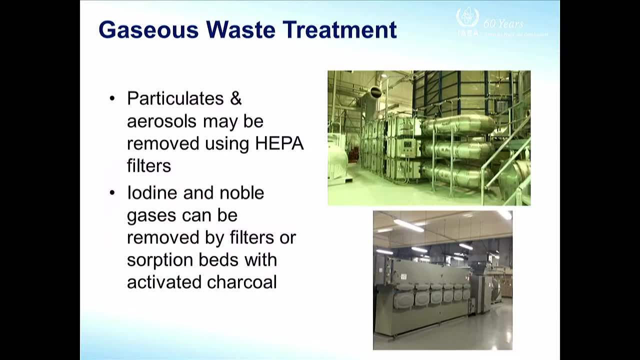 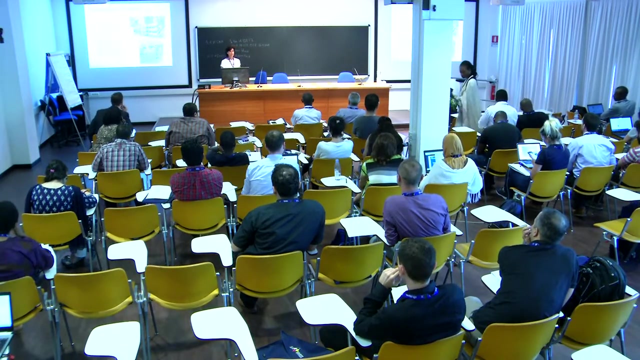 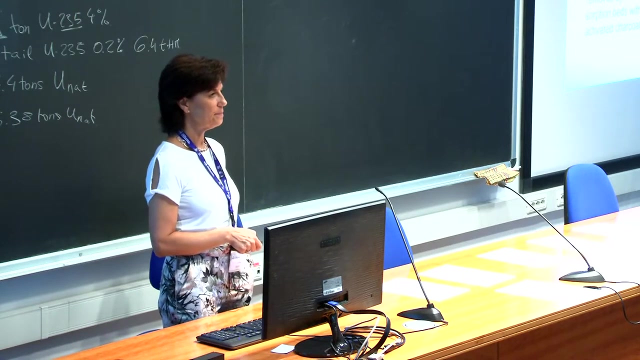 cycle. What about the filters? Sorry, What about the filters? Because you have, Yeah So, the off-gas. Yeah So the off-gas are treated with filters, with EPA filters, or also gases are trapped in insorption beds. Yes, Yeah, Yes, Depending on the contamination. 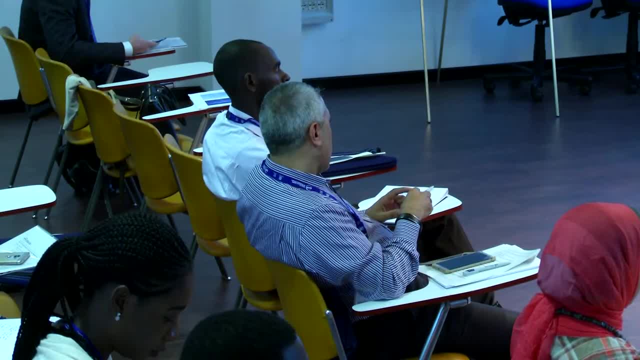 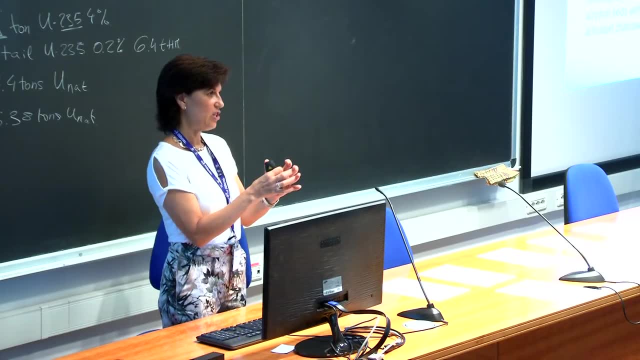 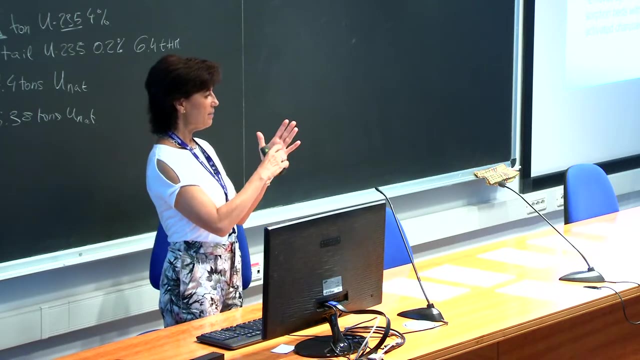 you can incinerate. for example, you can incinerate the filters if they are made of incinerable material. you can incinerate the filters and then get the ashes and manage the ashes. and yeah, sometimes it depends on the size of the filters and 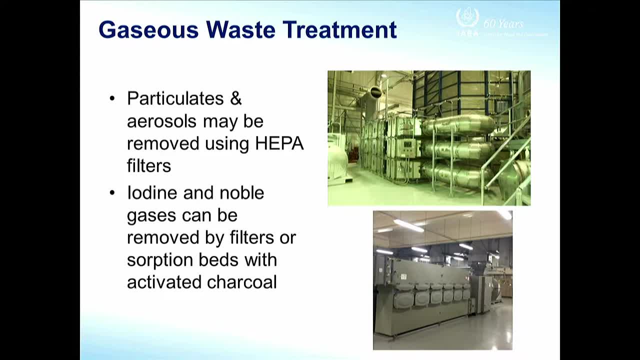 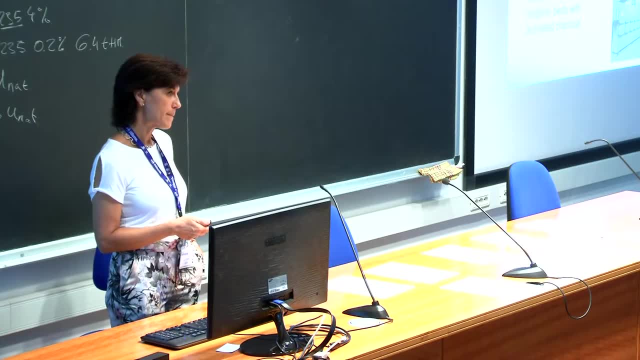 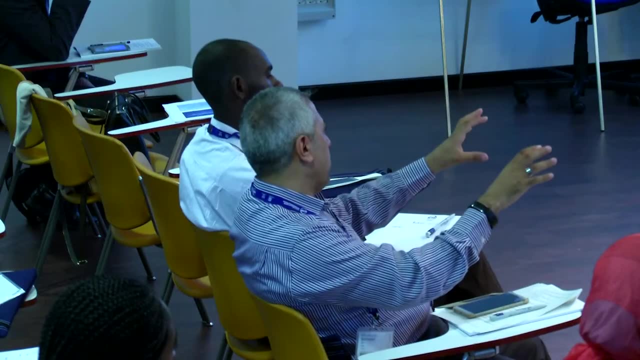 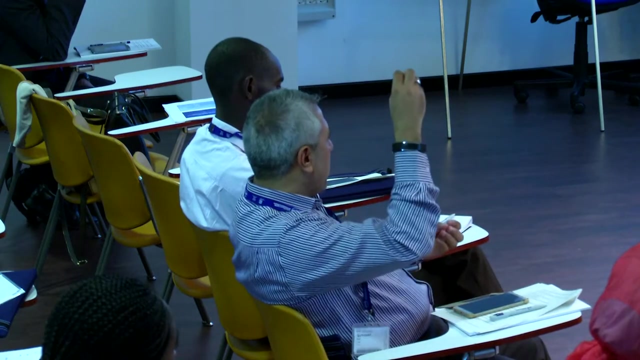 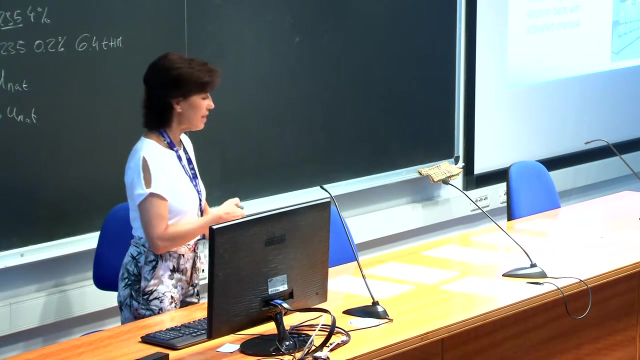 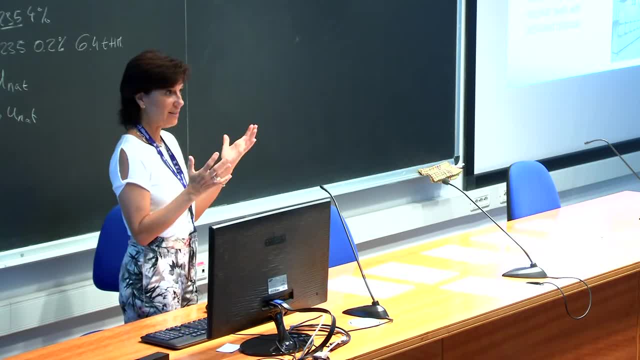 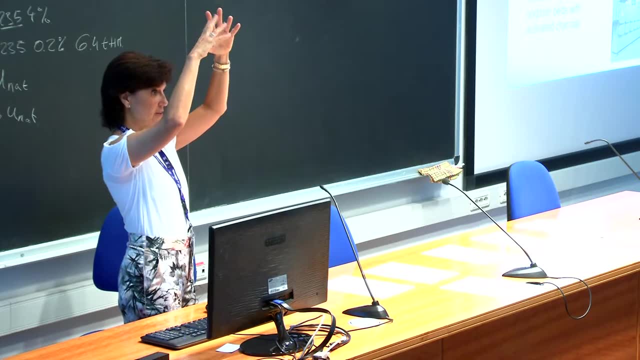 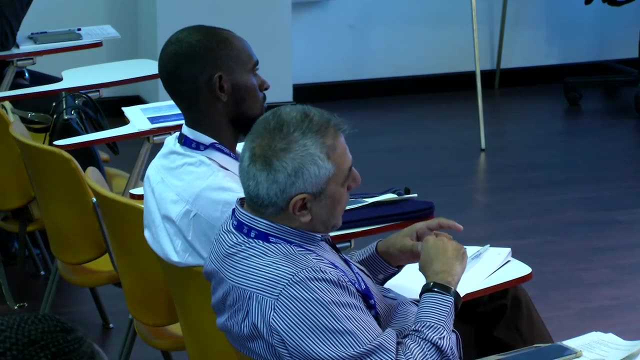 so the water condensate at less than 100 degrees so you can have lower condensation of water, and then the EPA filters above with avoiding to have water. you know what I mean. so you have a cool tower and then the emanations are cooled before. 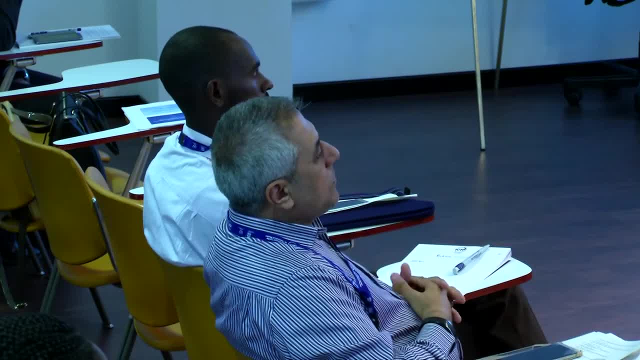 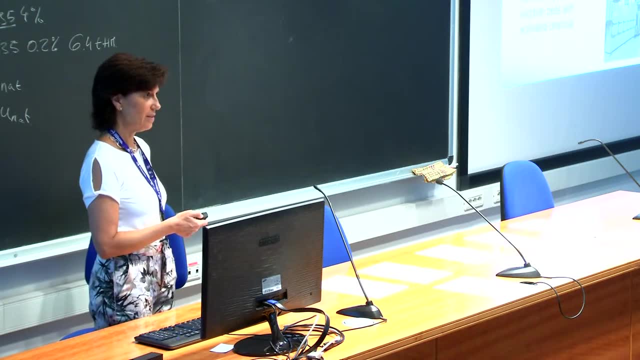 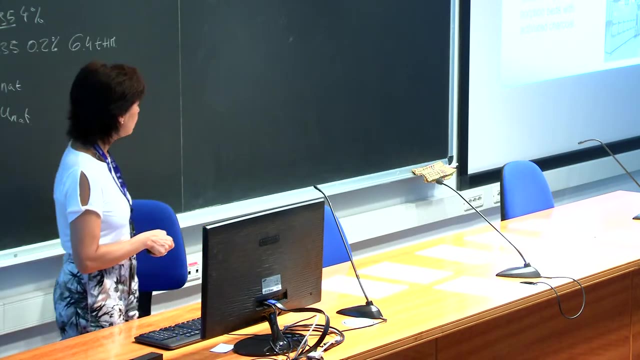 to get the filters that are sensitive to humidity, so you can work like this. I get so, because there are different steps in the filtration path, so of course the off-gas has to be treated, and this is, for example. this is for the case of the reprocessing facility. 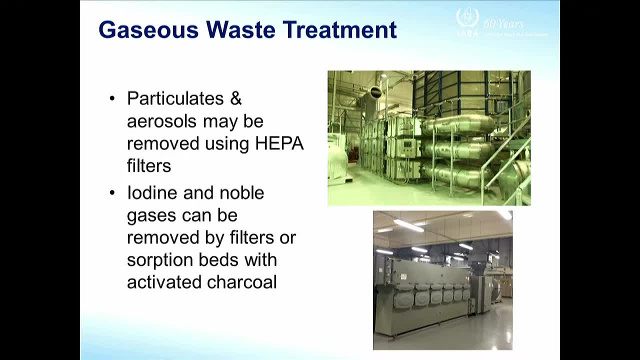 where the spent fuel is shoved and solved. the main radionuclides of gases contained in the spent fuel is the iodine and the noble gases that usually are inside the pellet or in the places between the pellet and the clad and should be these gases. 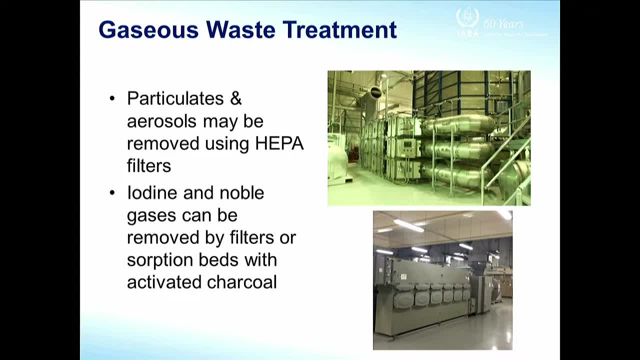 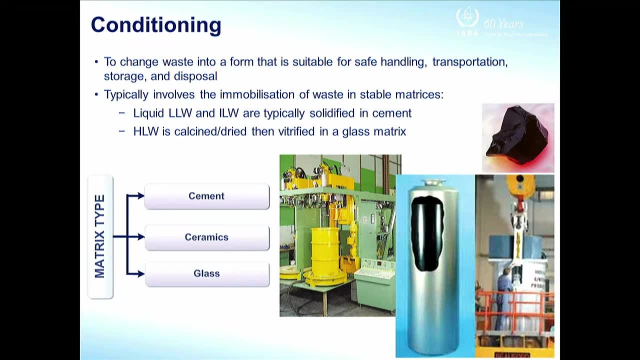 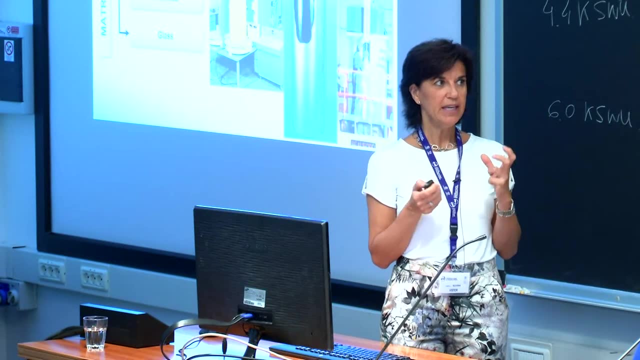 are treated by appropriate field sorptions beds. So conditioning- the conditioning is the main idea- is to solidify the waste and to put the waste in the form that the radioactivity will be difficult to be leached and to be released. so in the case of low level and intermediate, 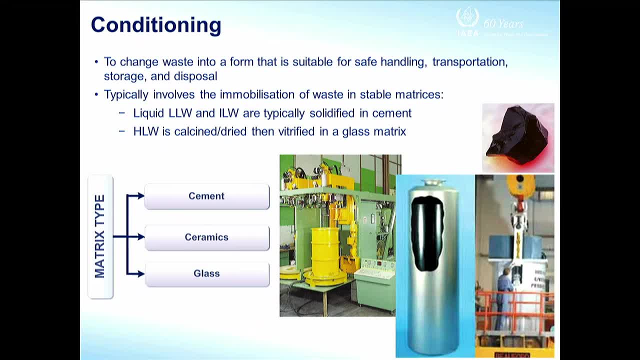 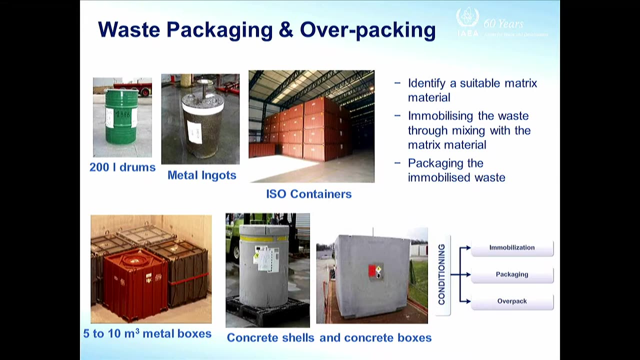 level waste, the cement is the more used matrix and in the case of high level waste is the glass matrix. There are different packagings, so once the suitable matrix is identified, it mixes the matrix with the waste and then is solidified and immobilized in a package. 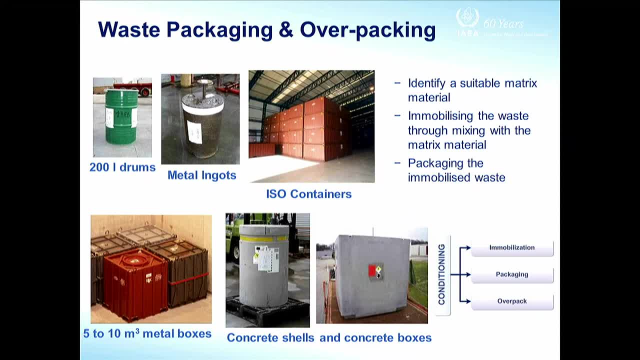 so this is a 220 liters drum and this is, for example, concrete packages for more active waste, because concrete stops the carbon emissions, and these iso containers are mainly used in the commissioning for sands for big volumes of radioactive waste with very low contamination and they are put like this. 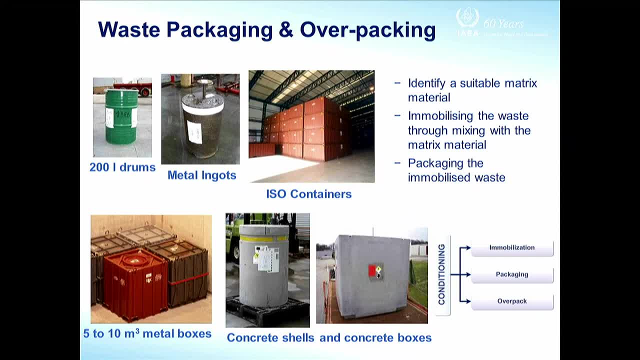 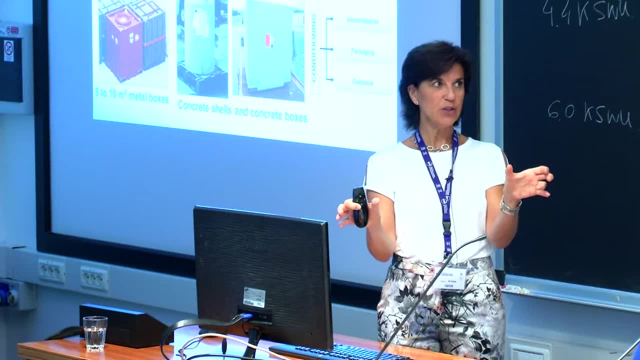 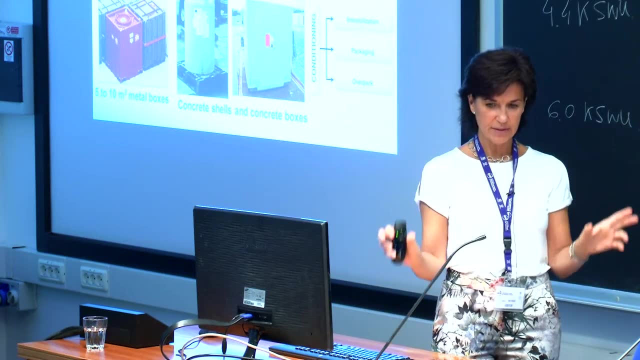 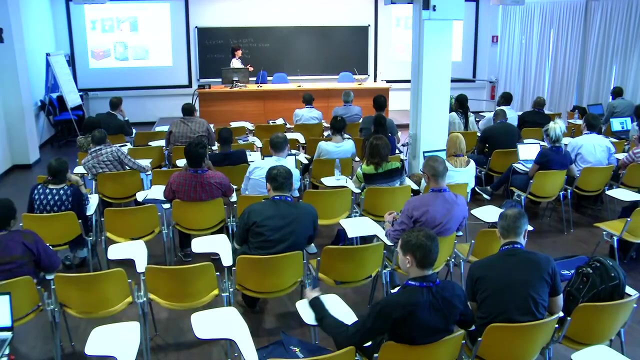 because there is design characterization procedure with three and three detectors. so the box, the box, the iso containers pass through the six detectors, and in a slow speed, and then it's detected if the content is below the certain levels, and then it's considered exempt or they are considered. 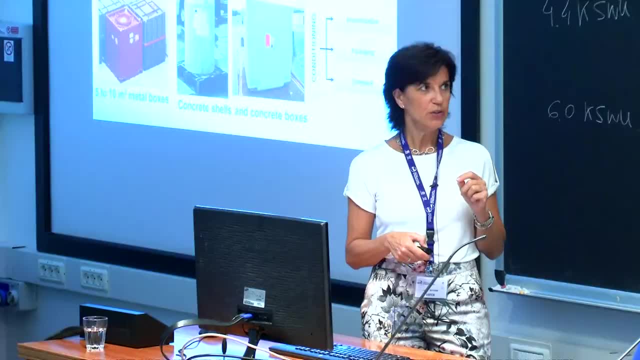 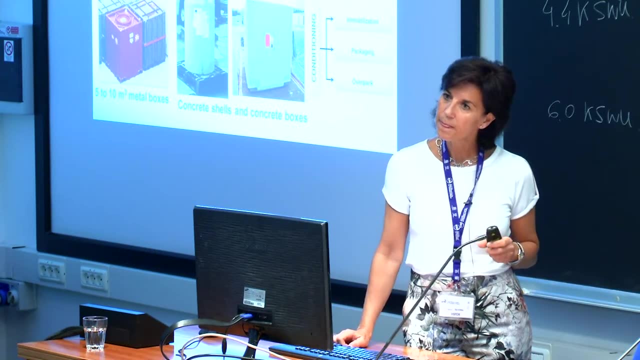 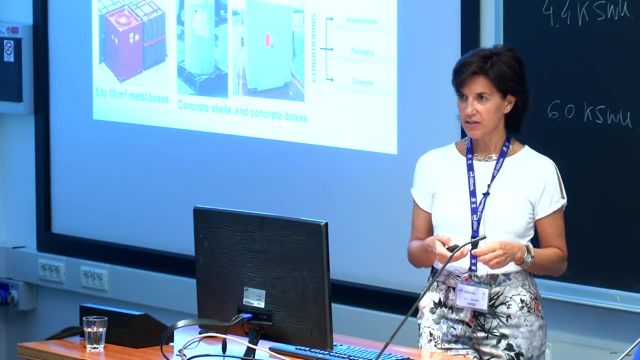 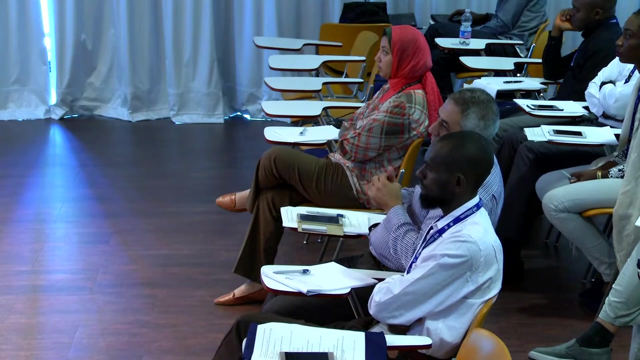 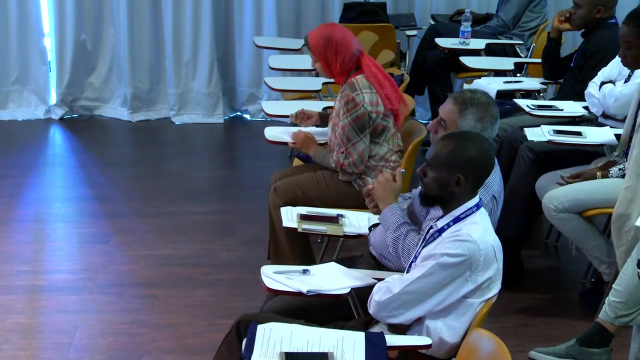 radioactive waste. so there is a harmonized procedure to characterize this type of containers. you mean the external corrosion or the internal corrosion? yeah, as far as I know, so far the concrete is improved to keep it safe because, for example, some facilities dedicated to low level are based on concrete. 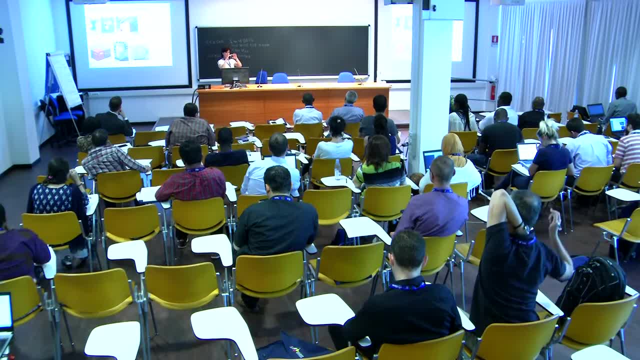 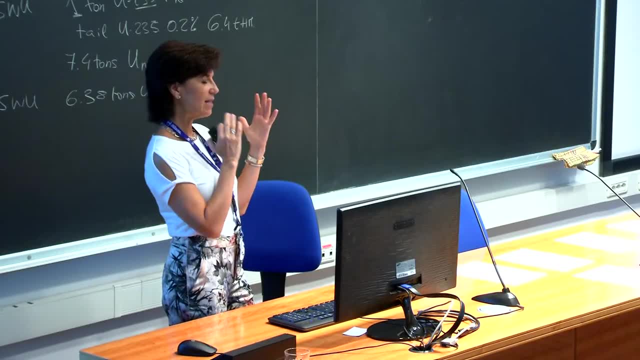 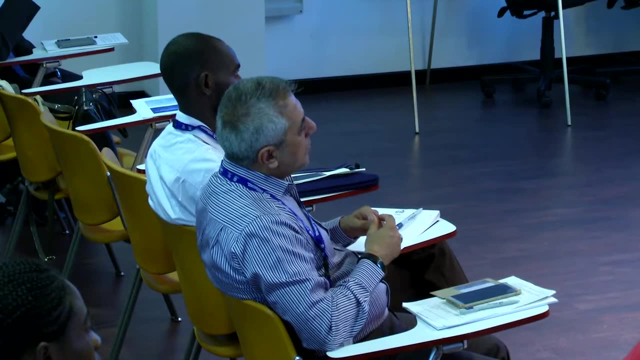 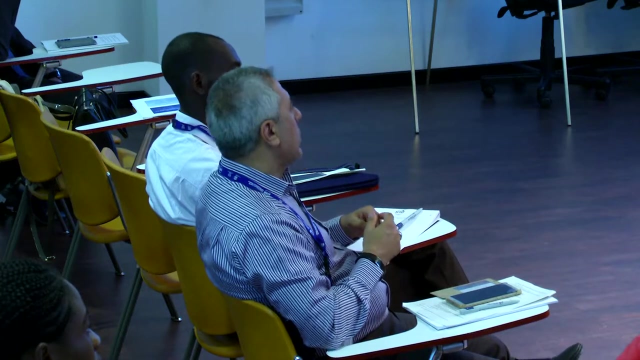 as immobilized matrix and also as a structural containment and as the buildings. so of course the concrete has to meet some specifications and requirements to be used in the radioactive waste facility as a matrix or as a structural containment. but I think, and the license, the facilities are licensed. 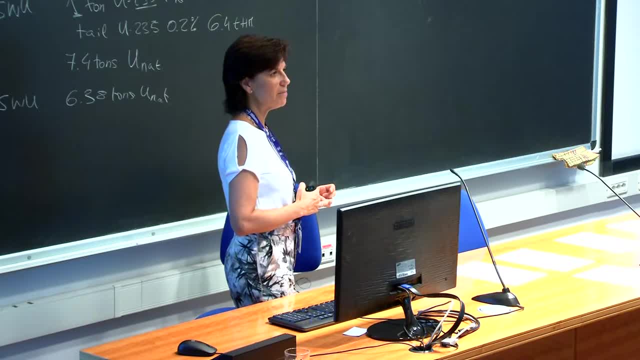 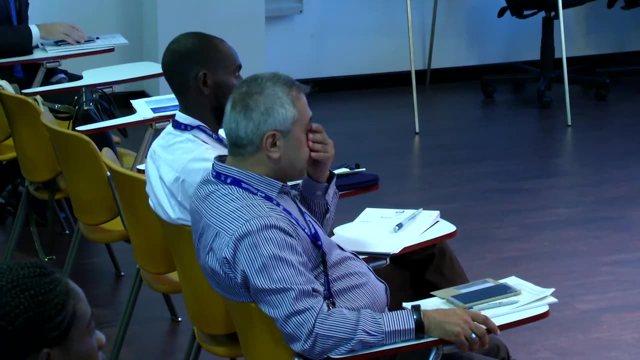 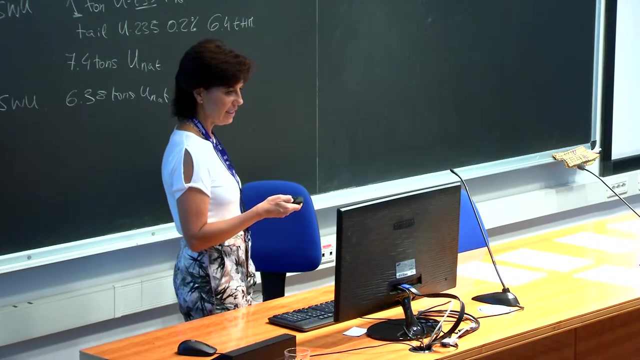 I think by 300 years, something like this, and it's proved that it's licensed by this time. so it's like the buildings, it's considered a suitable material, for example in the case we will see later, in the case of some facilities, at least in Spain. 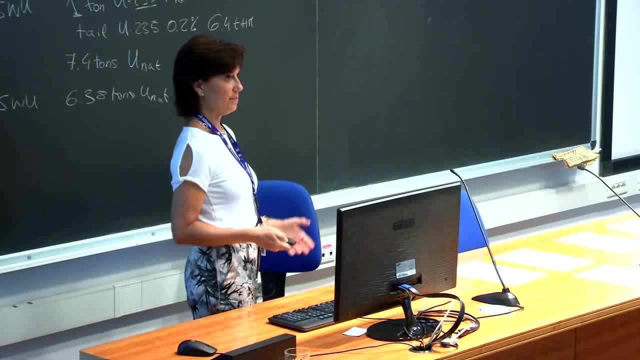 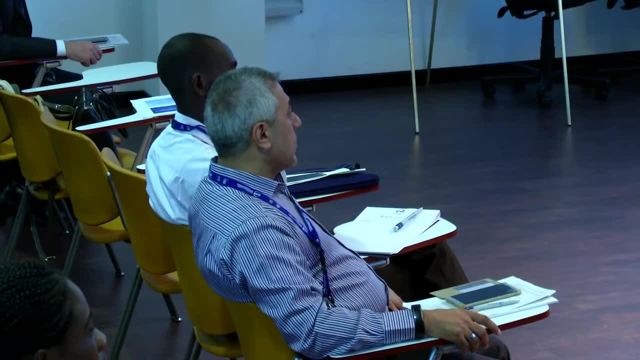 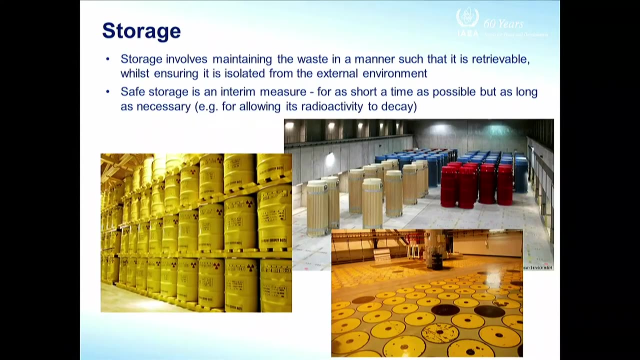 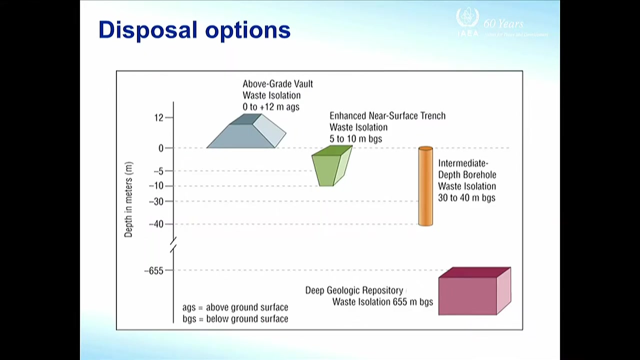 El Cabril is based on a concrete structure as a matrix and also different cells, plenty of trams and immobilized with concrete as a structural material. so after the conditioning, the waste have to be stored- I think we talk a lot about storage- and then have to be disposed of. 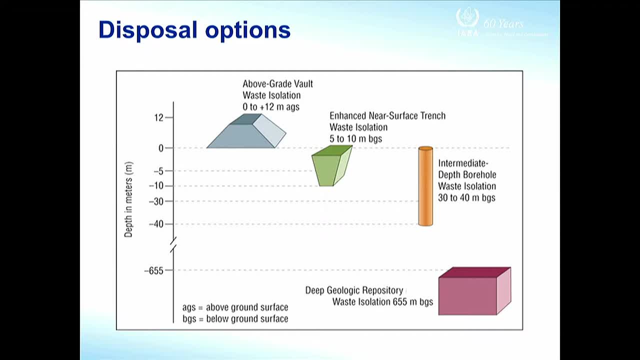 and this is the options. so for very low level waste can be stored in the surface. for low level waste needs to be stored in underground, but not very deep, maybe few meters depth. for intermediate level waste they need more isolation, so they have to be disposed in deeper. 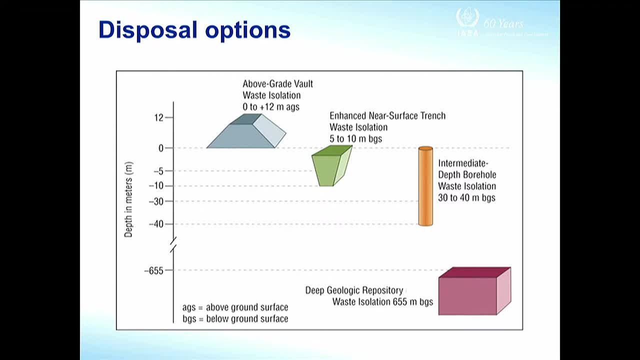 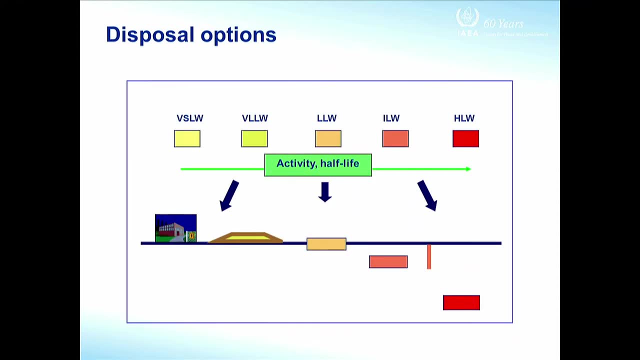 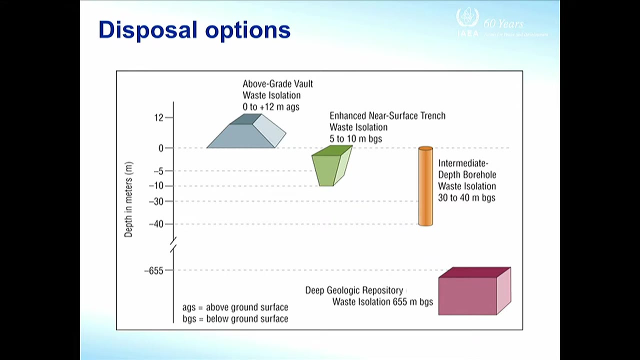 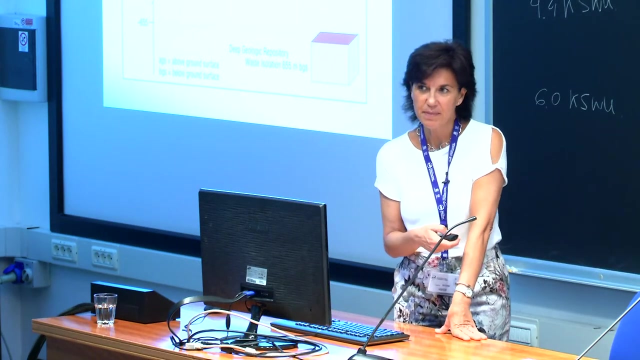 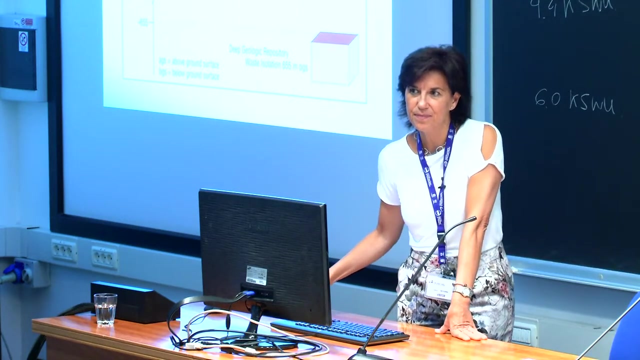 constructions and for high level waste or spent fuel is a deep geological repository. sorry, sorry seismicity, I think in any case, but it's more important in the case of intermediate and high level waste, but in any case, because if you put the surface repository in a seismic area, 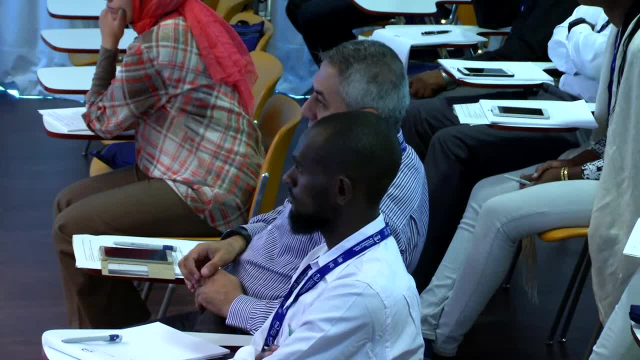 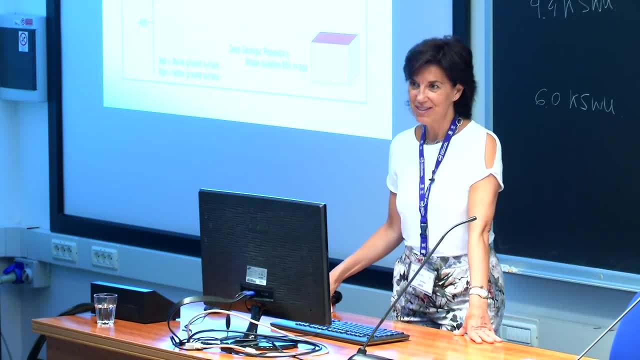 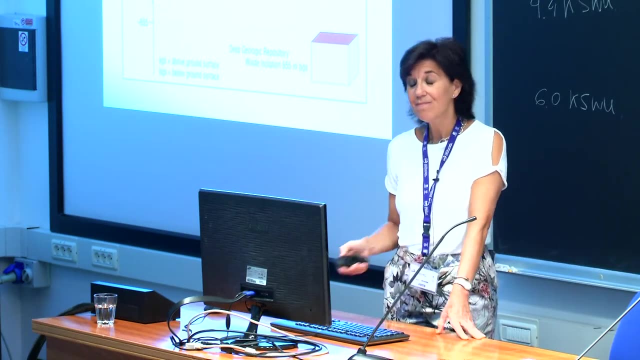 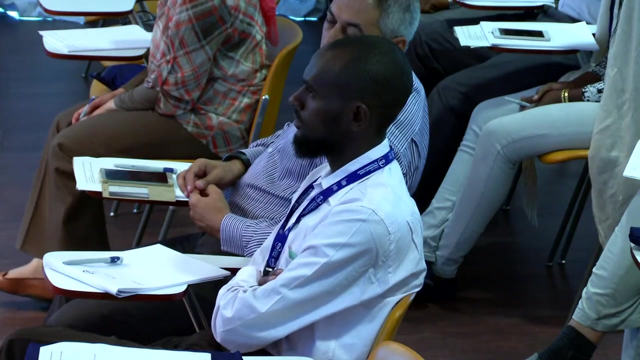 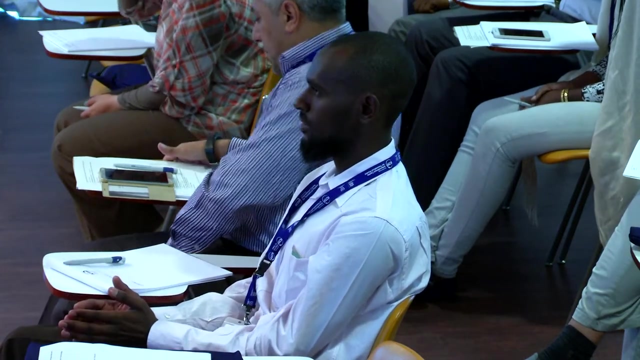 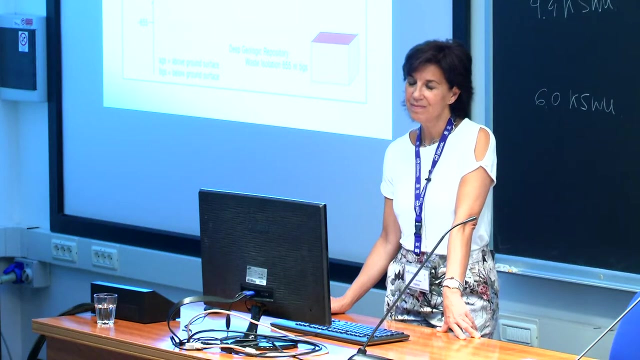 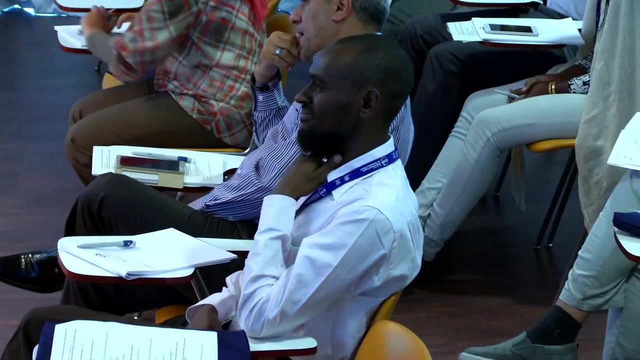 it's not good, but it's not a risk high risk. but in the case of intermediate or high level waste, it's one of the main parameters to be taken into consideration. this the same requirement? I don't know because I am not safe specialist, so maybe you should ask somebody from safety for license. I don't. 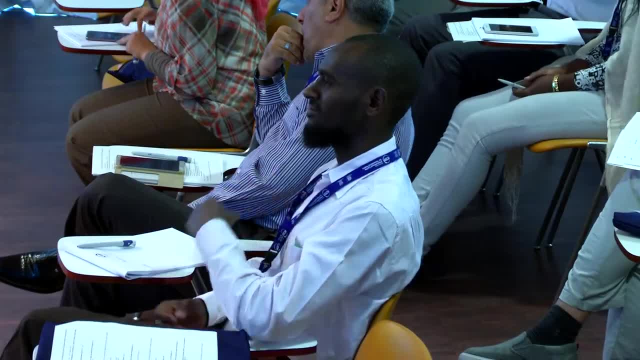 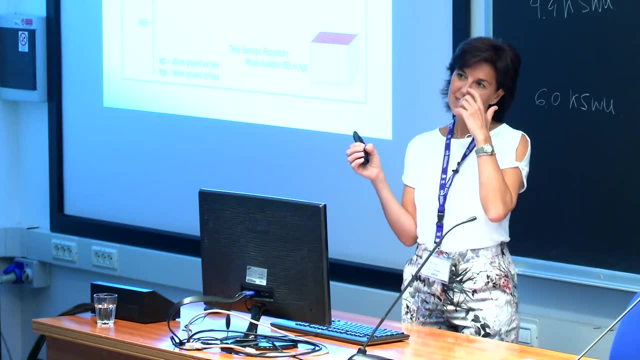 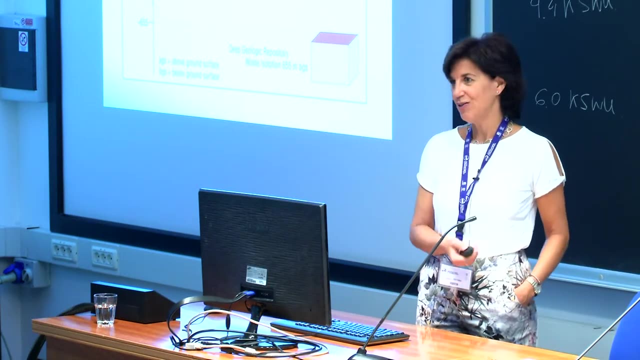 know, by my common sense it should be the same, but I'm not sure. but for example, in the case of the deep geological repository, because the nuclear power plants is licensed by 40 years of lifetime, but in the case of the deep geological repository it will last for a long time, so maybe it shouldn't be. 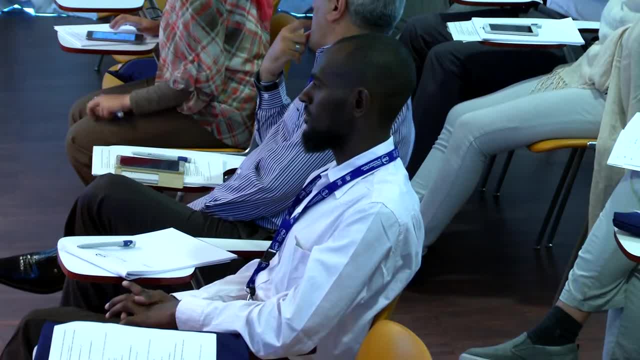 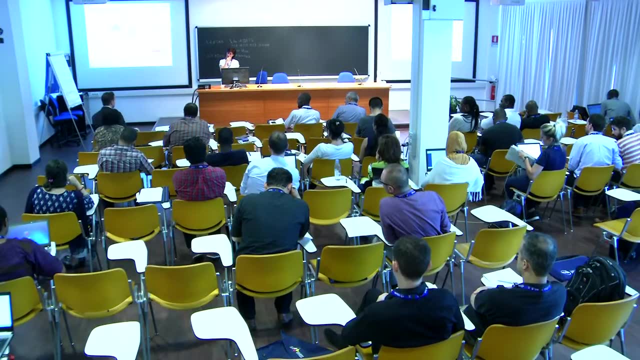 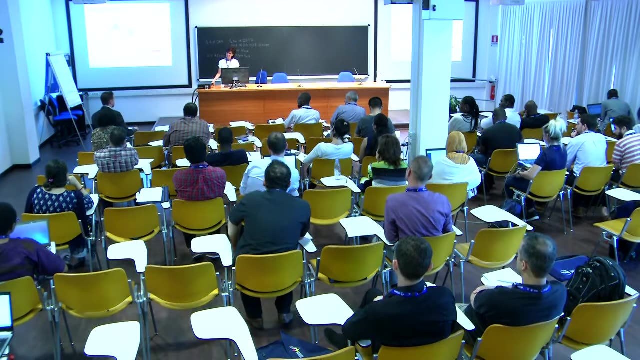 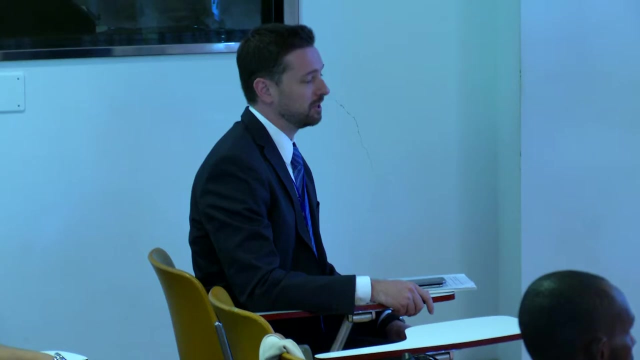 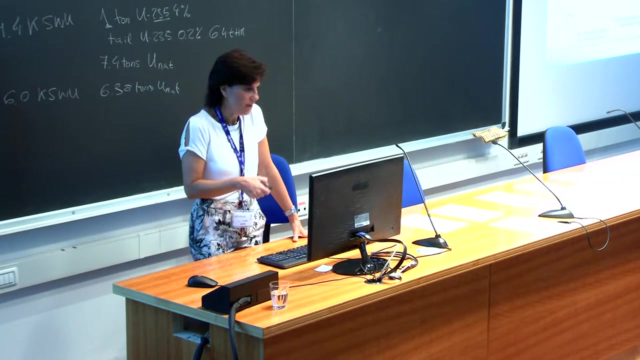 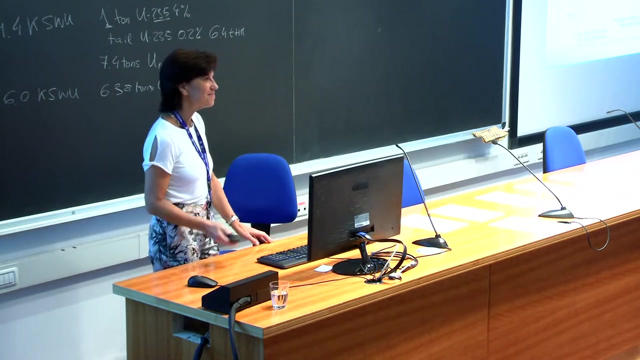 the same. maybe it should be more restrict in this case, but I don't know, yeah, because the nuclear industry is is always very, very safe, But maybe it's much more in the case of the geological repository. I don't know, Borhol. 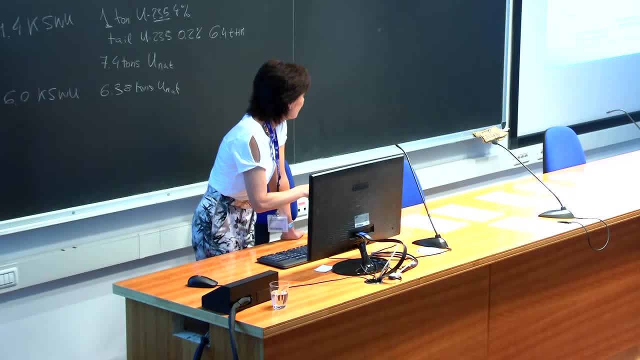 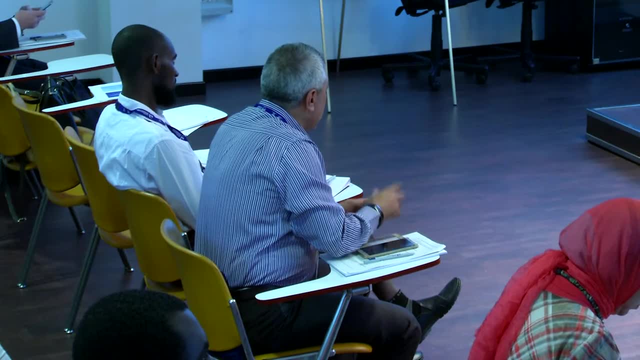 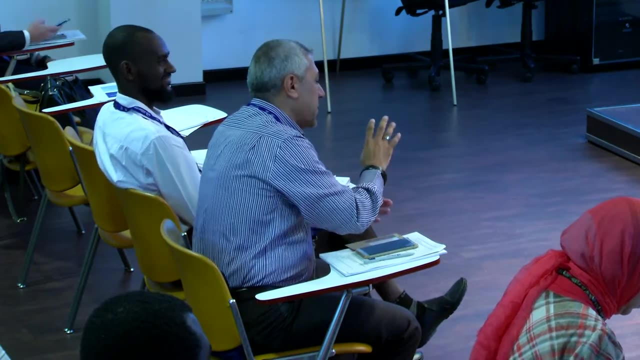 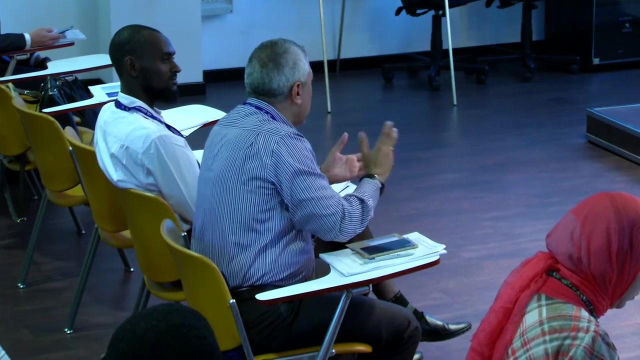 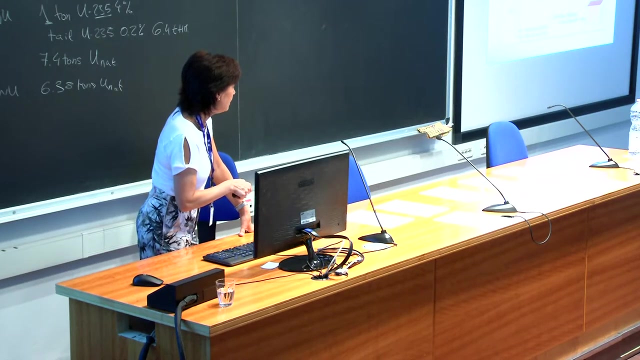 Borhol, Yeah, Yeah, in principle it's mainly dedicated to the source sources. Yeah, Yeah, But the source sources is a radioactive waste also. No, I think so far, the current options are dedicated to the source sources. 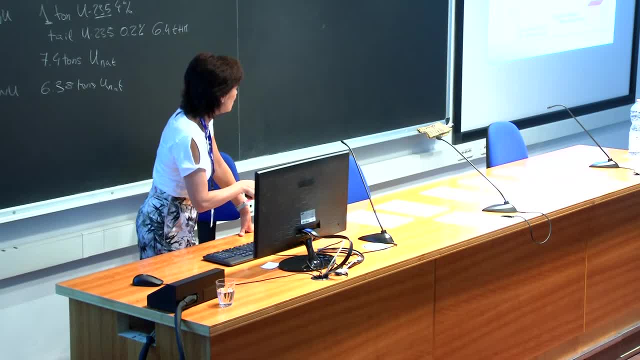 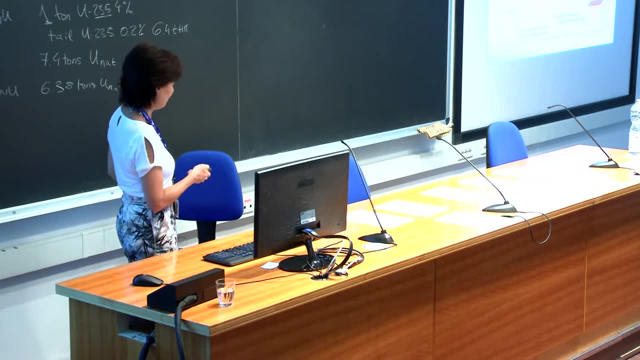 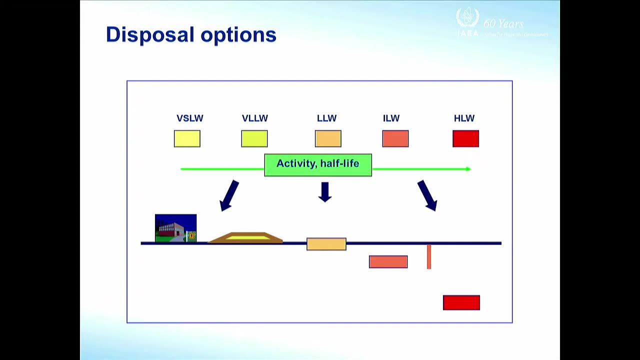 I guess more than intermediate. but in this slide it's considered all radioactive waste, not only those coming from the nuclear power plant. So this is a graph facing the different options with the different levels of classification of the radioactive waste. So we see the very low short-leaf and very low 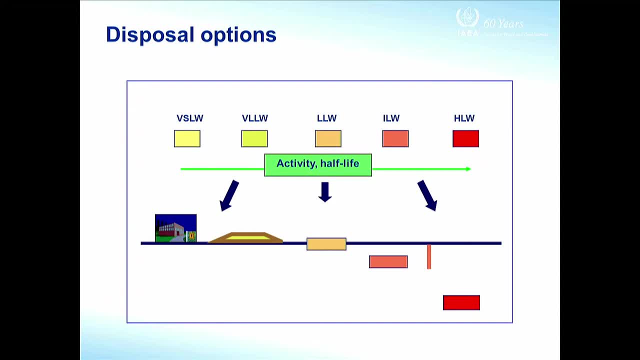 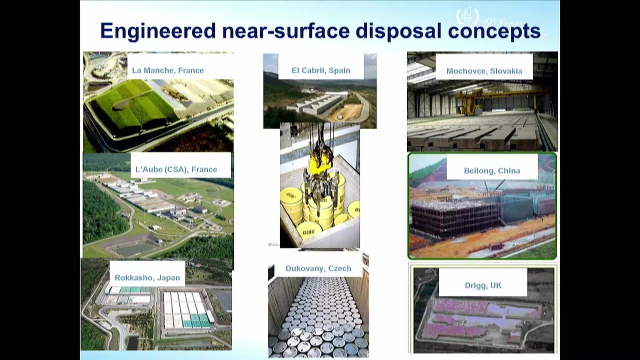 its surface low level some meters below or over the ground, the intermediate deep and the high-level waste very deep. So this is some examples of engineered near-surface disposal concepts And, for example, you can see here this is: 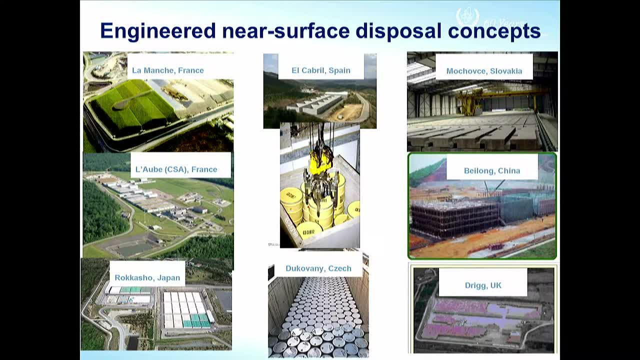 a covered And you can see the concrete structure. The cells are made of concrete And if we asked to fill these cells, anything is the same, like here, with drums in a square, cells filled with concrete, and then these fill all these cells with concrete and cover them and at the end the remediation is made with. 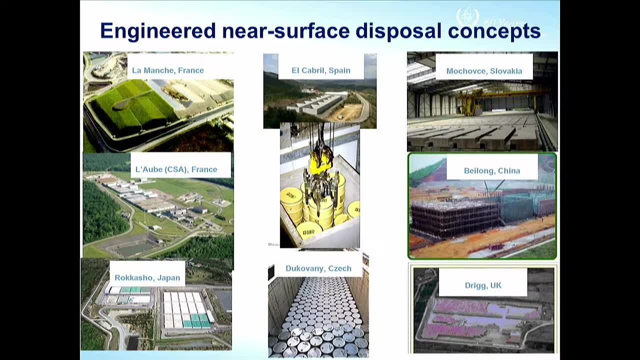 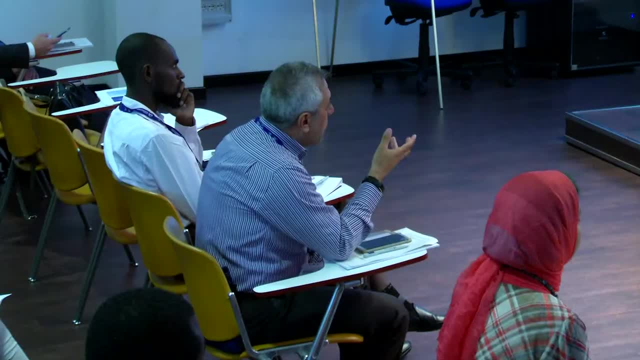 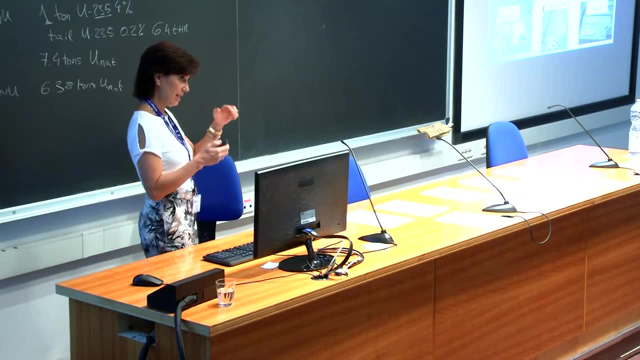 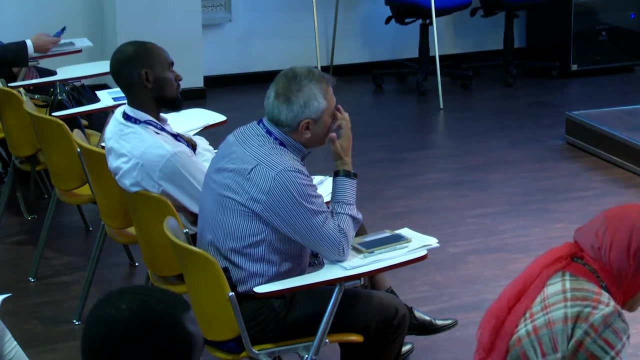 vegetation? I don't think so. I don't think the concrete, the formulation of the concrete, to be put in as a matrix. it's, it's supposed a facility. it's supposed to a facility, yeah, for low level waste, and the concrete is used as a matrix to immobilize the low level waste. 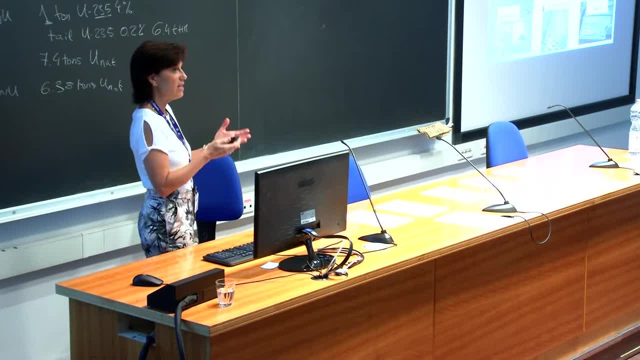 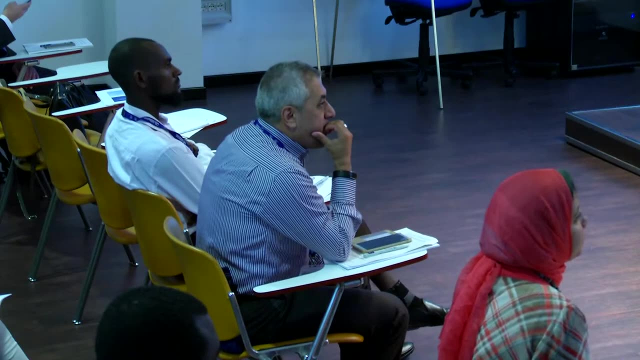 and the formulation of the concrete I think is licensed to last the whole period and to avoid the leaching of the radioactivity, and it's used as a matrix. it's a conventional matrix for low level waste and this is the other option is when it's a few meters below. 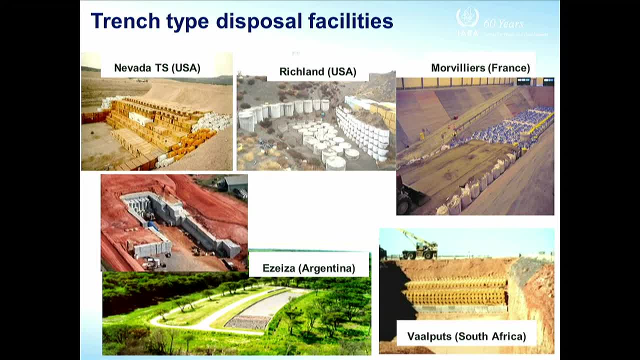 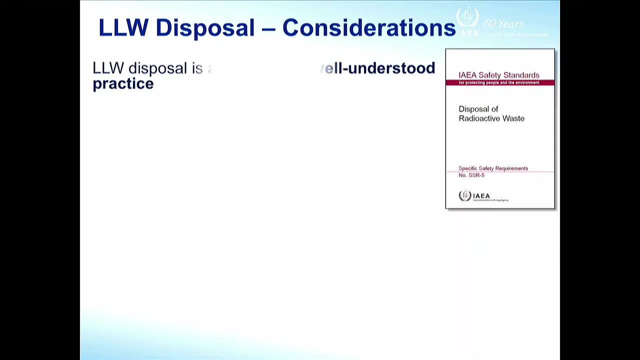 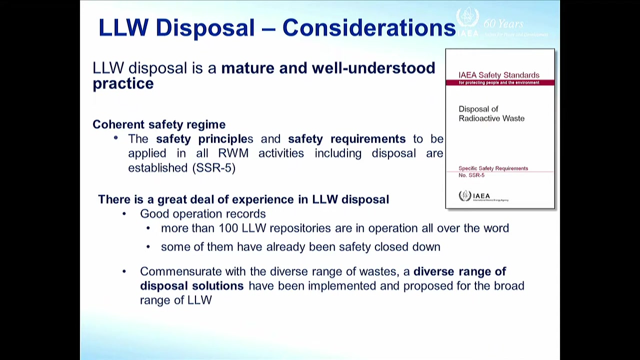 the ground floor is the trench type disposal, and you can see different examples in the United States, in France and in Argentina, for example- and it's dedicated to low level waste. so so far, the low level waste disposal is a mature and well understood practice and the requirements are. 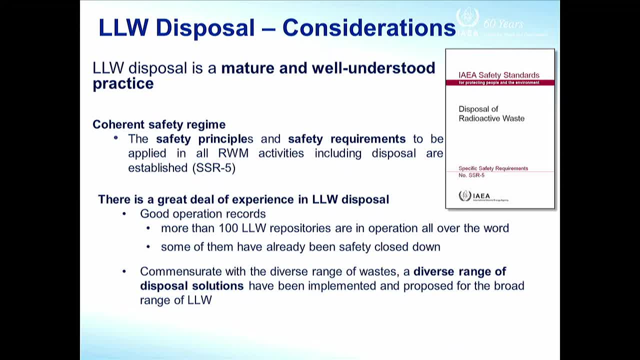 you can find the requirements in this safety guide. it's SSR 5 about the disposal of the radioactive waste, and so there are more than 100 low level waste repositories working so far in the world. so there is a lot of lessons learned and operational experience gathered, and this 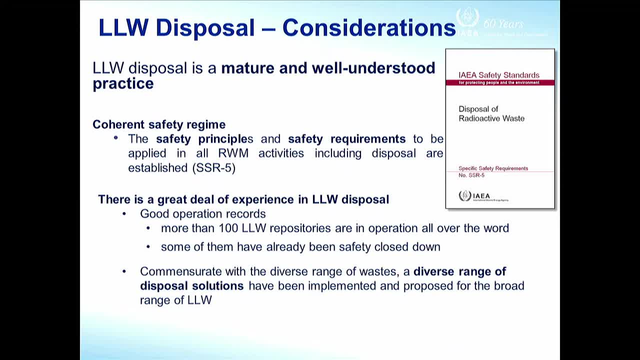 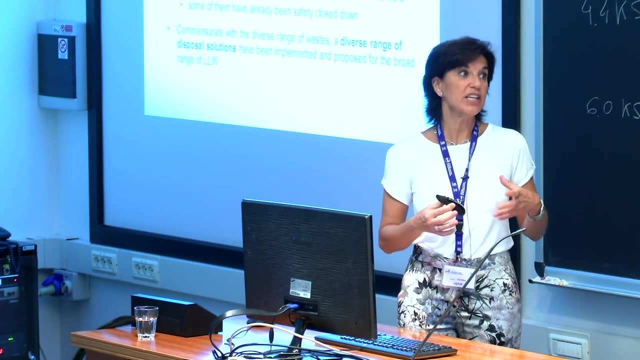 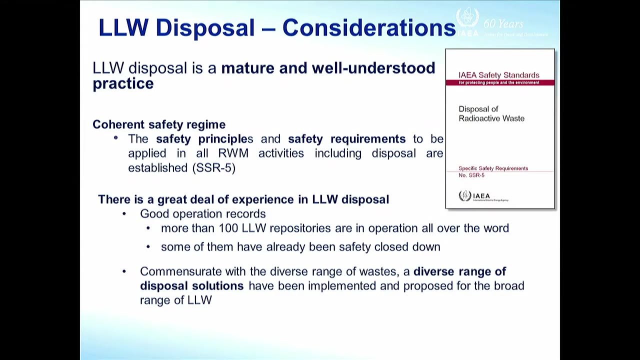 and this is the, the are different range of disposal solutions and since there are different types of radioactive waste produced in a different operations with applications of the nuclear energy, and this, these experiences gathered, are very useful for the newcomer countries of the people of the countries we started working with the applications of nuclear energy, not only with the nuclear energy. 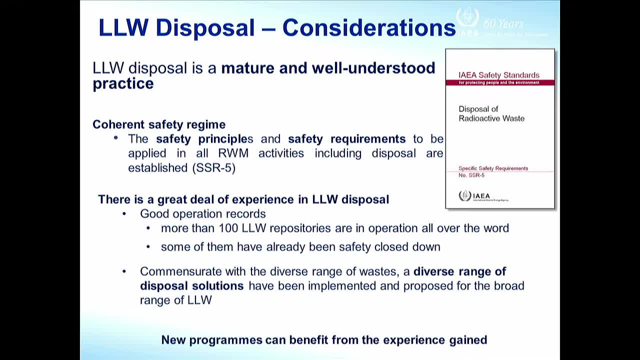 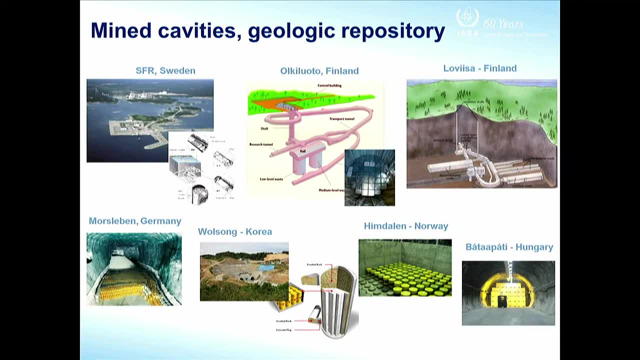 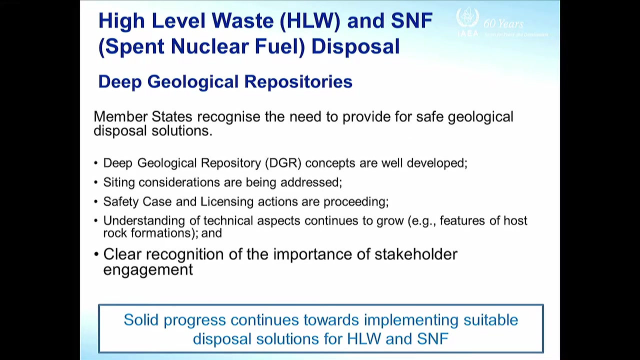 production. so the inc is always fostering the change, the sharing of lessons learned and the operational experiences. and this is options for the mine cavities is when the intermediate level ways are disposed of deeper and below the ground. and these are the examples of the different options of the geologic repository and we talked about them during the last talk. so the option for high 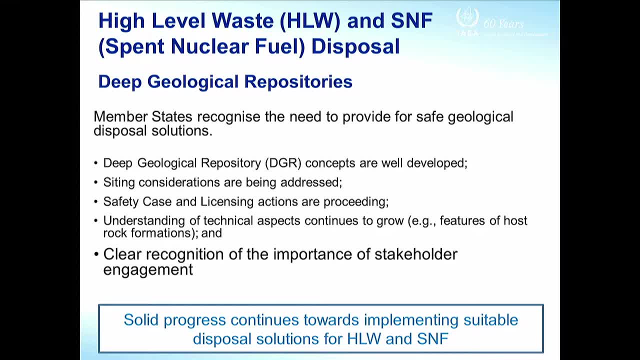 level ways. that we mentioned is the deep geological repository, and the most important thing is now, after experience, is there is a clear recognition that the importance of the stakeholder engagement- and now there's a lot of effort put in engage and find the ways and the tools to engage this. 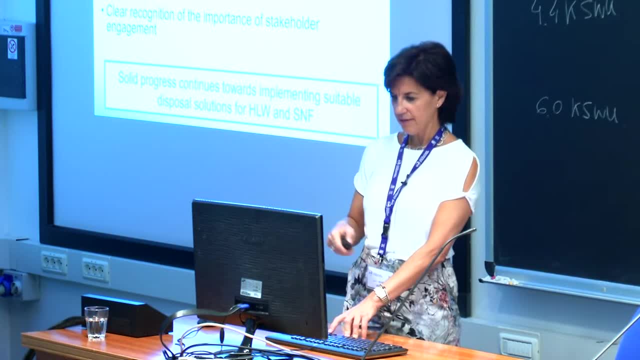 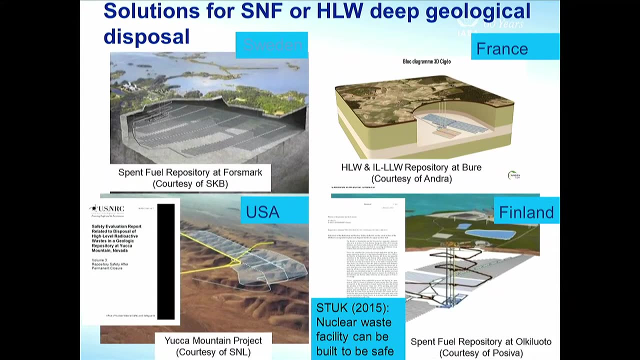 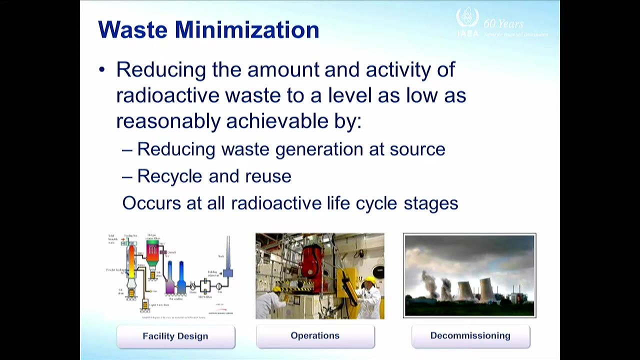 stakeholder from the beginning of the disposal facility and the decision and the siting process. so we talk about this- i'm not going to repeat that- and one of the most important things, to minimize the waste of the part, the volume and also the radioactive content, and it's made reducing the 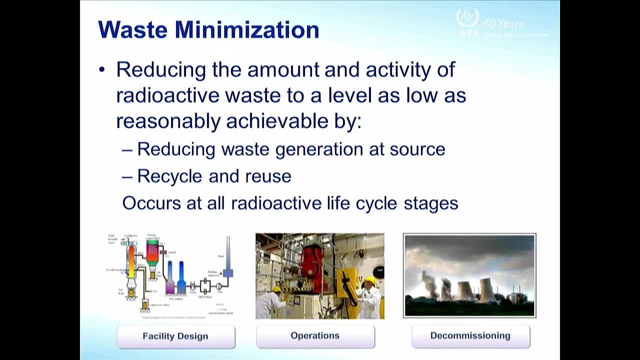 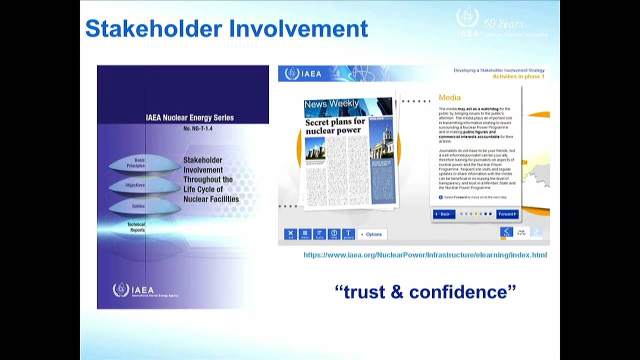 generation at source and recycling and reducing the material, and it should be made in all the stages of the nuclear energy cycle, so since the facility designed through the operation and during the decommissioning of the nuclear power plant. so, as i mentioned, there is a lot of effort now put in a stakeholder involvement and there are a lot. 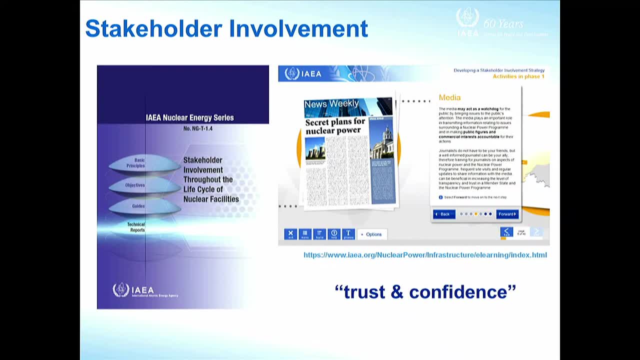 of activities performed by the imc and also in collaboration with another international organizations as the oecd, nea and the european commission. because it's important to build trust and confidence of the public in the nuclear industry and the nuclear applications. because many people go to the hospital. 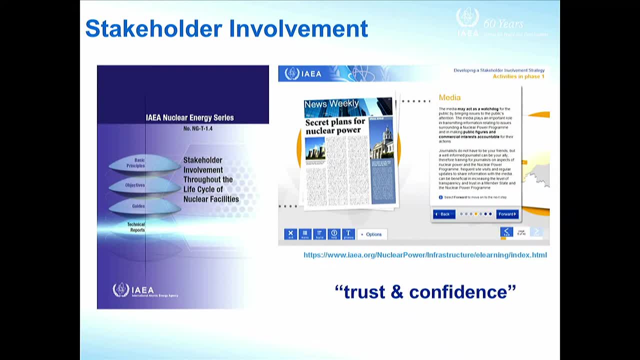 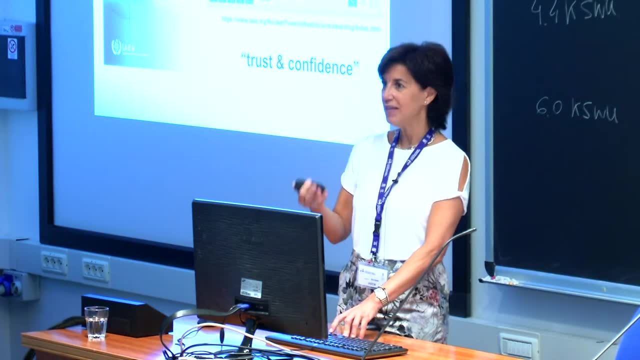 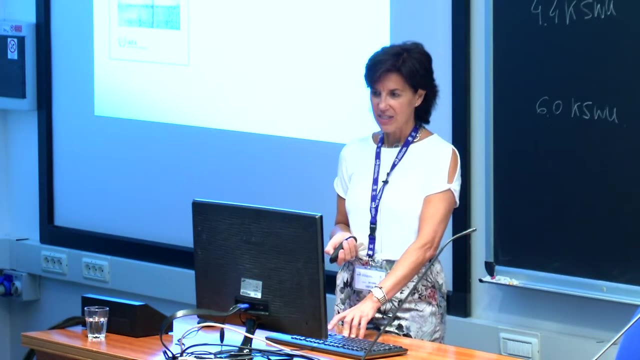 and they don't know that they are treated by nuclear material and they don't know. so i think there is a lack of communication to the public in general, public about the benefits and what they are receiving from the nuclear applications and the nuclear industry. so let's talk about the 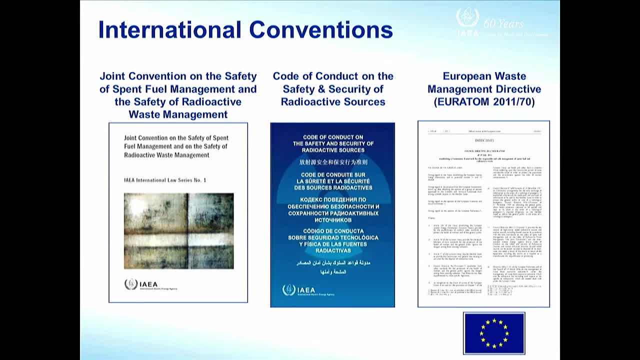 international conventions. so, since the countries are not working now isolated, so there's a lot of international relations and there is a directive issued by the euraton in the european commission in 2011 about giving a guide and advice to the countries on how to manage radioactive waste and spend fuel to harmonize the practices. 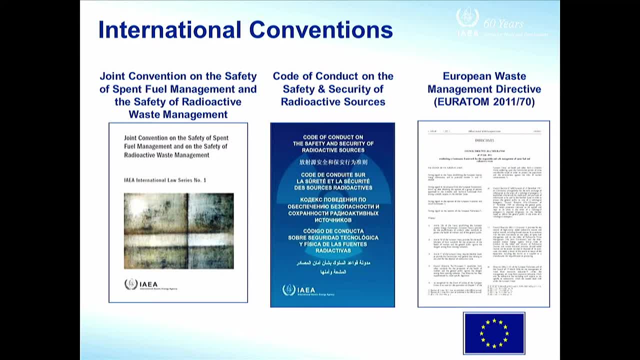 and also there is a code of conduct on the safety and security of the reactive sources, and now this is the joint convention on the safety of the spent fuel management and radioactive waste management, and i'm going to talk about a little bit about it and the john. 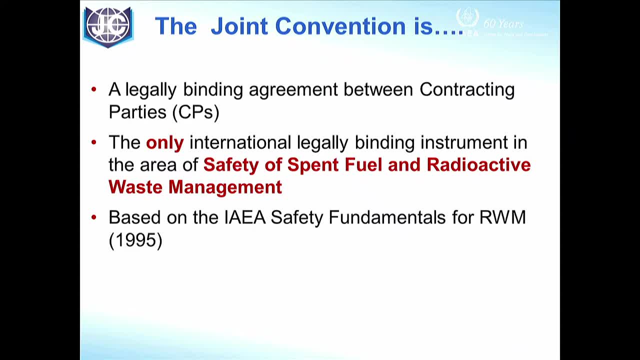 convention is a legally binding agreement between contracting parties, so the countries are free to sign the contract, but the inc is fostering and try to encourage the countries to sign the contact to be part of the joint convention. It's the only international legally binding instrument in the area of safety and security of spent fuel and radioactive waste management. 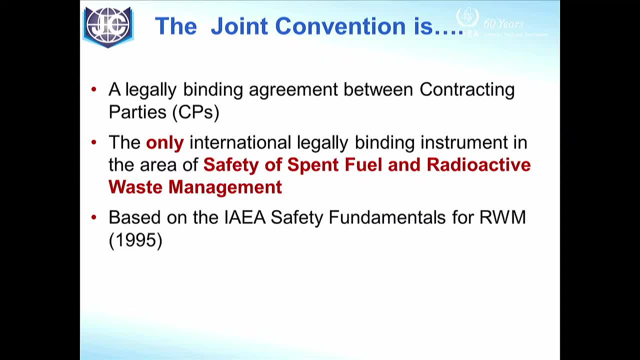 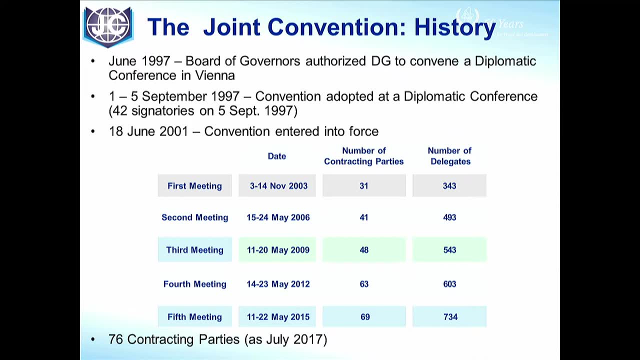 and is based on the safety fundamentals of radioactive waste management. So this is the story. In June 1997, the Board of Governors authorized the DG to convene a diplomatic conference and in September of this year the joint convention was signed by 42 member states. 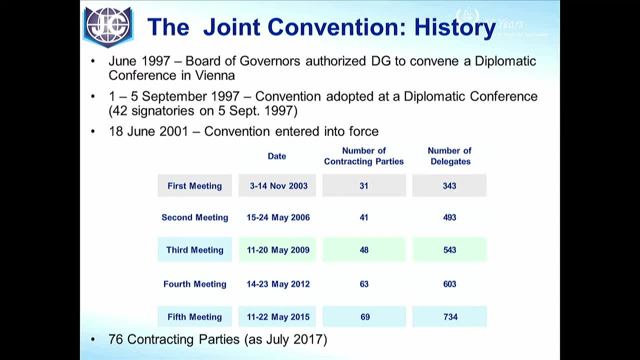 and entered into force in 2001.. So every three years there is a meeting, and the last one was in May 2015, and the next one will be in May 2018, so next year, And so far there are 76 contracting. 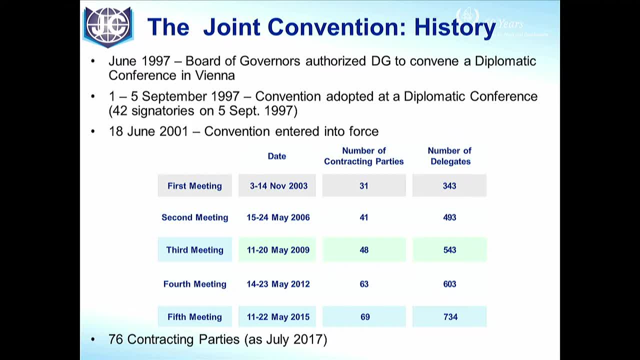 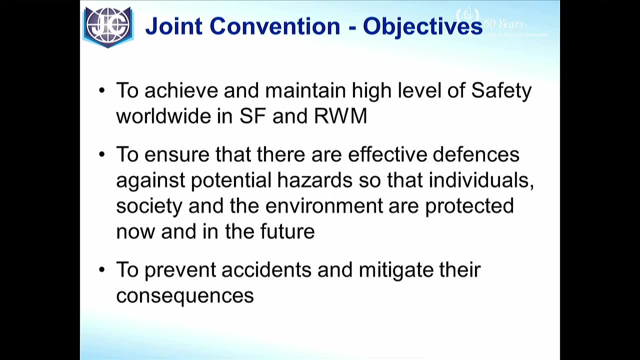 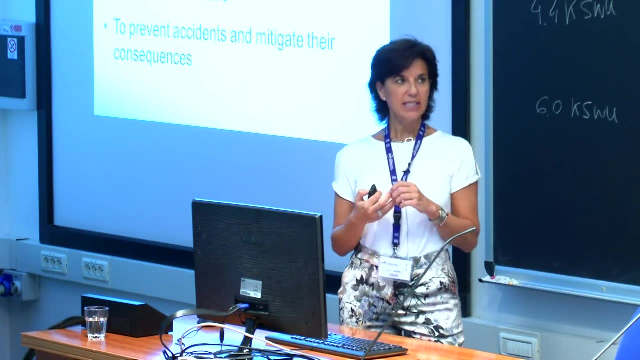 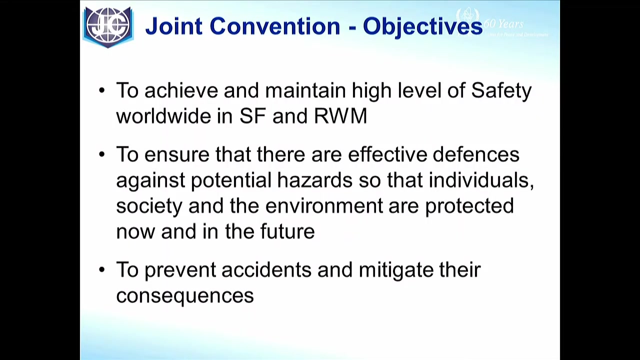 parties. So what is the objectives of the joint convention? It's to achieve and maintain high level of safety worldwide and to ensure that there are effective defenses against potential hazards to the individuals and to the environment. And also the idea is to prevent accidents and mitigate. 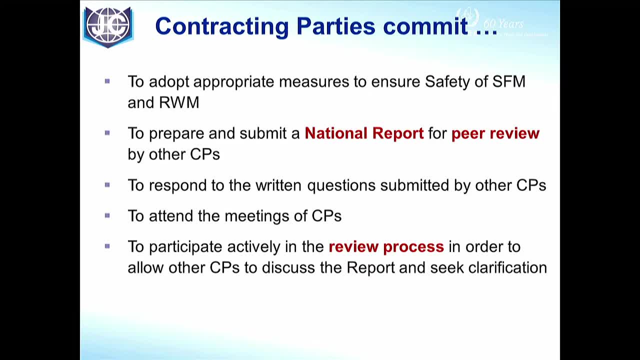 their consequences. So when a country sign as contracting party, they commit to adopt their appropriate measures to ensure the safety of the spend fuel and radioactive waste management. They commit to prepare, submit a national report for the peer review of the other contracting parties. They commit to 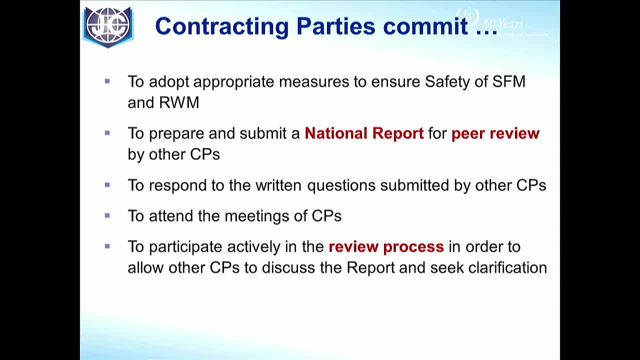 respond in written to the questions addressed, And so this is one of the proposals from the board third week of July 2019.. Great, Yes, thanksumbers, Thank you. Great Thank you. submitted by other contracting parties to attend the meetings every three years. 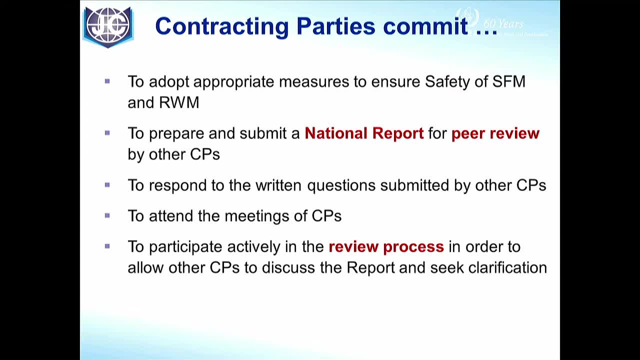 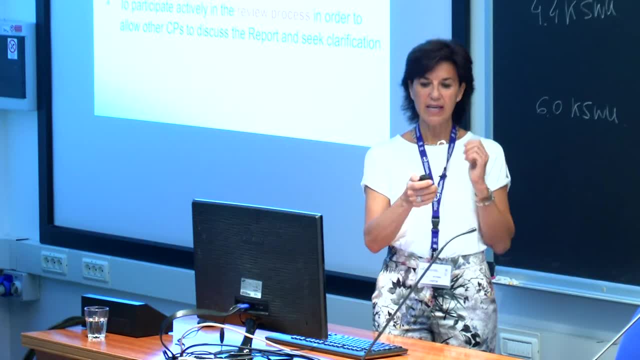 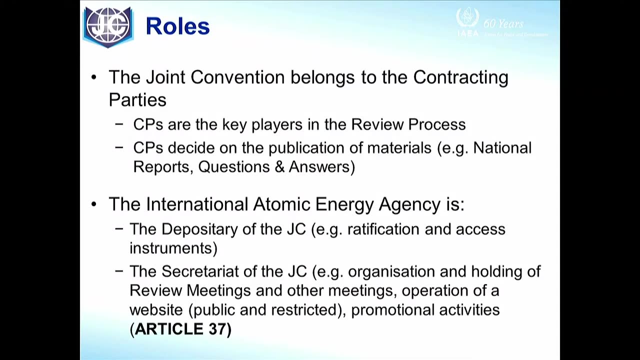 and also to commit to participate actively in the review process. so the strategy, the policies and a strategy of every contracting parties are peer review by the other contracting parties. so in this case the agency only act as a secretariat. so we are the depositary. we sorry, we are in charge to organize the 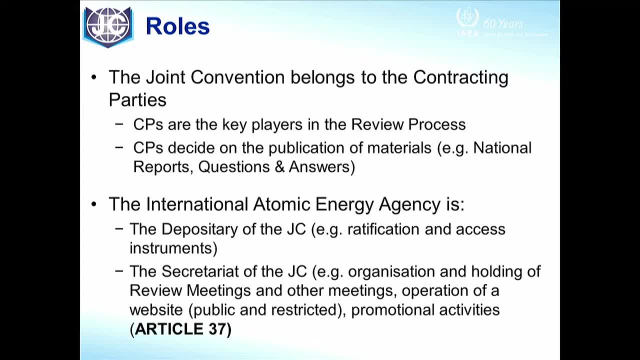 meetings, to hold the meetings, to maintain the website with the information and also to make promotional activities, to ask, to promote and to make other countries to sign as contracting parties. and, for example, the last two years. the last two years we got six new, so where were 70 contracted parties by 2015 and now we? 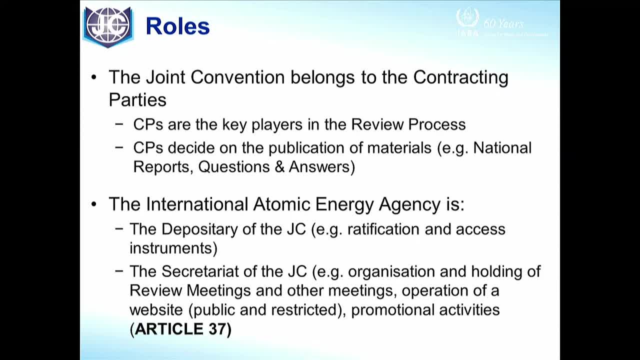 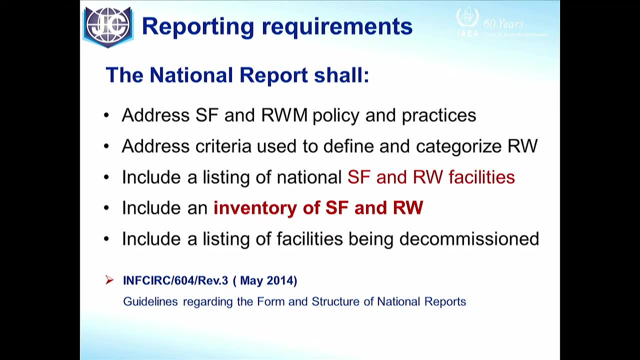 are 76, so in two years we get six more contracted parties. and the joint convention belongs to the countries themselves, so they have to submit a national report that shall contain the policy and practices for spent fuel and radioactive waste management, to address the criteria to categorize the 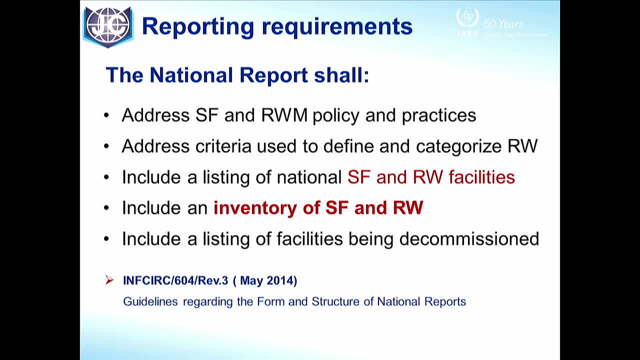 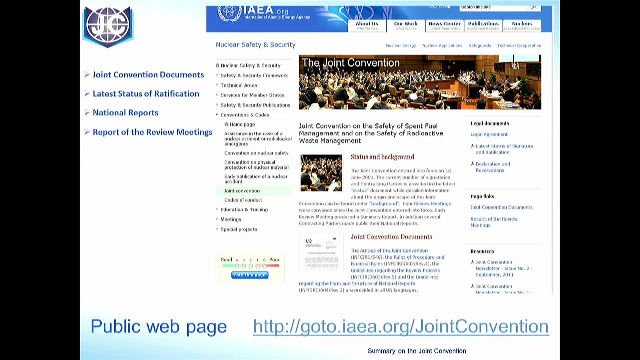 radioactive waste and they have to include a listing of facilities and the inventory of a spent fuel and radioactive waste and they have a web page you can find in this link with. and they decided which information they would like to make public to the public or they also decided 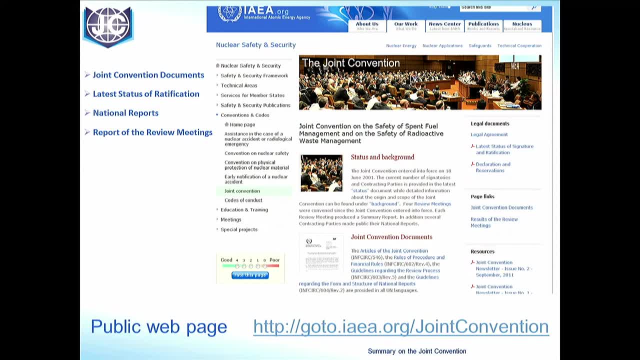 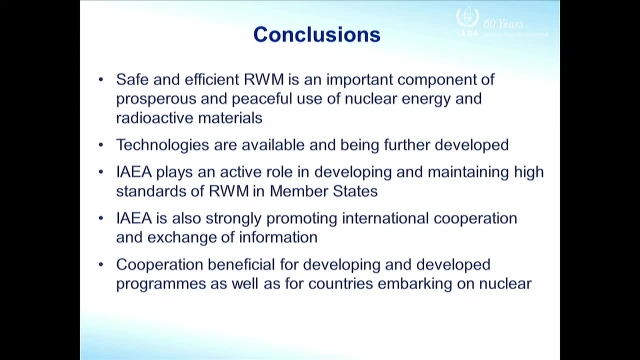 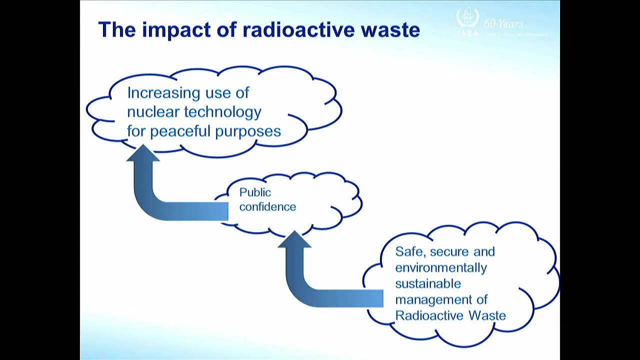 which information they would like to make public to the public, or which information ran content. let me see how to. or they keep reserved by themselves. so I think I'm going to go quickly to the decommissioning part. so only as a conclusion, if the radioactive waste are. 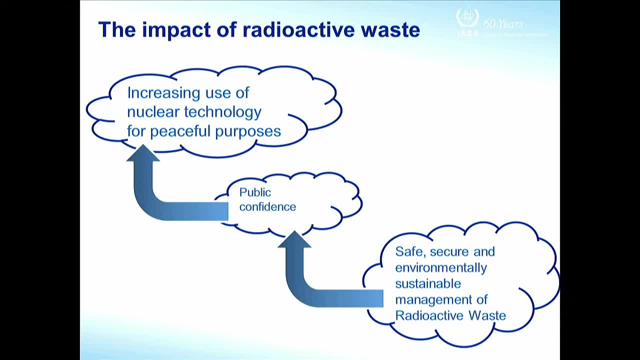 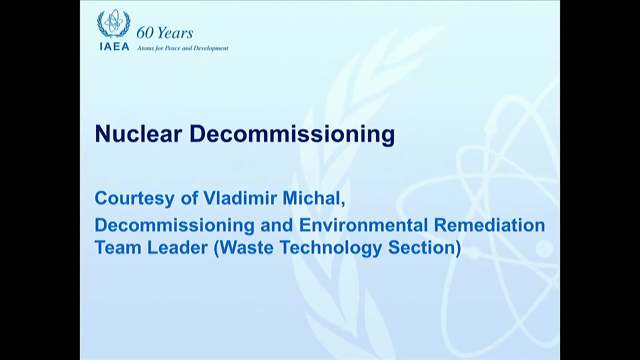 managed safely, securely and environmentally. I we would like to have more public confidence in the nuclear industry. that increase the acceptability of the nuclear energy and the nuclear applications. so now let's move to the decommissioning part of the talk. I will try to be as fast as I can, so 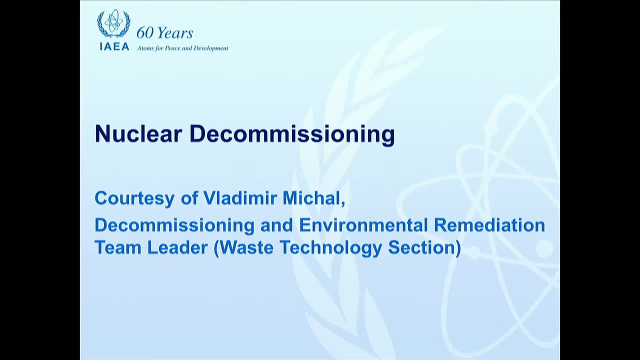 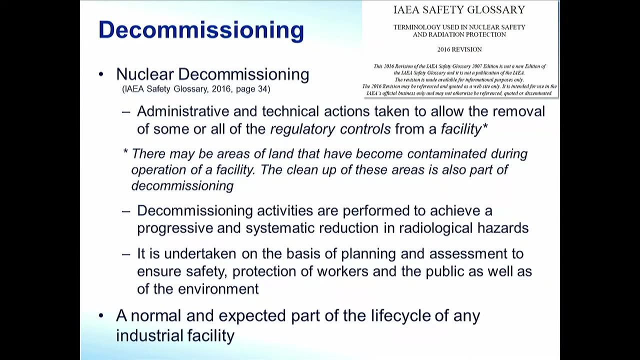 this presentation is a courtesy of my colleague, Vladimir Michal, who is the technical lead of decommissioning in the waste technology section and environmental remediation. so, looking to the glossary, the safety glossary nuclear decommissioning is the administrative and technical actions taken to allow the removal of some or 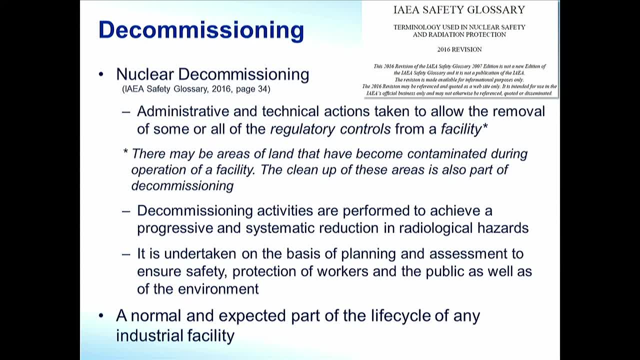 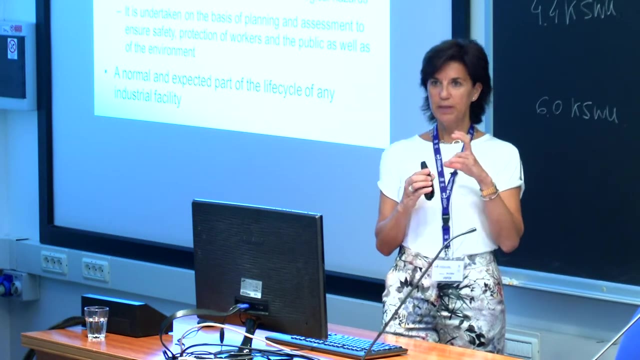 all of the regulatory controls from a facility, but not only from a facility, because there may be areas of land that have become contaminated during operation of a facility and the cleanup of these areas is also part of the decommissioning, so the commissioning activities have to be performed to. 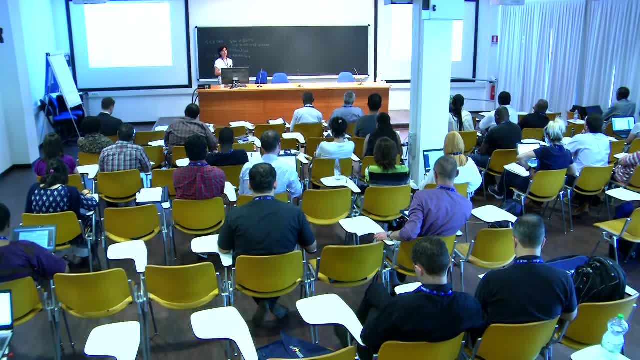 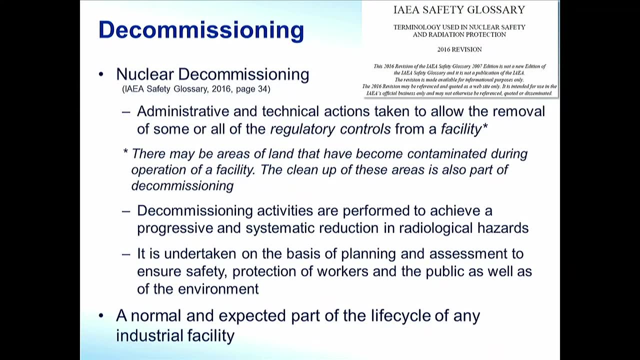 achieve a progressive and systematic reduction of the radiological hazard, and it's undertaking, on the basis of very rigorous planning and assessment, to ensure the safety protection of a resource for the ecosystem. these activities should not be continuously knew with obstacles when providing earrings and equipment for those of nature. 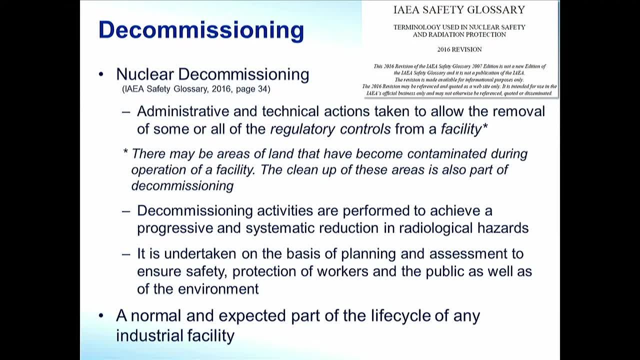 have to be accomp sandbox business with whoever is committed as a consumer in this business: protection of workers and the public and the environment as well. so, and it should be taken into consideration as a normal and expected part of the lifecycle of any industrial facility. so, as we will see that the commissioning should be, 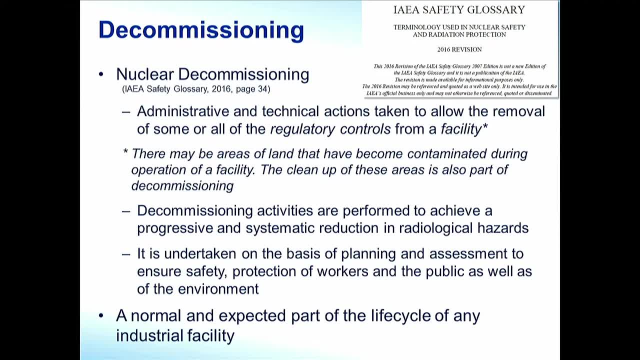 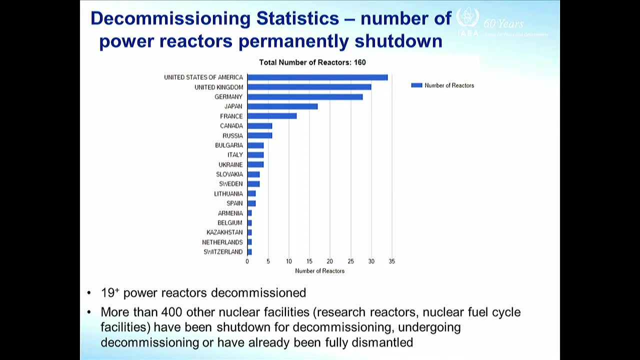 keep in mind from the beginning of the design of the facility, because if we have to dismantling a facility- and it was taken into account at the time of the design of the design- it should be easy. so this is the situation, the current situation. so there are more than 19 power reactors. the Commission so far. 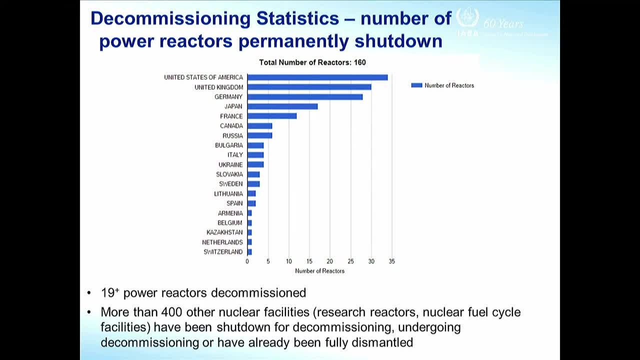 and there are more than 400 other facilities, including research reactors or research and development facilities, universities and nuclear fuel cycle facilities that have been shut down for the commissioning and undergoing the commissioning or have been the Commission. so there is a lot of knowledge and experience on the 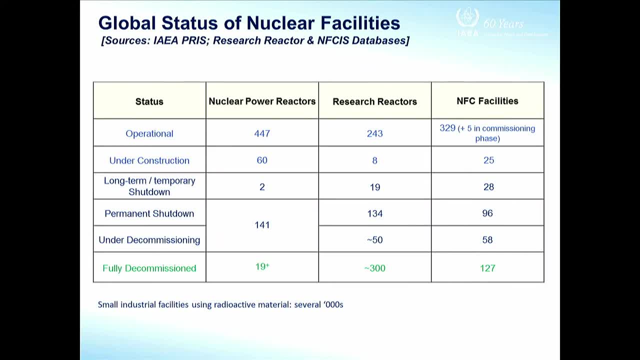 Commission so far. so these are some numbers that you can get. if you type PRIX is the INC power reactor infrastructure system information system, thank you. and if you can type, if you type google, EIA, PRIX, you can get the link. and also we have a database on reactor and nuclear. 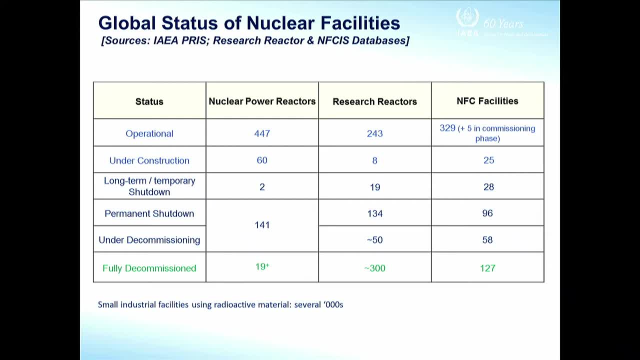 fuel cycle information system, also for nuclear fuel cycle facilities, and you can find this type of numbers of the nuclear reactors in operation which are launched in temporary shutdown or in permanent shutdowns and so on. so that's it for today. thank you so much for your attention and we will see you next time. 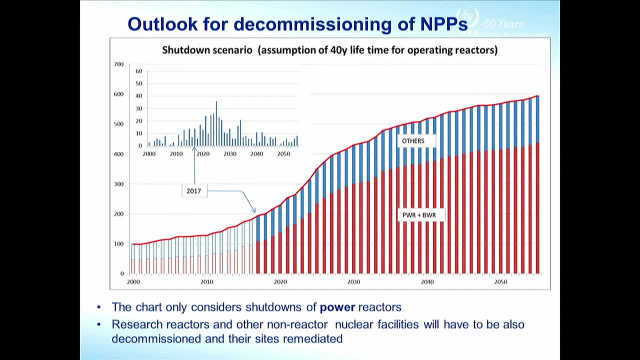 this is the outlook of the Commission in for nuclear power plants, and so it's for seen growing in the commissioning of the power reactors and this is the scenario for the shutdown. so in 2020- something most of the plans that were built on constructing the 80s will reach the end of the life of nuclear power plants. 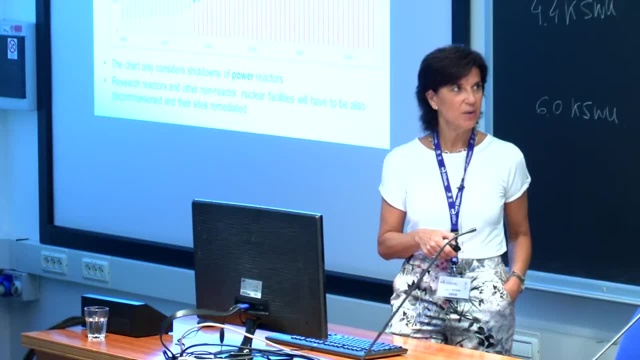 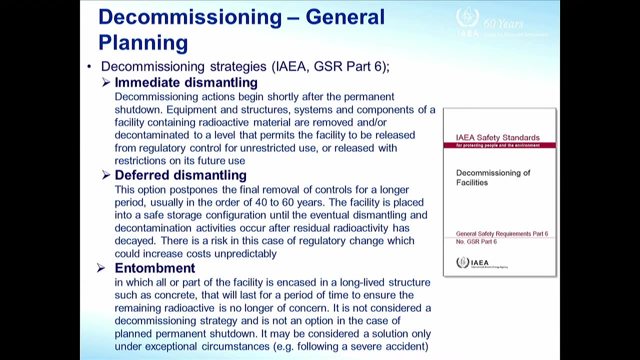 so they will be shut down and they will go under the commissioning. so, as it's mentioned in the general safety requirements, in the part 6 on the commissioning of facilities you can find the this three the commissioning strategies. one is the immediate dismantling. 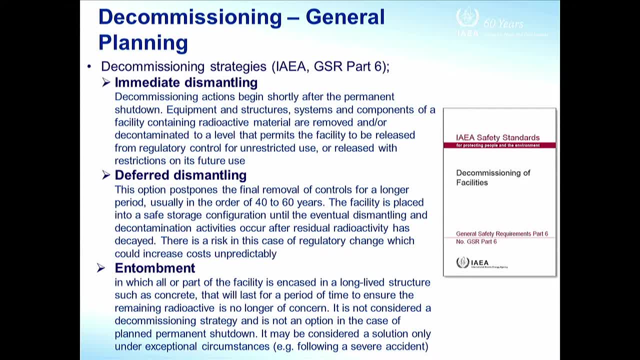 it means that the commissioning actions begin shortly after the permalint shutdown and everything is removed and they land is clear for other purposes. but there is another option, that is, a deferred dismantling and when it's considered that after shutdown the country weight or the operator weight 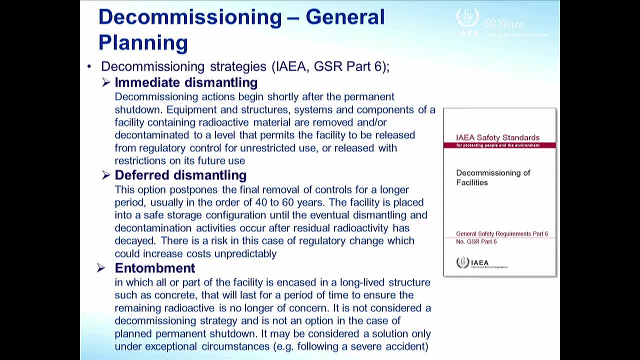 until 40, 60 years before starting the dismantling of this power plant, theức, the facility In this case. they use this time to allow the short-lived radionuclide to decay, and then the radioactivity to be managed is lower and the decay heat is lower. So this is the strategy that the country can choose. but in the case of the referred dismantling, since they wait 40, 60 years, it could be a lot of changes in the requirements and in the safety and in the government. So it's very dangerous and that maybe can cost a higher. 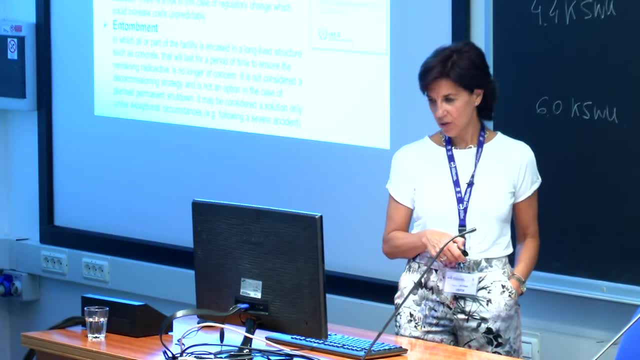 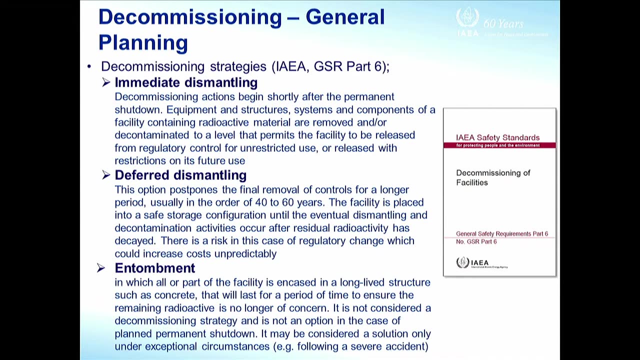 cost at the end. And the third option is the so-called entrapment, and it's a combination of the two other options. So on one hand, some parts of the facilities are dismantling at the commission and another part are kept in the government. 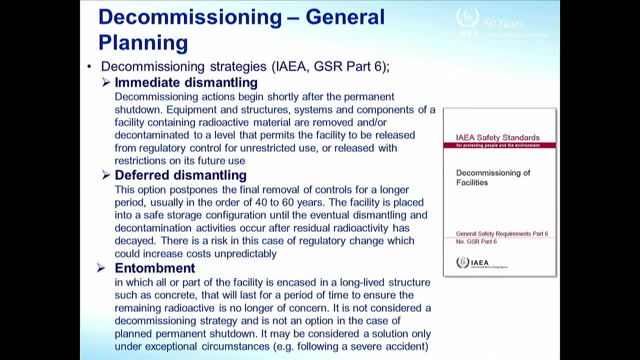 In safe mode, so are conditioned in order to avoid the radioactivity release. But this condition, this option, is not considered as the commissioning strategy and it's not an option in a normal shutdown and the commissioning is only considered in the case of normal circumstances. 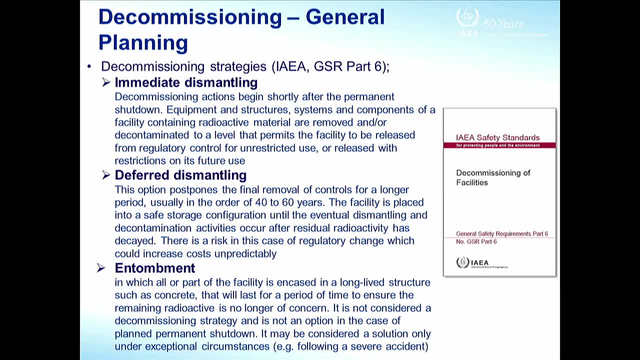 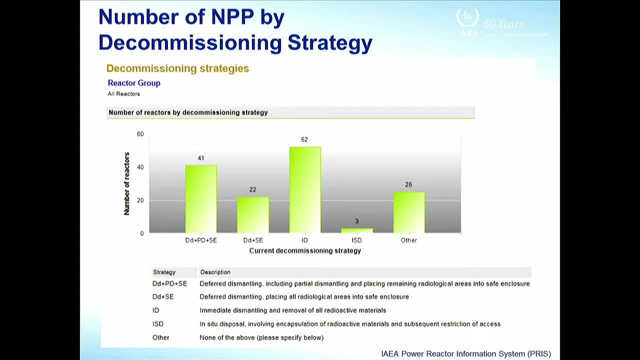 as a severe accident Or as we will see in the case of the reactors using graphite. it has decided to go through this option and I will explain later. So these are some numbers of the nuclear power plants so far. So they are around 50 that go, or plans to go, under deferred dismantling. They are 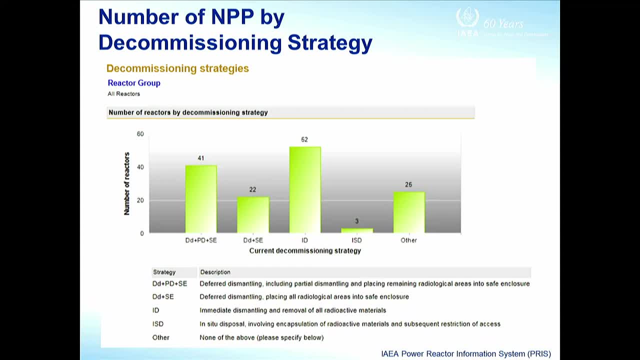 around another 50 that plans to go under immediate dismantling. And there is these three entombed, so the radioactive material has been conditioned in situ. so the land has to be restricted access and restricted use. And there are another around 25 without any decision taken so far. 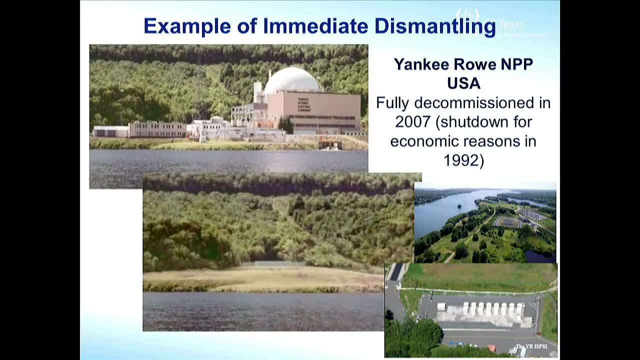 So this is, for example. this is an example of one nuclear power plant under immediate dismantling. So it is the Yankee Road nuclear power plant in the United States and it was fully decommissioned in 2007 and the shutdown was in 1992.. And you can see the land with 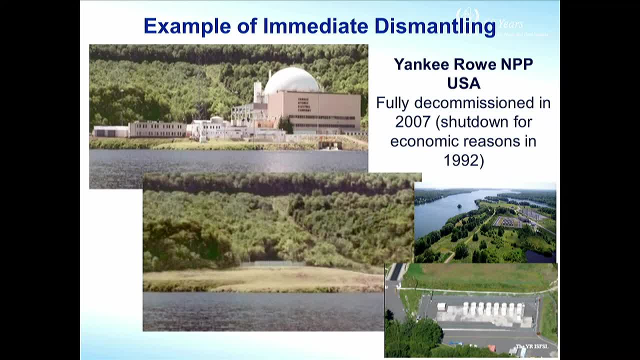 the nuclear power plant, the land up there with the completely commissioned site, But the spent fuel remained in the site. so now it is a problem that, for example, in the case of United States, they are facing the cost. Most of the plants are reaching the end of. 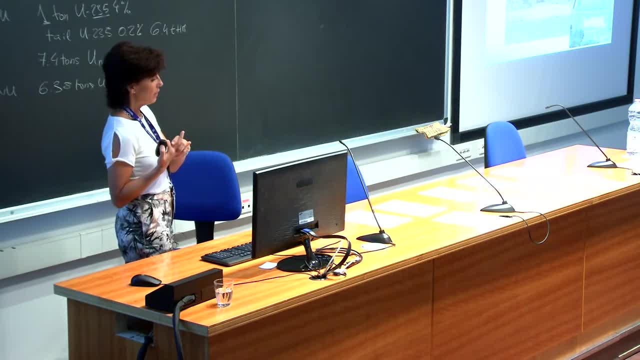 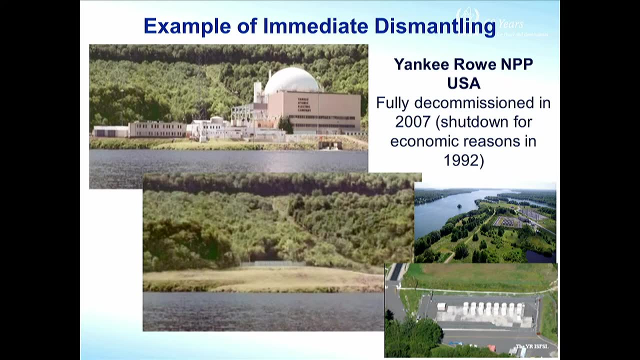 the light time or they are shutting down due to economical reasons And the storage remained on site And at the time the nuclear power plant is in a poor condition And the cage that is fully staffed but should remain staffed- that take care about the storage facility. 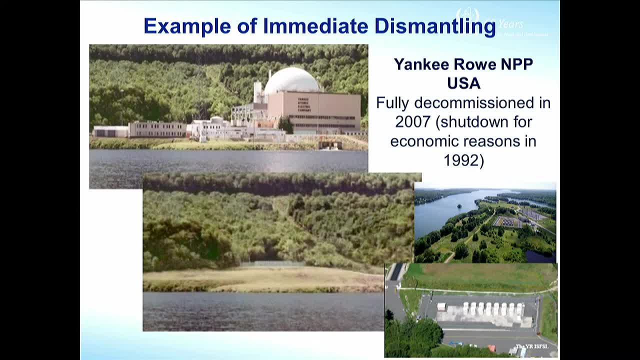 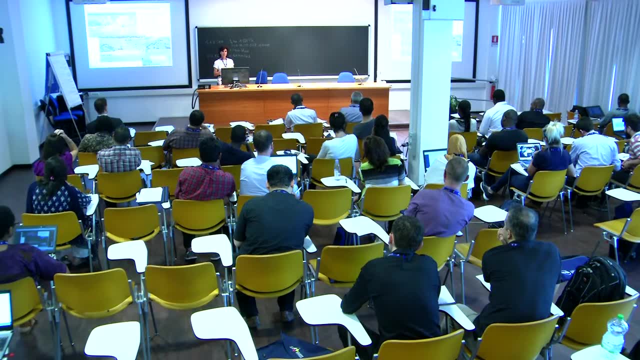 So it's an issue that now countries are facing: how to deal with different interim storage sprouts. all over the countries And also in Spain, we have the same problems. We are building interim storage because we don't have any centralized interim solution. We are building interim storage in three, four of our nuclear power plants. 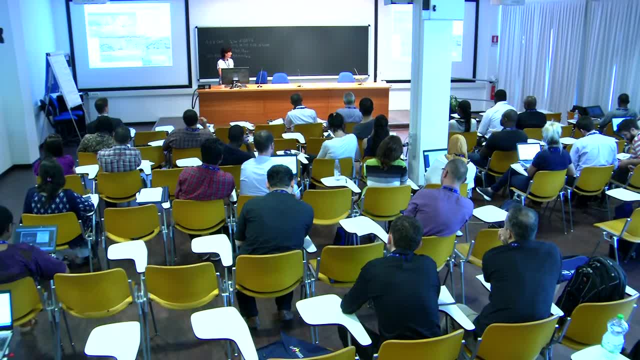 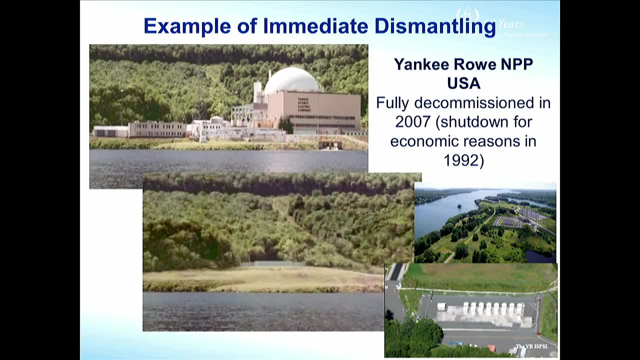 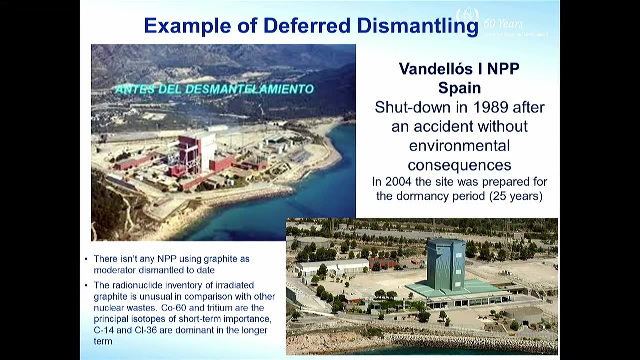 And at the end of the lifetime, when the nuclear power plant will be decommissioned, the storage will remain alone there, And this is an example of deferred dismantling. So it's an example of the nuclear power plant of graphite gas. This was one. It was shut down in 89 after an accident, without any environmental consequences. 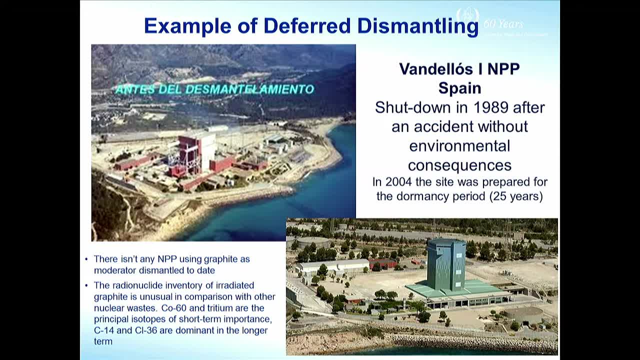 but the operator decided to shut down the plant, And so this was the plant, And then, after the demolition and dismantling, the graphite is kept. So the spent fuel was sent to France For reprocessing, But the graphite is very difficult to manage. 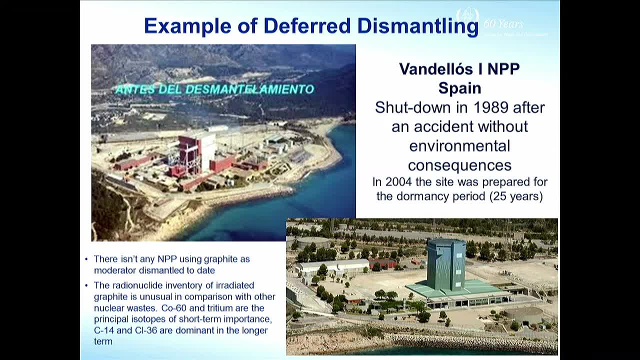 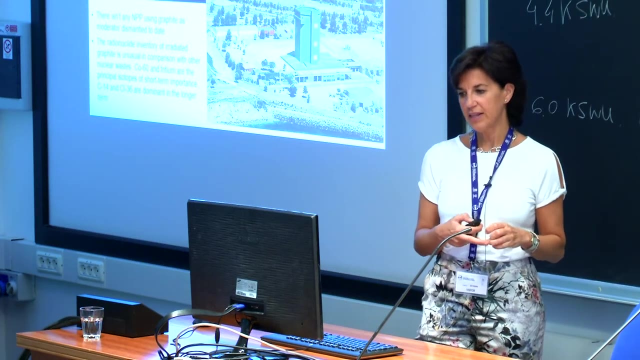 And was kept for a dormancy period of 25 years That will be finished in 2028.. Yes, because it was started in 24 for 25 years, To allow the majority of the activity to decay. Because the graphite, the radionuclide inventory of the radiated graphite is unusual. 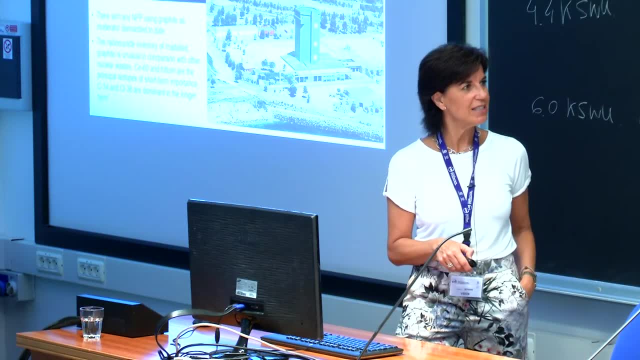 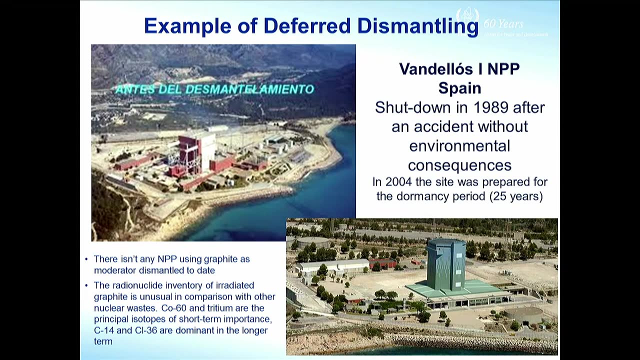 in comparison with another nuclear waste. So there's a lot of cobalt-16 that has a half-life of five years And there's tritium, A huge amount of tritium, And it's one order of magnitude of the concentration of carbon-40.. 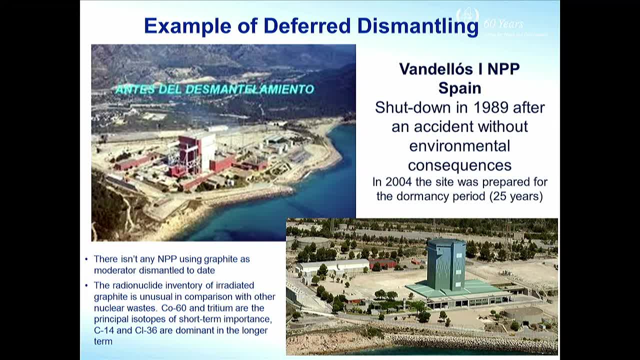 And it's also chlorine-36. that is a long term because it's a radionuclide, It's a beta emitter with a long term And it has a half-life. So now there is a project run by the agency in order to harmonize and to find solutions. 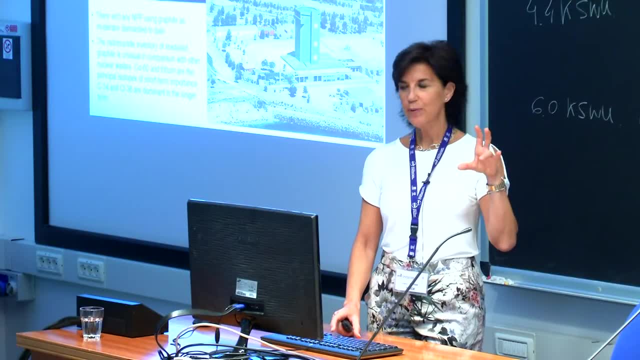 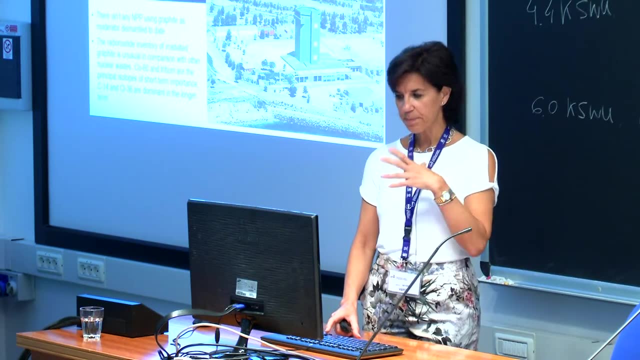 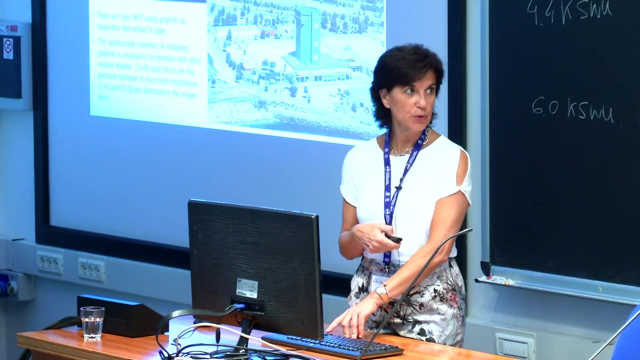 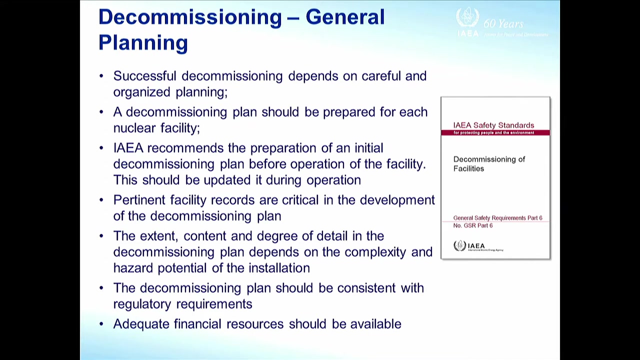 among all countries that have nuclear power plants with irradiated graphite to gather practices and to discuss and to find harmonized solutions among countries to manage the radiated graphite. So the decommissioning has to go under a very strict plan. So the success of the decommissioning depends on the 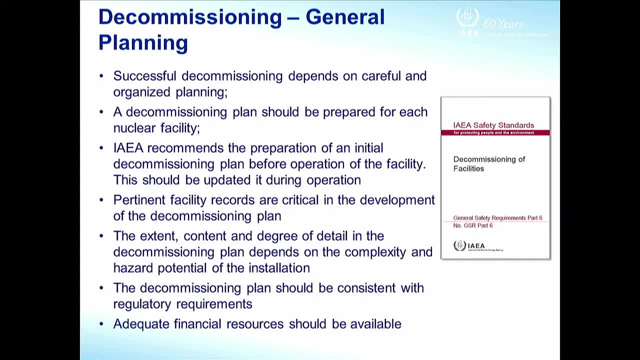 carefully organized plan and should be prepared for any nuclear facility. So the agency recommends to prepare the plan for decommissioning at the beginning, before the operation of the facility, and to revise the plan, So in that case the records of all changes that during the lifetime. 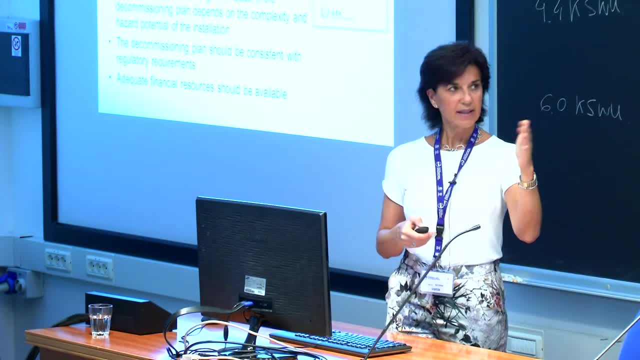 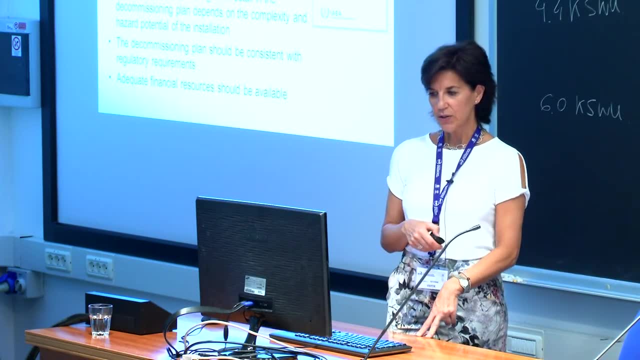 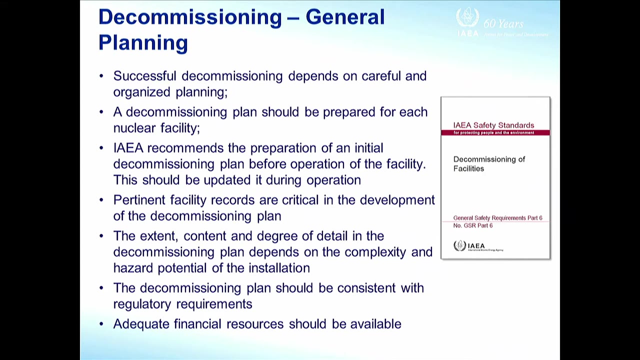 of the facility are made should be kept as a record and facilitate the decommissioning tasks. And also the agency recommends, when a nuclear power plant is shut down, to start the operation taking the spent fuel first to store on site or away from the reactor, but starting discharging the spent fuel from the core. 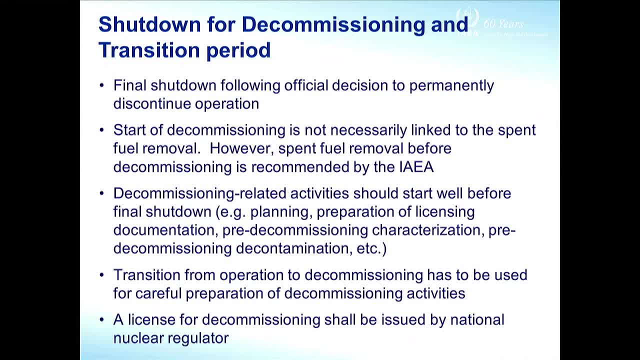 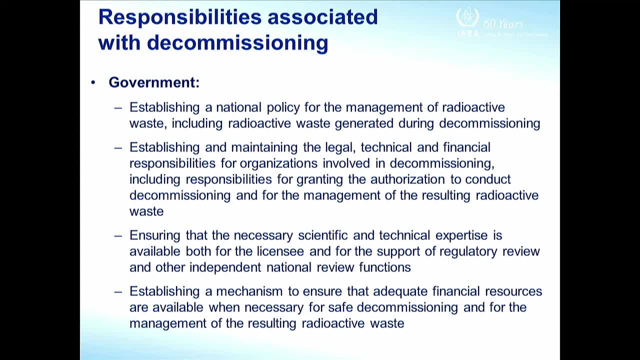 from the first part, So the responsibilities associated with decommissioning. we have three main bodies: The government, the regulatory body and the licensing. So the government: the responsibility is to establish a national policy for the management of the radioactive waste And also the waste generated during the decommissioning. 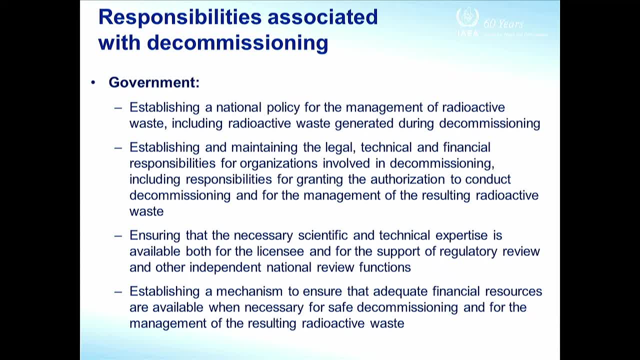 The government is responsible to establish and to maintain the legal so with the regulatory body and the technical and the financial responsibilities for organizations involved in the decommissioning. So the government is responsible to be sure that there will be funds available at the time of the decommissioning. 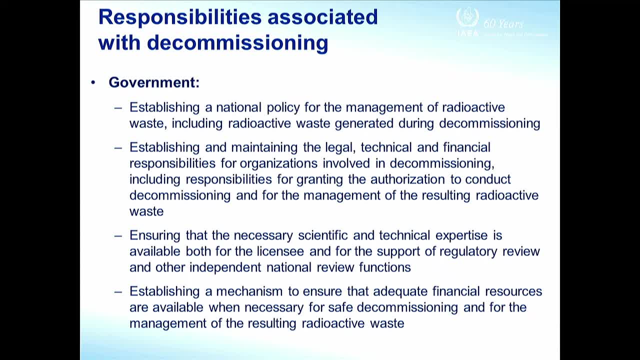 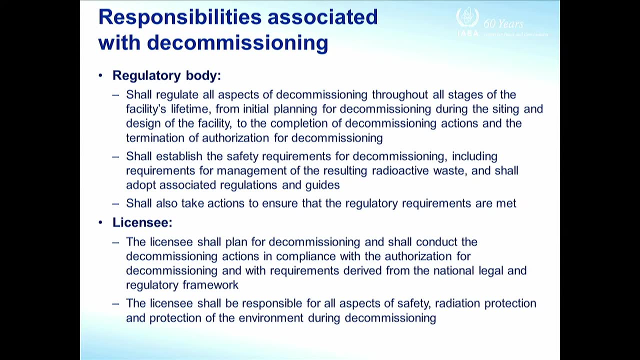 of the nuclear power plants And also they are responsible to ensure that there are the necessary scientific and technical expertise in the country to do the decommissioning activities. The regulatory body shall regulate all aspects of the decommissioning throughout all stages of the facility's lifetime. 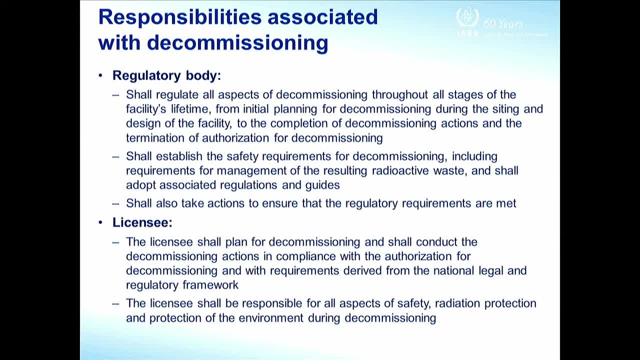 from the initial planning and during the decommissioning. So it's the responsibility to issue the license for all operations and also the license for decommissioning, And the licensing shall plan for decommissioning and shall conduct the decommissioning actions in compliance with the authorization. 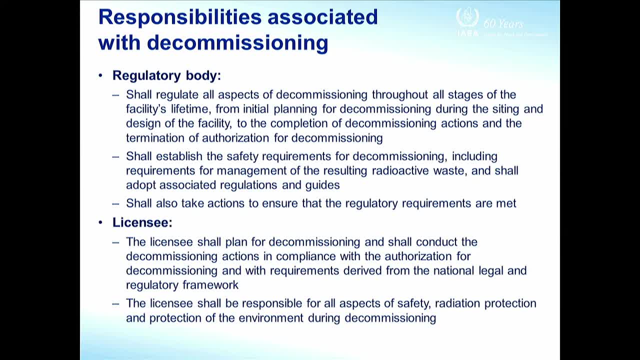 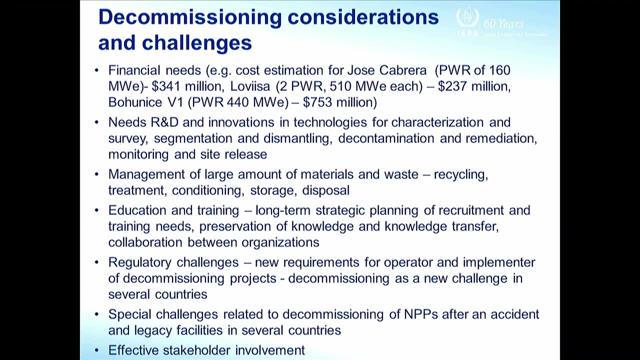 of the decommissioning issue by the regulatory body And is responsible for all aspects of safety, radiation protection for the workers and for the environment. So what are the decommissioning challenges? So the first one is the financial needs. So, as you can see, I put some figures. 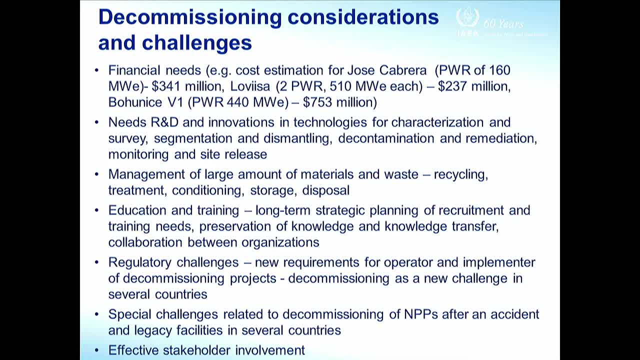 of the cost of decommissioning of different plants: In Spain- it's very small plant- and also in Finland and in Slovak, And this is the forcing cost. So there is also a need for research and development and innovations in technologies for characterization and survey. 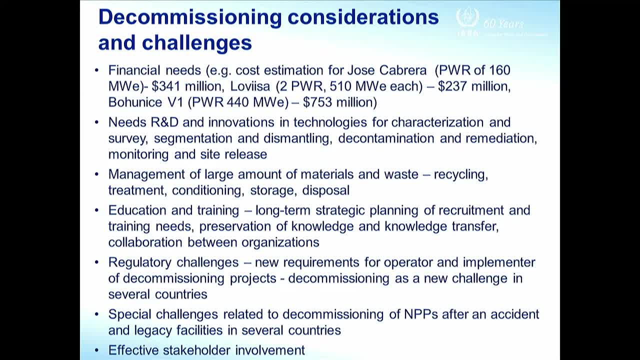 for segmentation and dismantling and the contamination and remediation of the environment, And so, since there are different types of facilities to be dismantled, the agency is organizing discussion groups to share information and to put in common all the developments that different countries are getting. 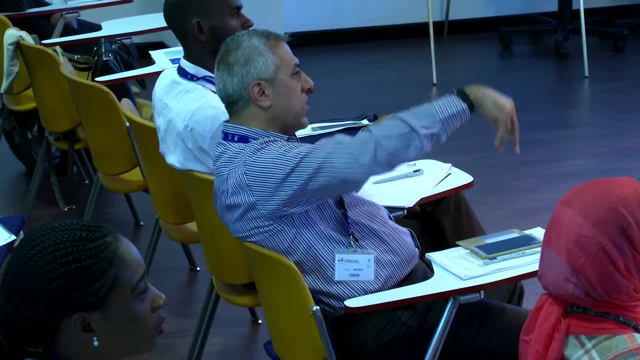 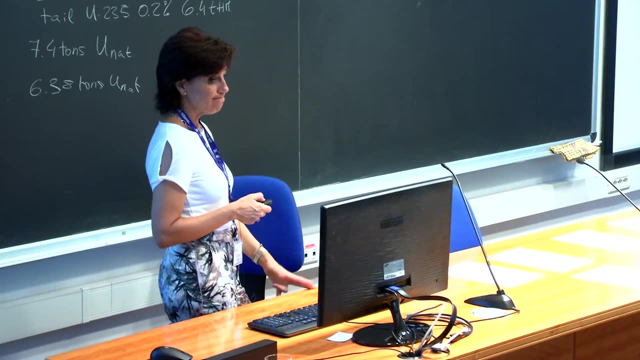 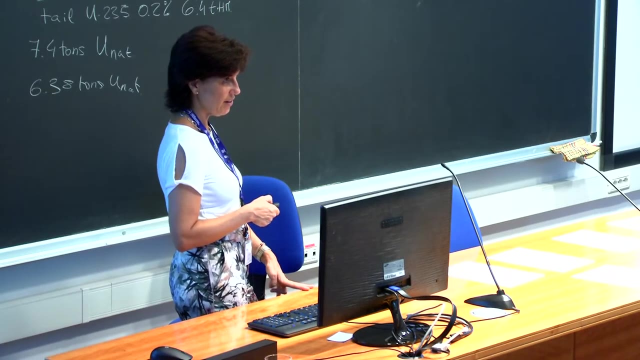 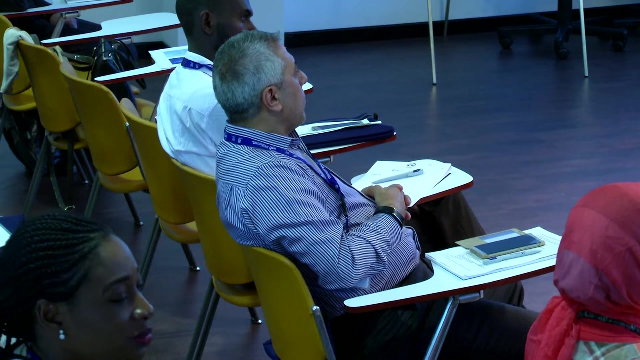 Thank you. Is there a country estimation for the cost? I don't know what they consider, the figures they consider or the implications in the country, Because the is in Finland and they have the disposal facility available and I don't know. I don't have. 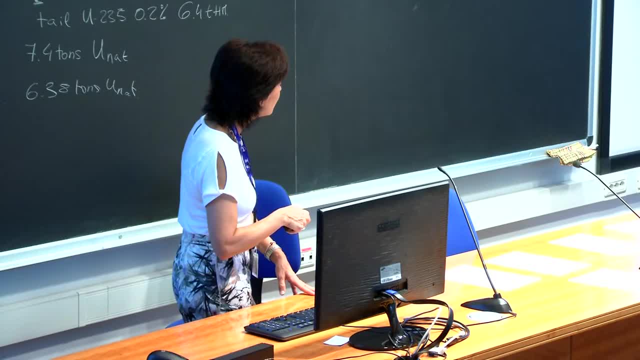 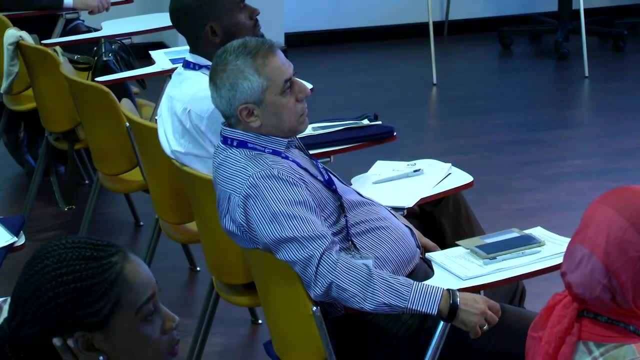 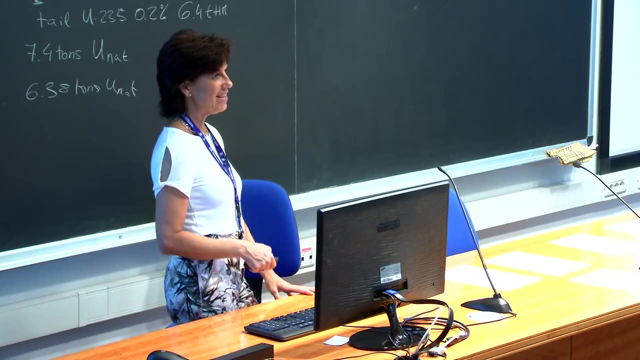 all the considerations they consider when they calculate the cost. This is the calculated cost by every country, But it's to give an idea that it's about 100 millions of dollars, 100 millions of euros, And I guess that this is the initial calculation. 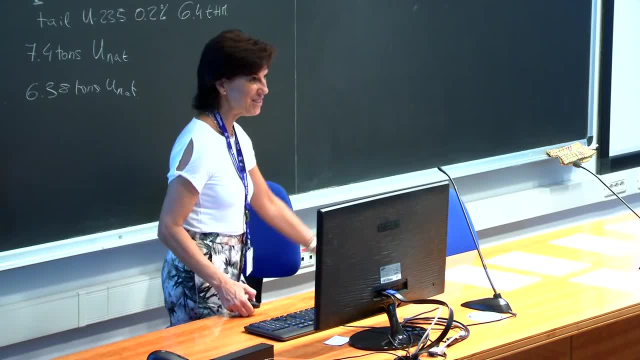 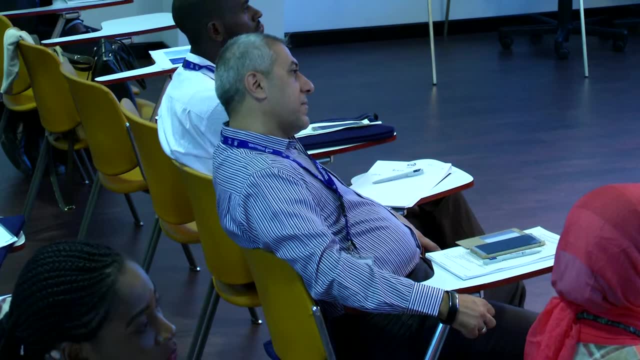 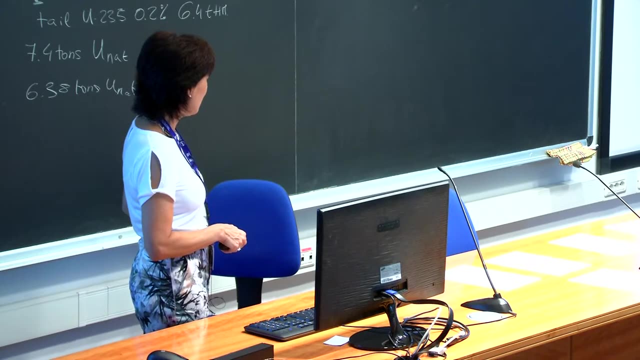 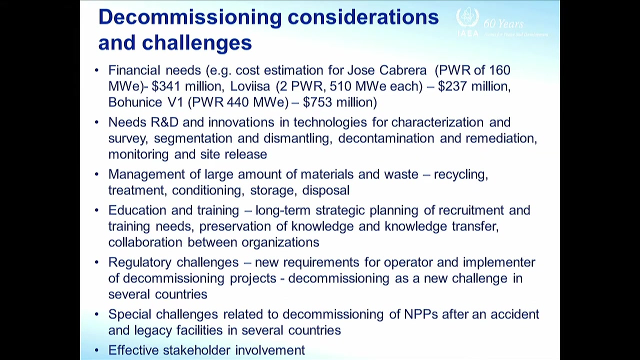 and the final calculation is completely different And the final cost will be completely different. So this is the estimation cost, depending on what is considered. So, but at the end we finalized with the same as during the nuclear, the spent fuel and radioactive waste management. 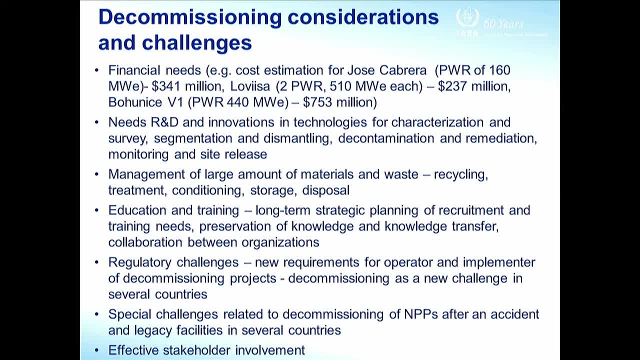 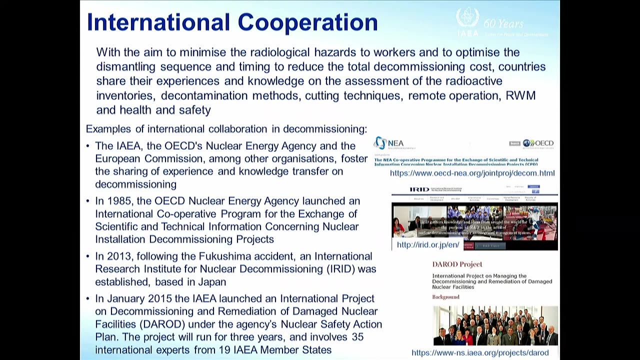 So it's necessary to have effective stakeholder involvement also in decommissioning and environmental remediation activities, because there's a huge amount of waste managed during these activities. So- and this is very important, because there is a lot of international cooperation and collaboration in this field- 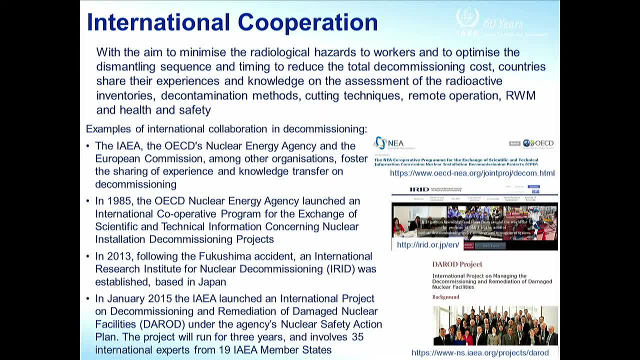 So, as an example, the INC, the OECD, NEA and the European Commission are working together And, for example, the OECD launched in 1985 a program dedicated to a change: scientific and technical information, And they are still working in this project. So the phase will start. 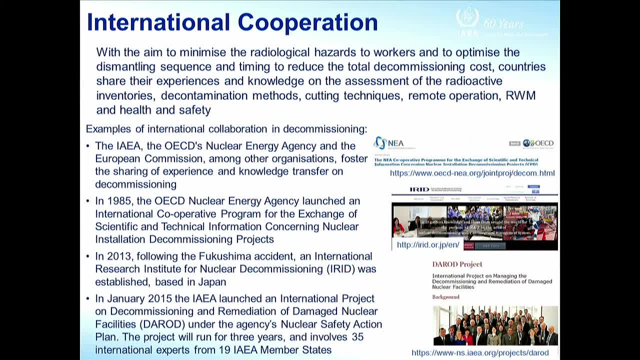 in 2014 until 2018, the last phase of this project And after Fukushima accident. in 2013,, Japan established the IBRIT project and it's an international research institute for nuclear decommissioning, And in January, the INC, also after Fukushima accident. 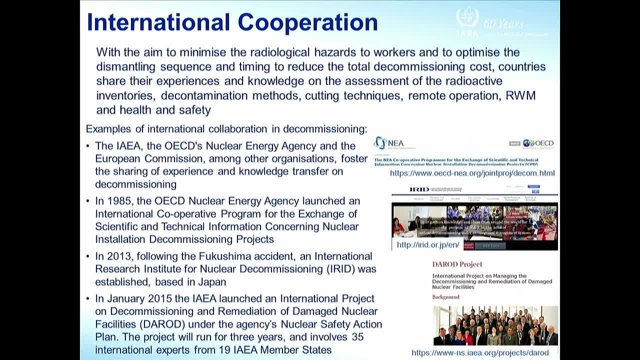 in January 2015 established the DAROT project, as is the project on decommissioning and remediation of damaged nuclear facilities under the INC nuclear safety action plan, And the project gathered 35 international experts from 19 member states, So you can have. 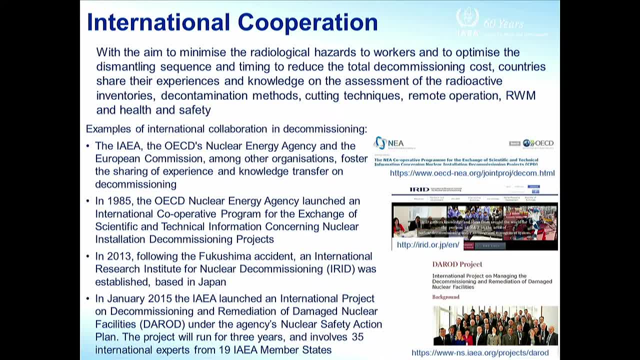 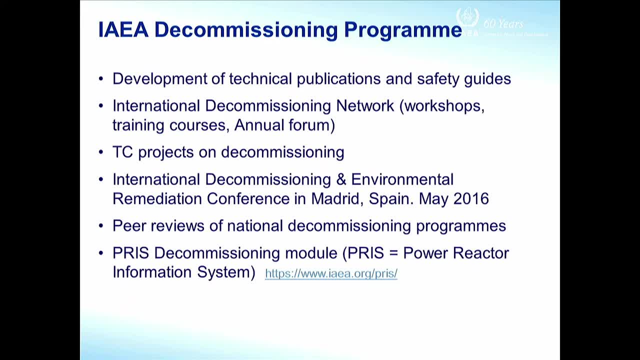 you have here the links of the three webpages where you can find the information of this international collaboration. So what is the INC doing in the decommissioning program? So we are developing technical publication and safety guides. as you see, The network we have an international 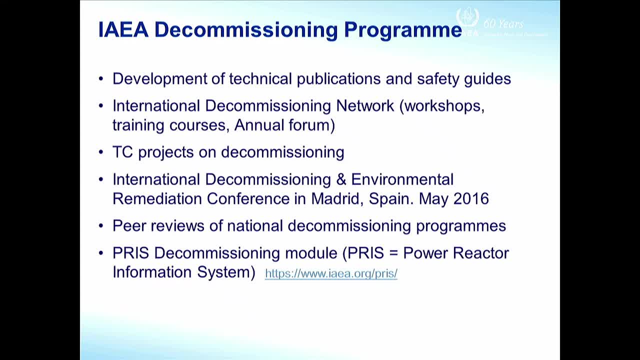 decommissioning network. We collaborate with the technical cooperation department in projects on decommissioning to help member states. We held some conferences and the last one was the international conference in Spain in May 2016.. We also organized peer reviews missions to review. 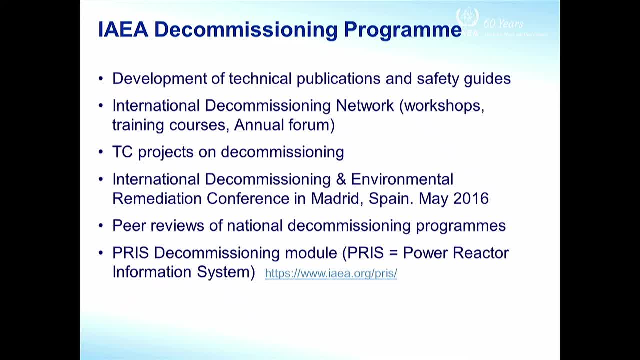 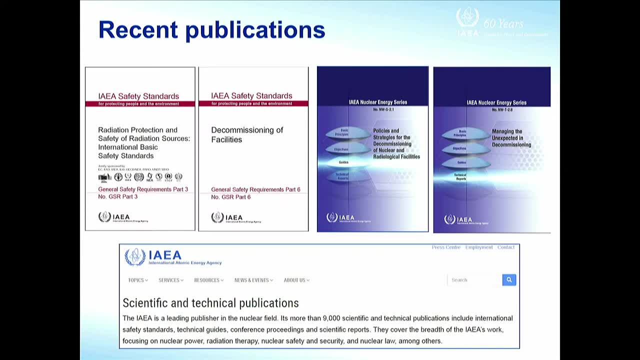 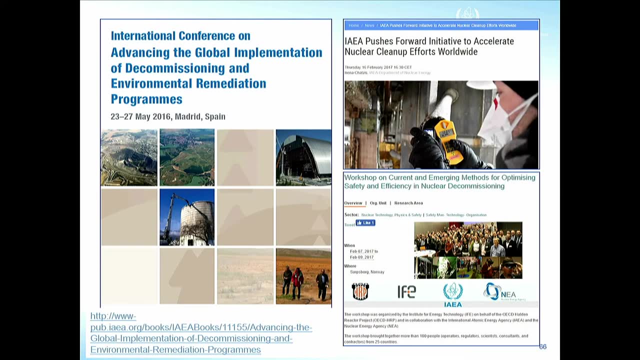 the national decommissioning programs and you can find a lot of information in the decommissioning module in the PRIS information system. So these are some publications and this is the conference in Madrid and this is the link of the proceedings. You can have all the information. 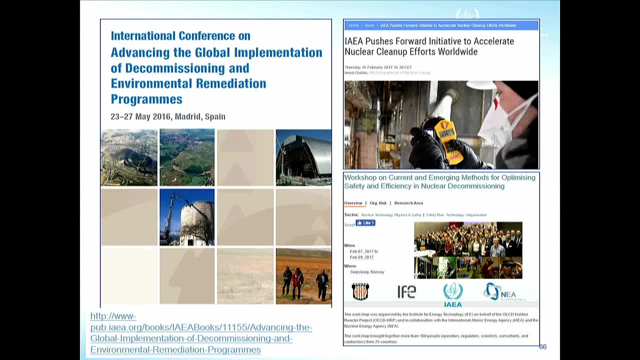 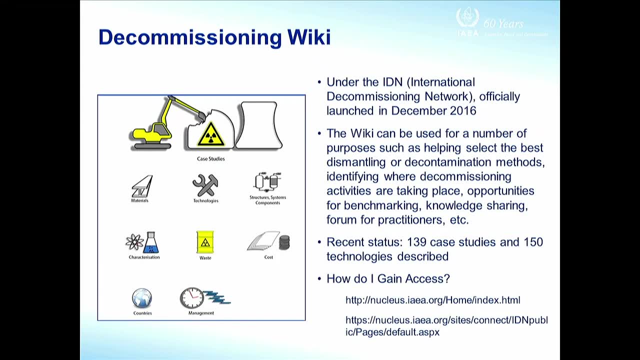 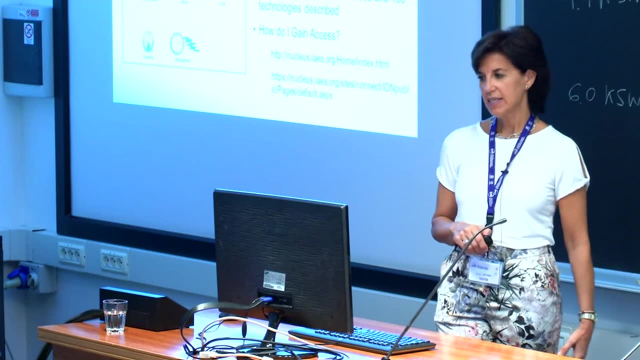 for the conference in this link and some examples of activities related to the commissioning. We have a wiki here under the network on the commissioning, So the wiki can be used for a number of purposes, such as helping to select the best dismantling or decontamination methods.